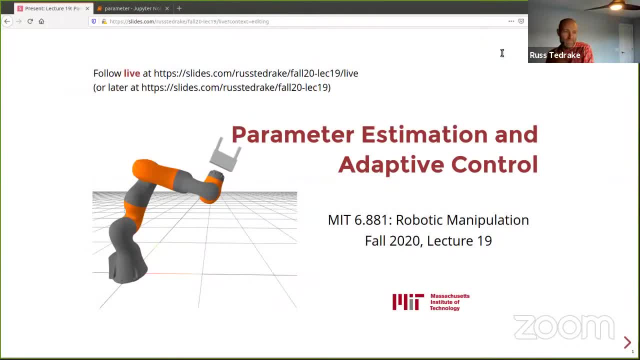 And we're ready. All right, I think I'm ready. I think I've got like the 15 things Good to go. All right, Welcome back everybody And we're ready, So okay. so I had originally planned to go right into control through contact, but I've had some good discussions with people in their projects and the like and 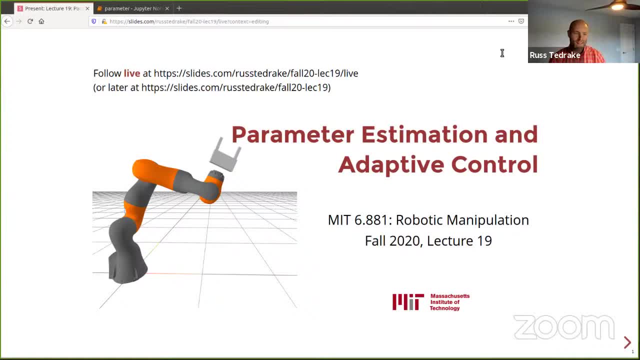 I couldn't help but stick this lecture in. I feel like there's a few things that the field knows that I want to make sure you know about how powerful parameter estimation can be in the context of manipulation like this, and certainly for the robot, maybe even for the things you're picking up, and how that plays into adaptive control. So I'll talk more about estimation than adaptive control. 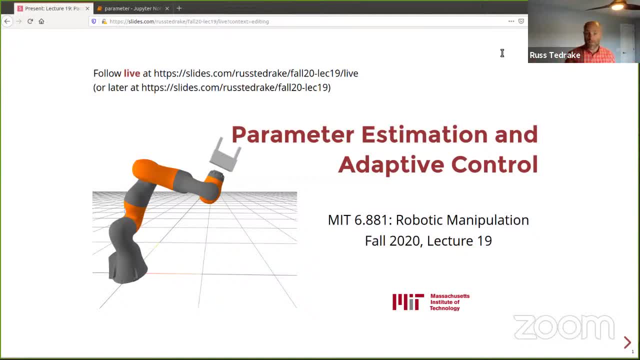 You could take an entire semester on adaptive control. I'm just going to give a teaser, But I thought I'd do it in the context. A few of you, for your projects, are doing things related to tossing right, And I think this tossing bot project captured a lot of imaginations. This is: 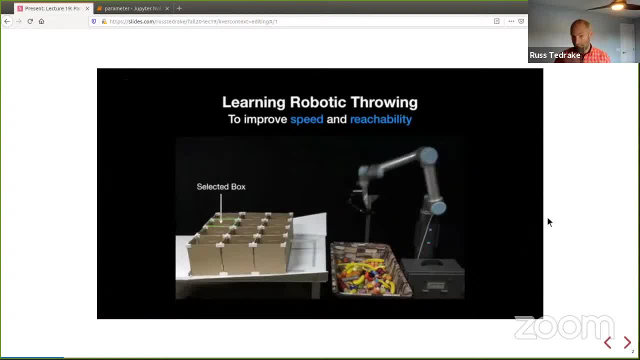 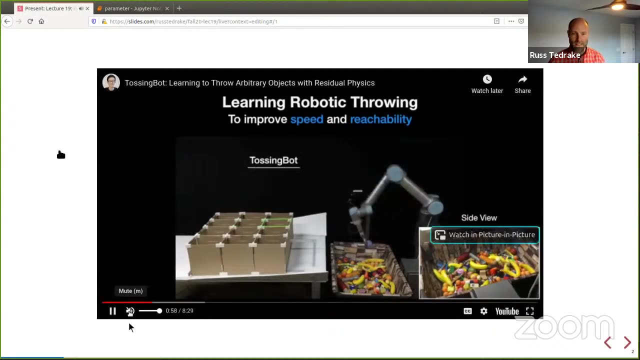 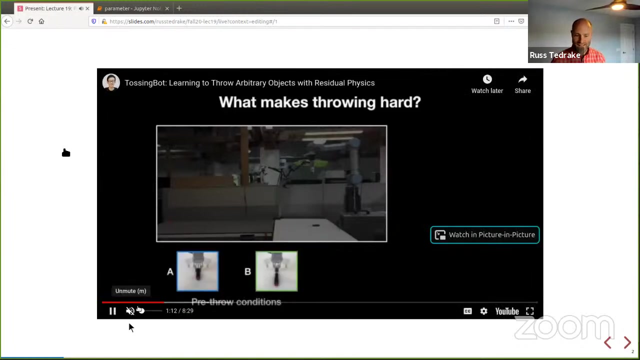 you know, I'm not sure if the audio is playing for you or not, but roughly, Andy and company made this robot: throw objects into bins. Actually, I think I will let the audio play here. See how The audio got me Okay. so I will leave my audio off and let people's audio play, I guess. 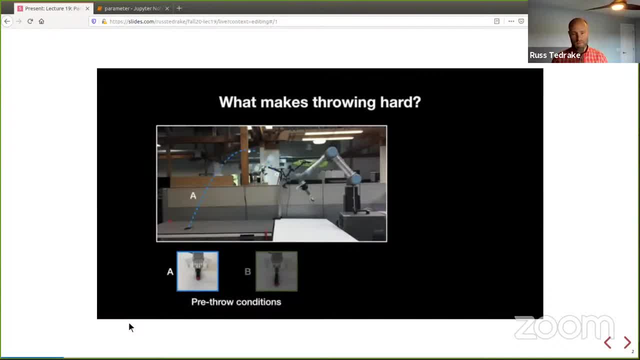 But there's. I want to. I want to let this play for a minute. There's a couple of good, really good points being made here. So, first of all, the pre throw conditions says: if you pick up the screwdriver at a different point, it'll take a very different trajectory. 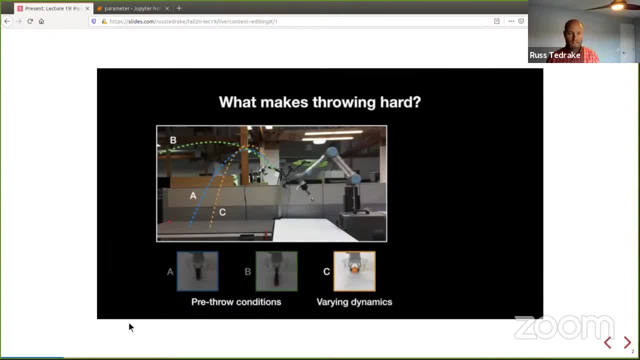 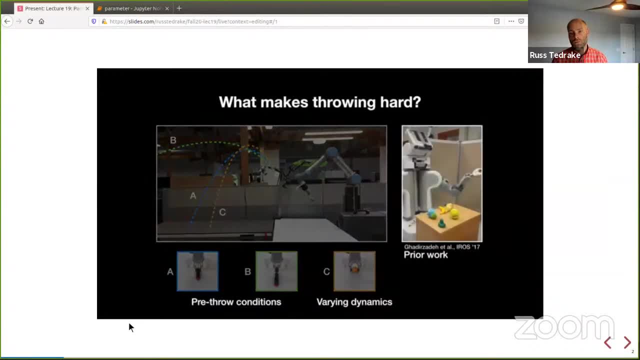 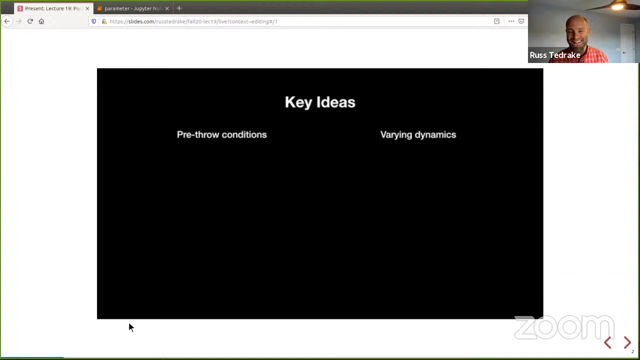 Now we throw a ping pong ball, aerodynamics maybe come into play So you get a different trajectory out. I want to read the paper about darts. I haven't seen that one. Okay, I just want to get To a key part here. 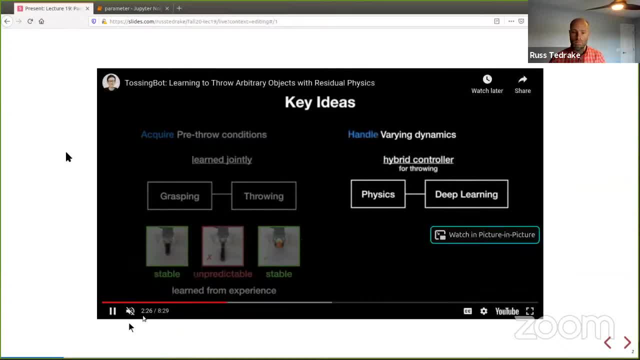 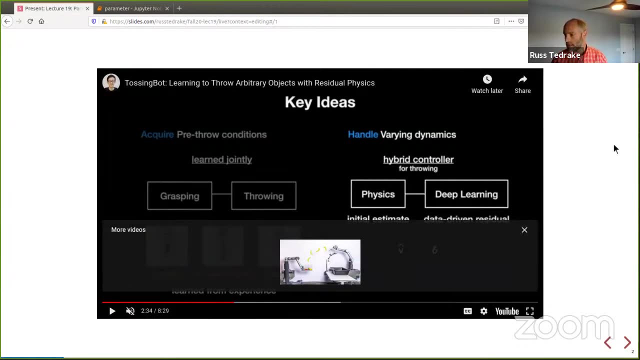 And let me see if I can get a drag. Okay. so I think one of the big ideas in the paper, I guess, was this idea of combining physics with deep learning in order to throw. so you have the basic physics based understanding of, Maybe, where the ball would go if it was just projectile motion. 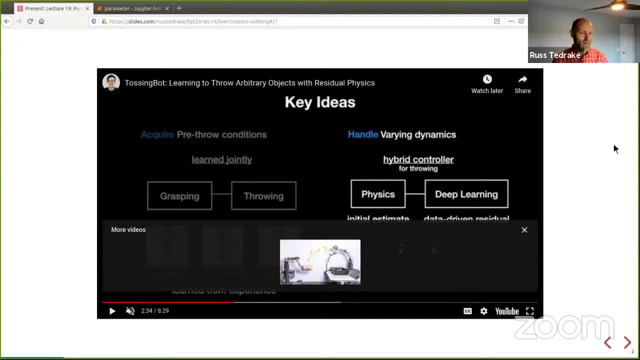 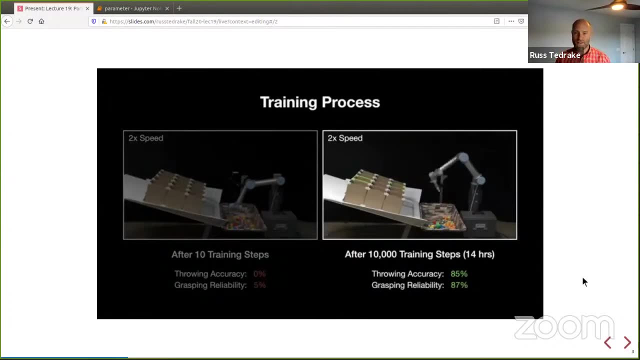 But then you can learn to throw bananas and ping pong balls and screwdrivers with a residual model. And one of the best things about it- if I go to the next slide here, I think my favorite part of the work- is actually the way it so it's throwing. you know the way it trains: it throws into a bunch of different bins. 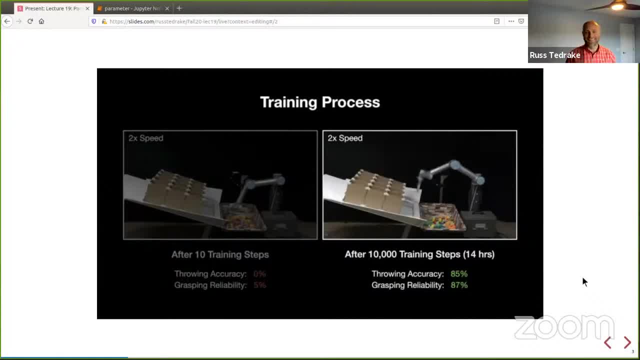 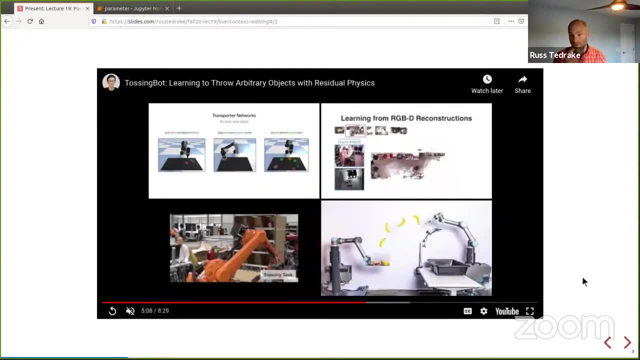 And then super good to just automatically reset and then keep throwing. That's like that's the best part, Okay, so I think that was. that's a cool recent paper that I think the idea of learning these residual networks is extremely good. 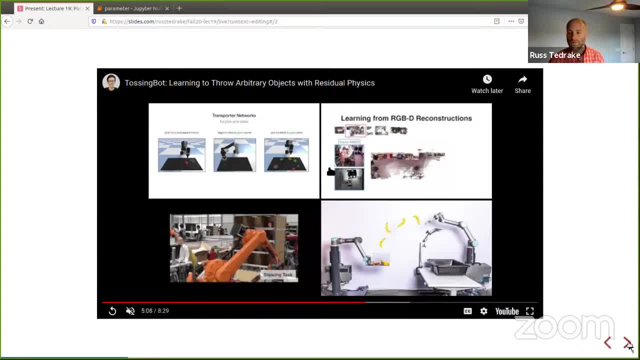 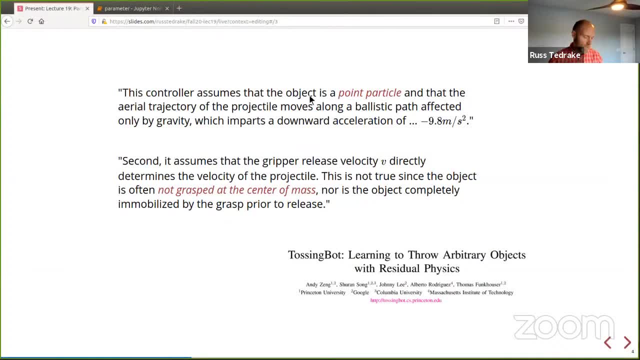 I just want to make sure we understand what we could have done, you know, before that piece of that work. So let's let's look a little bit at the assumptions here and we'll think through a few of the details. You know, the controller assumes that the object, the model based controller. 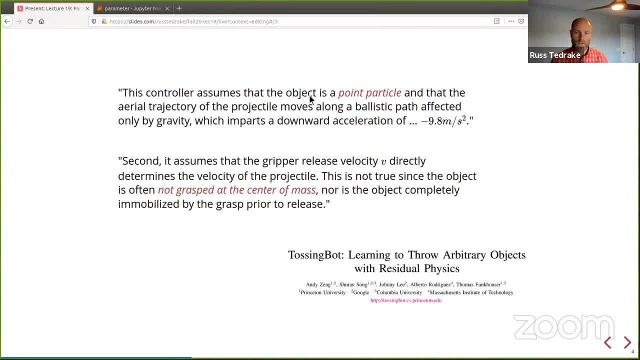 The physics based controller, that object is a point particle and that the aerial trajectory of the projectile moves along a ballistic path. and we'll write some of the equations down in a minute. So that's the basic. you know physics model And they point out, I think correctly in the in the paper- I mean there's even in their description. They say there's two major phenomenon that caused this to not be a good model. 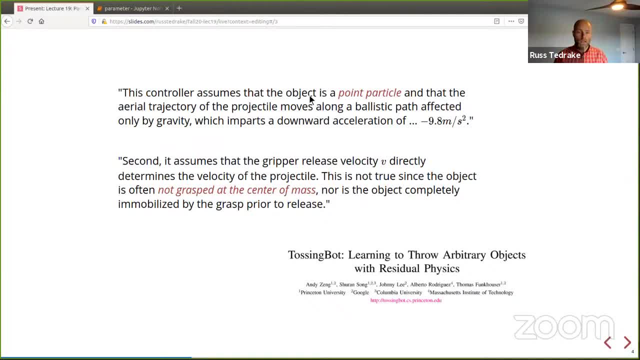 I think one of them is the fact that you're often not grabbing the model, the object At the center of mass. So if you pick up an object and you know it's center masses is far from your grasp And you control the velocity of your, of your hand, when you let go It's really the velocity of the center of mass that matters- And we'll see that in the equations- not the velocity of the of the hand, and that can lead to a very different trajectory. 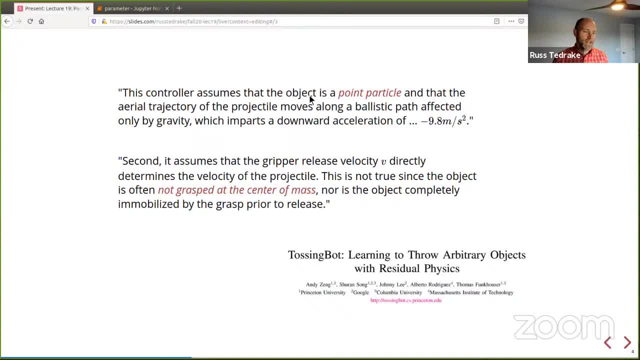 Okay And I have to believe that's kind of the dominant effect, that the dominant thing you'd have to learn The aerodynamics, I think You know, was the second thing they call that, you know, i think the aerodynamic. maybe for the ping pong ball the aerodynamics are significant but I don't think aerodynamics are a major factor in the projectiles that that they're throwing. 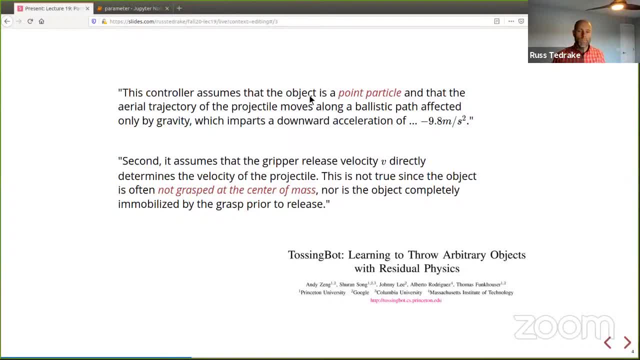 So I want to question you know how well can we estimate the center of mass of the object Before we throw it without any learning, instead of instead of like learning from pixels and and everything, picking up the grass? What if I had to estimate? 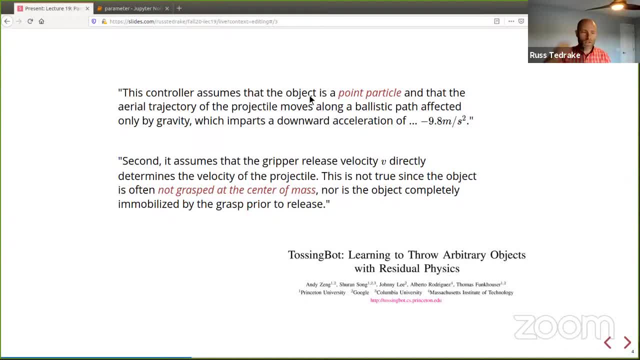 if we just pick up an object, move it around a little bit, use our torque sensors to estimate the center of mass of that object and then do a more accurate growth, How well would that work? And that's what I want to sort of talk through today. This is a 1991-ish video. 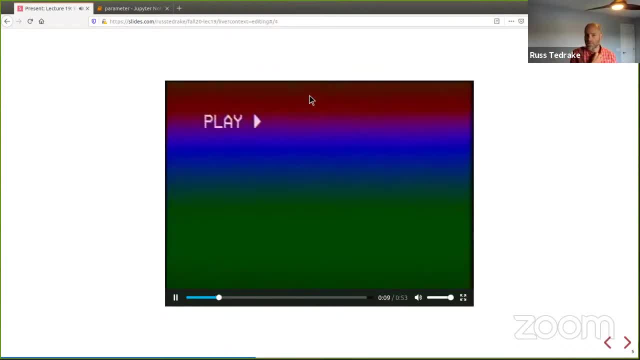 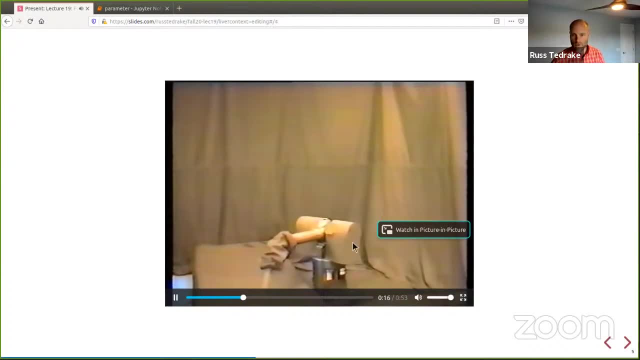 from Jean-Jacques Slotin. It was actually. the paper was never published, but this was an adaptive controller which would pick up a mass. I'm going to mute my thing again there. pick up a ball of unknown mass, go like this to estimate its parameters, and then you know. 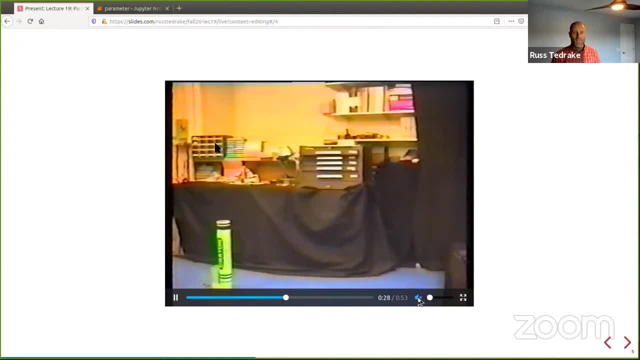 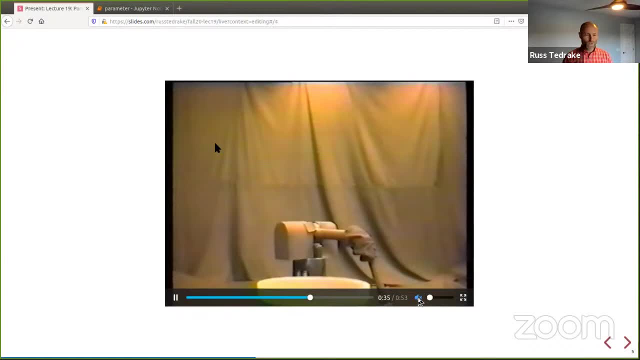 throw it into a hoop across the room. really well, I think. So this is so. now you're looking down the, you know, down the chute of the, of the hoop That was just to get it to a known position in the hand and then slunk, you know, slam-dunk. 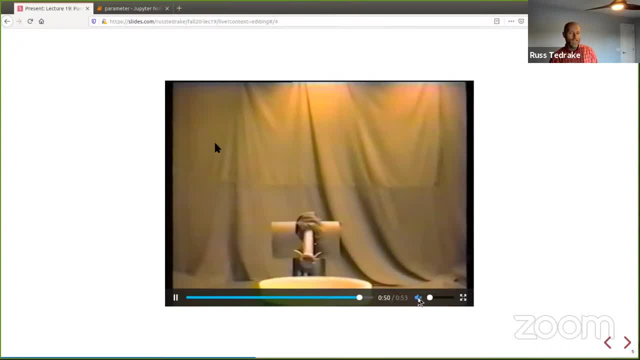 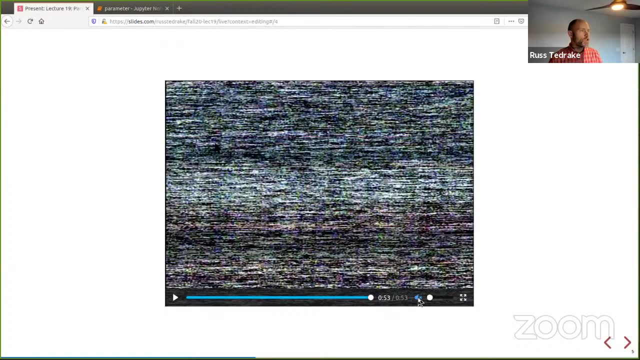 everything time. So there are some very, very powerful ideas there of, just you know, parameter estimation and adaptive control, and I think the newer work on learning and learning residuals can improve on that in important ways. but I want you to understand that there's some things where 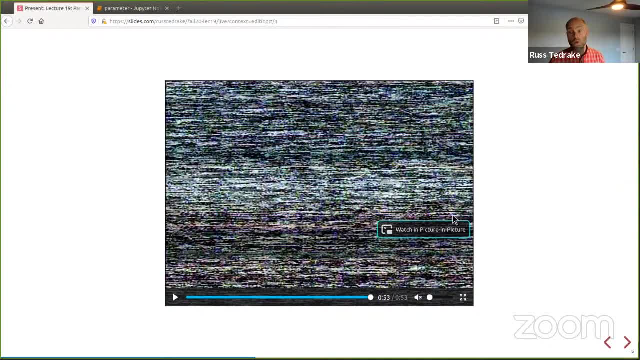 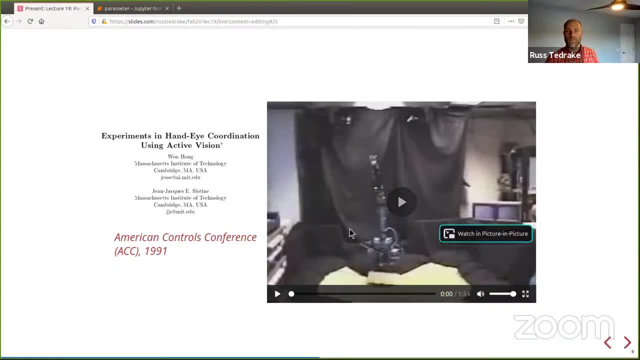 we have almost closed-form solutions for that go a pretty long way. This is actually a series. there was a series series of papers that were sort of around that time from John Jock's lab. By the way, that arm is the WAM- the Barrett-WAM arm It was. 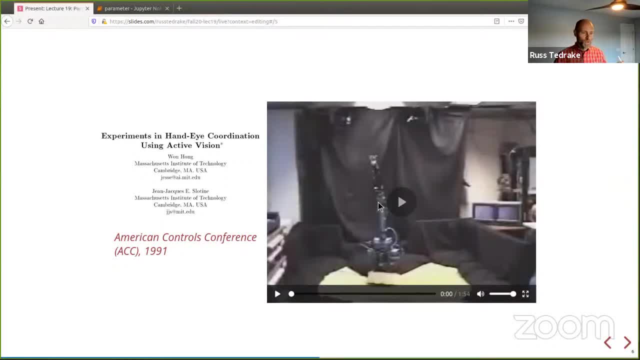 this was actually like, I think, Barrett-WAM number two or something like this, you know, and because Bill Townsend is in town and was in the lab for a while and they were building this, This was also the time when Ken Salisbury was here building incredible hands. 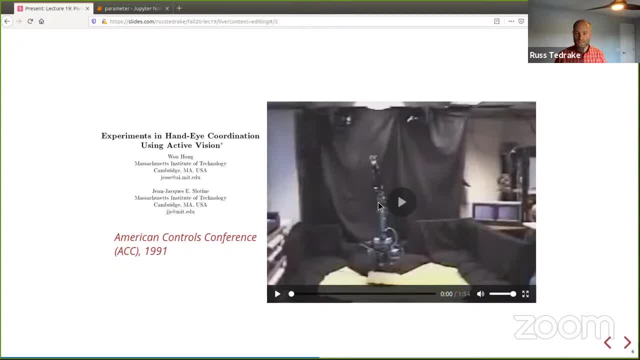 including the MIT-Utah hand. Actually, I'm going to have to show you when we get to the Dexterous Hand stuff. but so they also. they did a bunch of really clever things. They didn't have computer vision the way we do now back then. So what they did is they would they had foveating cameras. 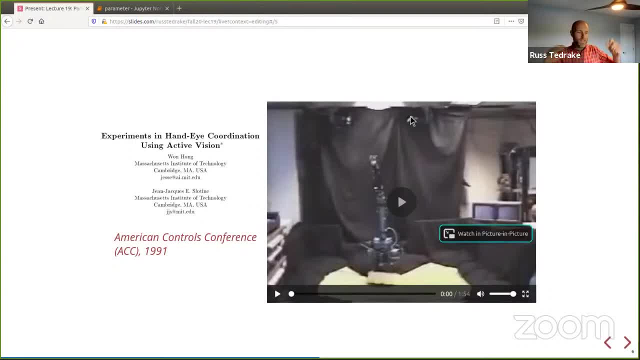 right. So there's two cameras at the top here, if you watch them carefully, and the scene is such that there's like a bright white ball, a bright orange ball or something like this, and all the vision system knew how to do was keep the bright white or orange ball in the center of the camera. 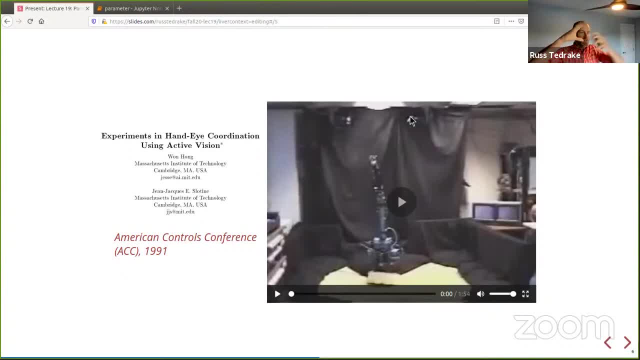 And then it's very easy to track the center of the bright white ball and then use the encoders on the camera to track the ball. So that's what you did like before. we had deep vision, But this was a series of projects where they would also do catching right. 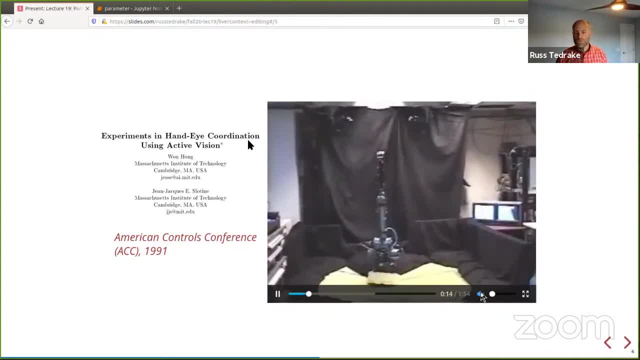 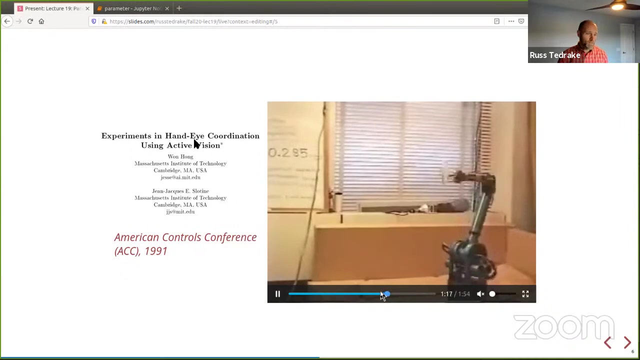 And they'd throw it back And we'll talk about the type of models that they learned and estimated with least squares, But they were pretty rich. Certainly they could learn the parameters of the ball and the robot. But if you look, if you fast forward, you'll see that they're also learning to catch paper airplanes which have significant aerodynamics. I would say. 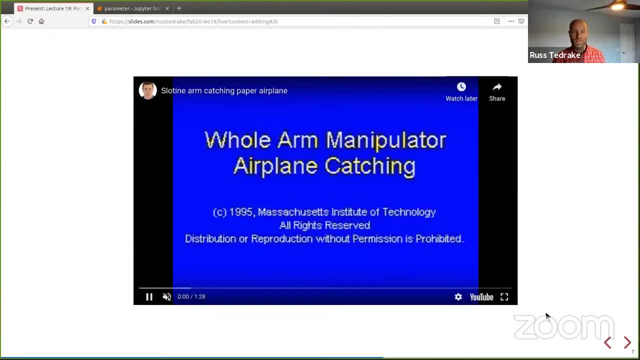 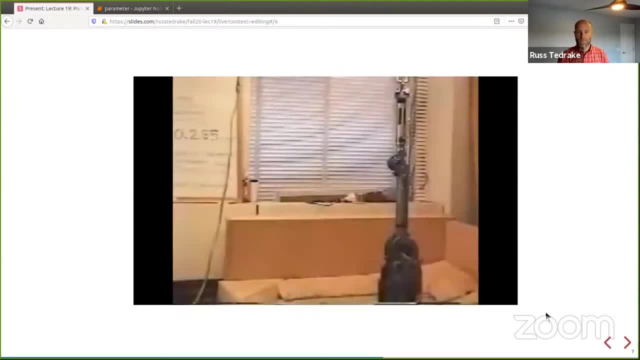 And there's a second video here of, actually explicitly focused on catching the ball- And they used- you know you could think of it as a linear network or, you know, a linear function approximator based on nonlinear features- to learn the aerodynamic terms that they didn't have from their first principle models and they'd grab an airplane out of the air. 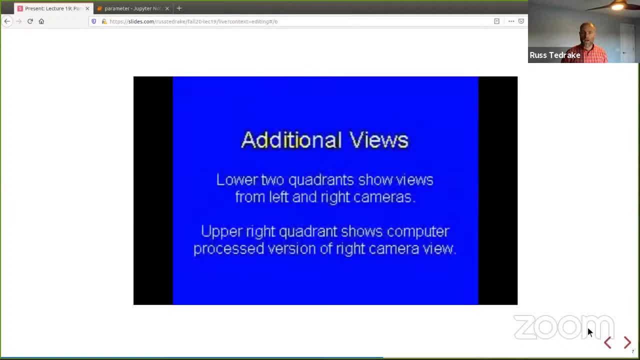 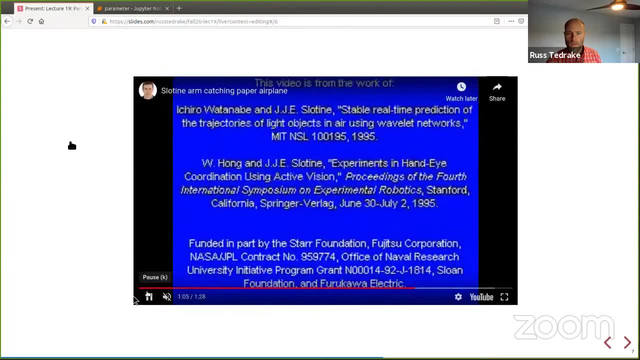 Okay. so I want to sort of talk through some of that And if you were to fast forward somewhere along here. there's a nice, There's a nice, There's a nice. Yeah, right there. Stable real time prediction of the trajectories of light objects in the air using wavelet networks. 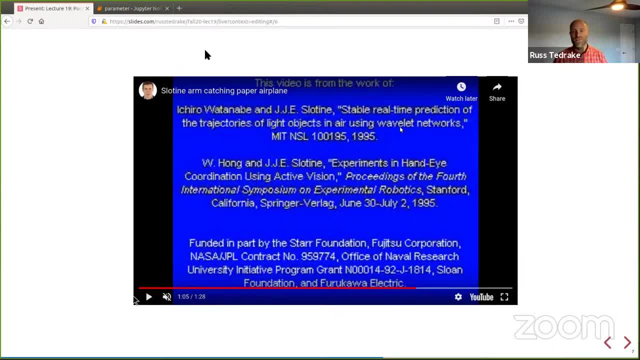 Right, It's like what, how does all this stuff work together? like, what does that do and how does that compete with a deep network? I don't know, but this went farther, I think, than people remember today. Okay, so Okay. 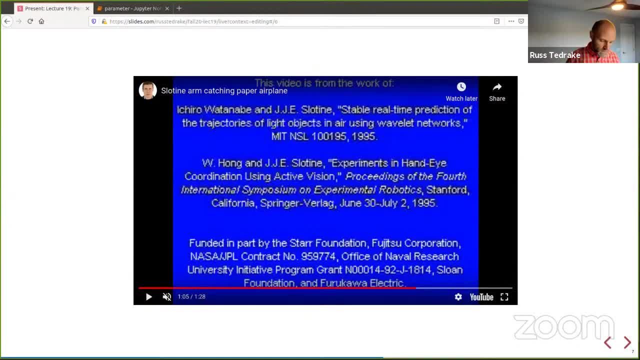 Let's think about parameter estimation and throwing random objects, bananas. Okay, so the first thing I think to think about is the ballistic trajectory of of an object, of an inertial object here of a rigid object. So one of the things that I guess, I guess you know, but you have to remember- is that- and actually Andrea and I were talking about the other day- she's been doing catching for a project and I said: Are you estimating the mass? and then I realized you can't estimate the mass of a flying ball. that you know. 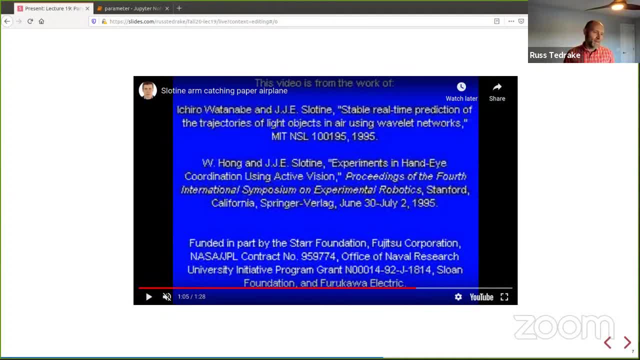 you just have to. If you're watching a ball through the air, there's no way to tell if it's a 10 pound ball or a five pound ball, right, because the equations of motion are just in the air. You know they are. MX. double dot equals zero. 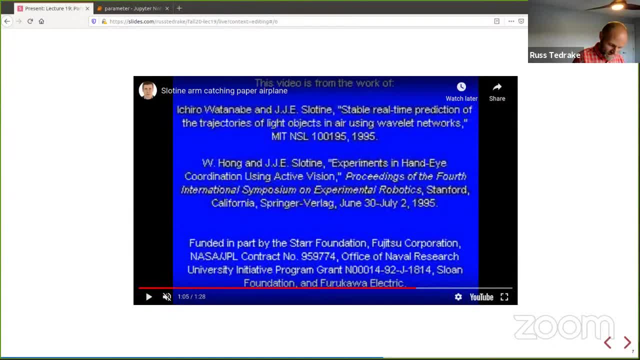 Right, Which implies that X double dot equals zero mass, does not affect the trajectory of the ball at all, And MZ double dot equals negative MG Right. So Z double dot equals negative MG Mass, has no effect on the. I see that I. 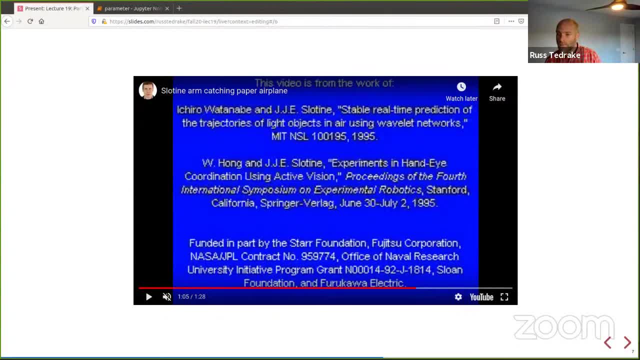 missed my window a little bit again. I'll remember to write low Mass has no effect on the center of mass of the ball Right, But so let's be careful here. the X and Z here. I just said I was going to miss top and then I wrote on the top three. I think we're still seeing the slice calm. 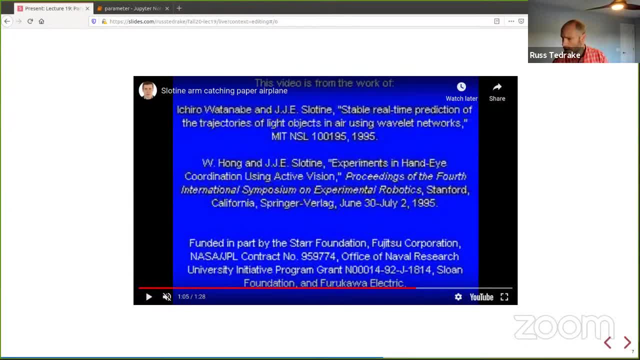 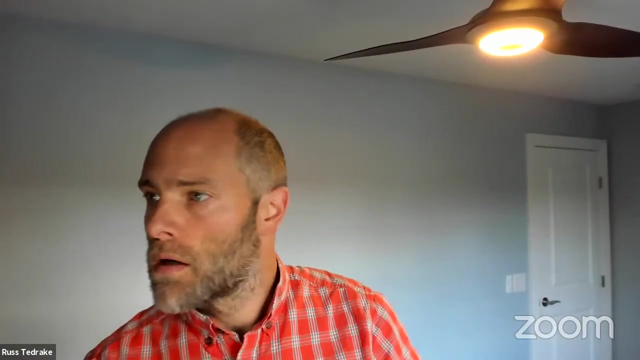 Really, Oh, yeah, Yeah, That's weird. Give me a second to figure that out. Okay, Okay, Okay, Okay, Okay, Let me Gilbert Just gonna restart mind sharing. Okay, Oh, you know, Okay, Yeah. 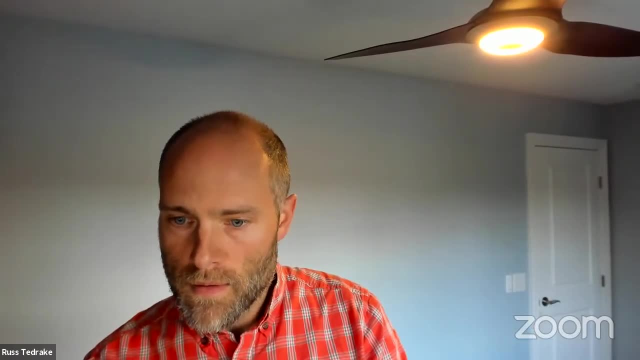 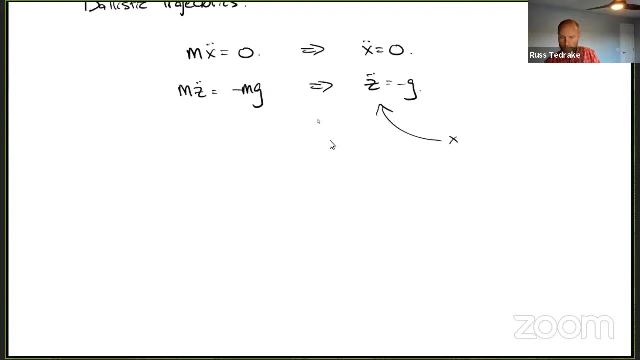 Yeah, hopefully that works better now. let me just test if I can flip back and forth. that's working right. yeah, I don't know why that didn't work for a minute, but let's hope it's better now. okay, so the ballistic trajectory which I will 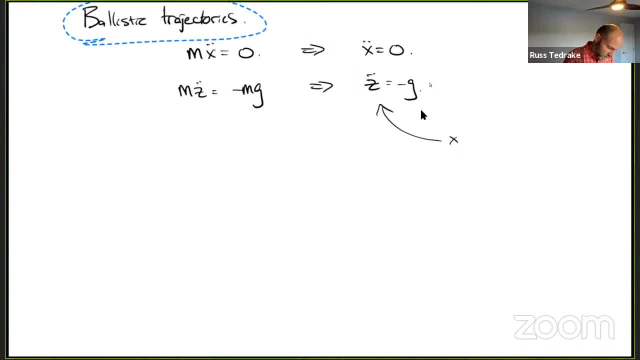 now you don't even know why I was talking about it being too high. okay, the ballistic trajectories are mx. double dot equals zero. these are the equations of motion of where x and z are the location of the center of mass right, not some arbitrary um before most of us was born. thanks, um, not some arbitrary point on. 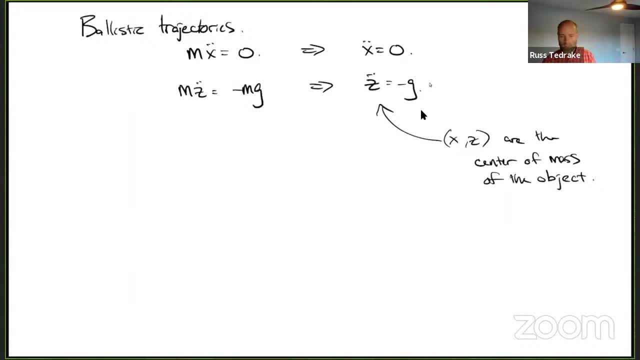 the body that you've chosen as your zero, zero, zero in your SDF file, but it has to be the center of mass. it's the center of mass that goes through that completely ballistic trajectory. so similarly, you can ask about the rotations. maybe you want to flip a bottle and have it land on the. 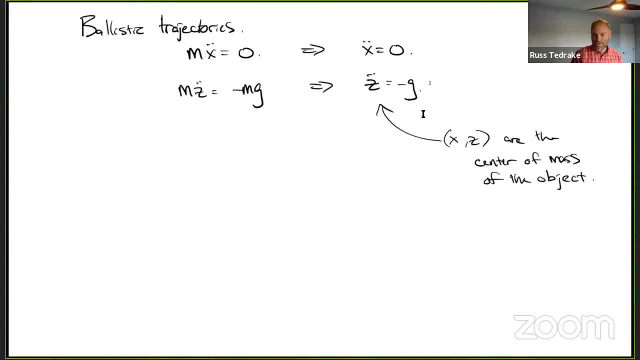 land on its, um you know, upright, or you want to, I don't know. the banana has to get in a certain orientation when it lands. so um the again. we have conservation of angular momentum about the center of mass right. so um i theta. double dot equals zero in the planar case, because there's no moments. 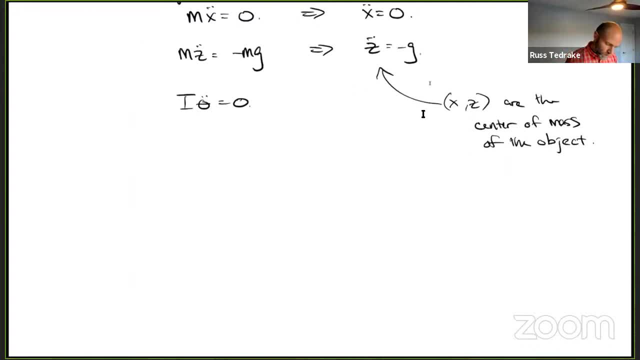 acting directly on the um, on the robot and i, is the moment of inertia about the center of mass. okay, so, um, that also implies that theta double dot equals zero and I just don't need to know the mass and the inertia. but I know when the um ball takes off if I know its center of mass location, or the banana. 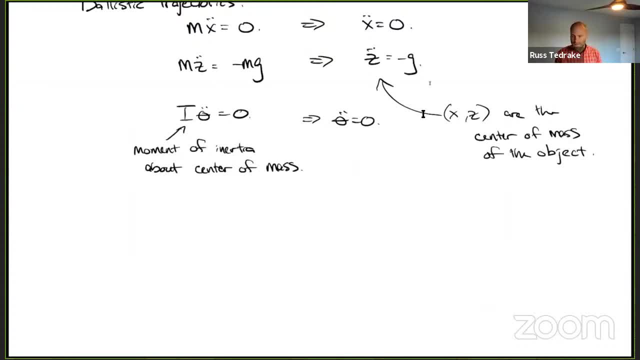 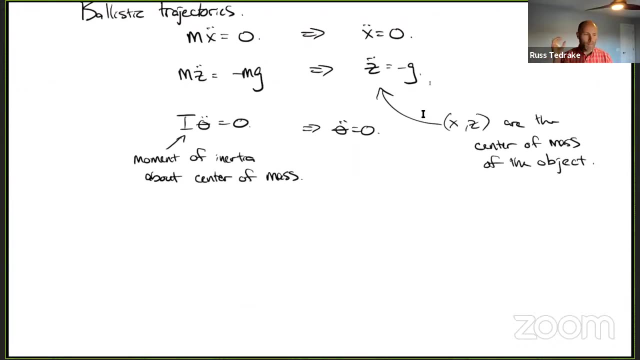 whatever takes off, I know its center of mass, location and velocity and rotational um position and velocity. then I know everything about how it's going to evolve without estimating the mass. okay, so, um, so, do you even need to estimate the parameters of the ball in order to do the tossing? 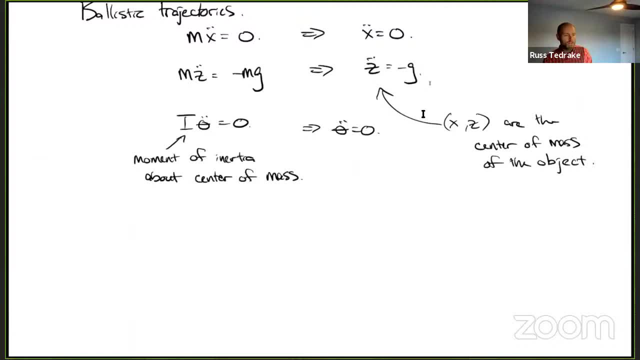 the reason you need it is because your goal is to control the takeoff velocity. so you need to know at least where the center of mass is relative to the hand, so that as you go to take off, the thing that you're regulating should not actually be the center of the gripper. 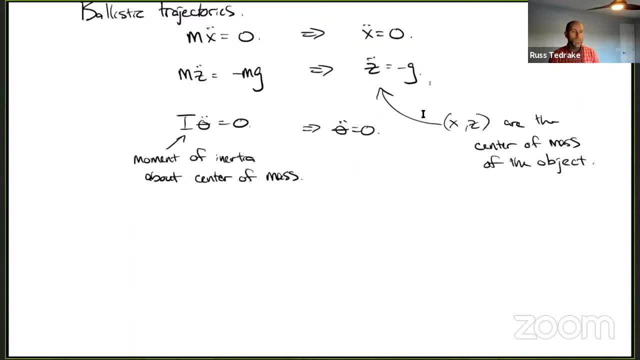 right, it should be the center of mass of the object. okay, so at very least when you shake it around, in fact, the only thing you really need is the center of mass of the of the object and the in the hand coordinates. okay, now it makes sense to actually it turns out to not be harder to. 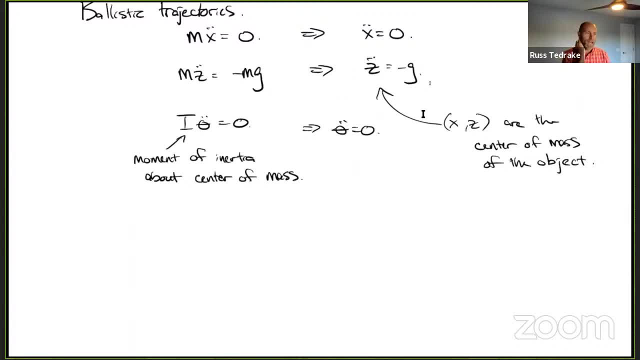 estimate the um inertia matrices at the same time, and you kind of can't- uh, you can't pretend you know them, you'd get the wrong answer. so so we're going to estimate the mass, the center of mass, and the inertia which, which is the entire spatial um inertia of the of the object, uh, all at once. 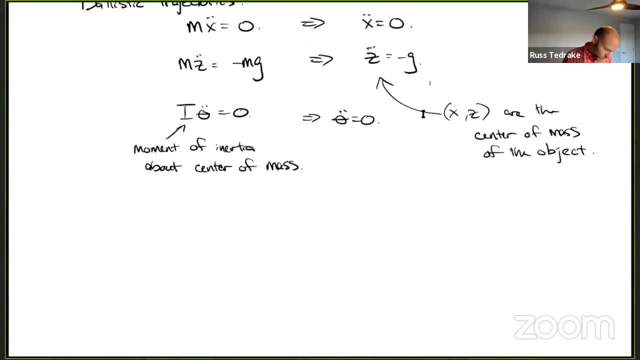 but we really only need the center of mass, right, right, so the trajectory depends on initial velocity of the center of mass. okay, so you might. i guess there is a case where you might need the, the mass and inertia of the object more more completely, and that would be if if it affected the dynamics of your robot in any. 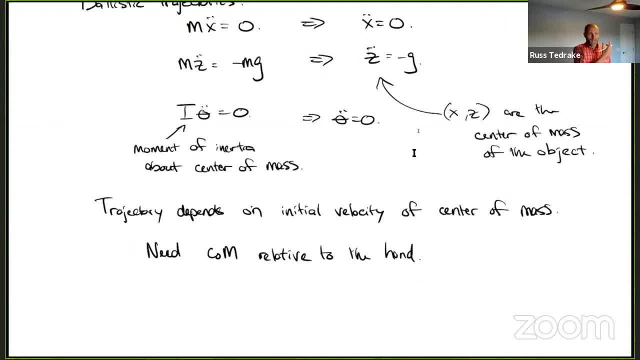 substantial way. if your goal is to build, you know, a robot that is at sort of at the limits of its performance, or or even close, where, like a pd controller, is not good enough, you're going to have to willing, have to take into account the fact that the weight- if you're going to throw milk jugs, for instance, with a, with a wham, then then 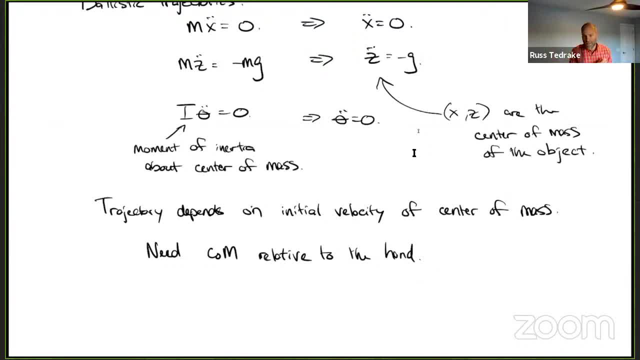 suddenly the, you know, estimating the mass of the milk jug is going to affect the ability of the robot to lead to to open its hand at the right velocity, right so you might need the additional information for tracking, but assuming that the object is light, relative and you can track with. 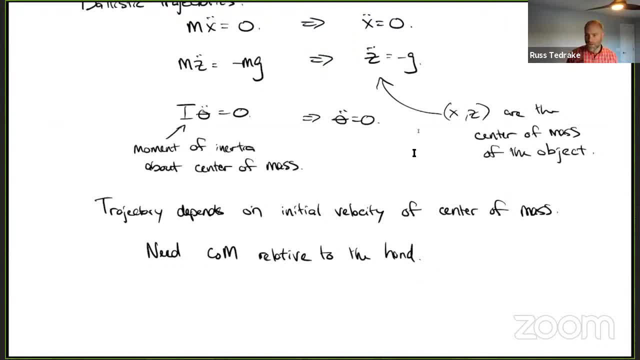 high gain feedback and get to a good takeoff velocity, then it's really only the center of mass that you, that you need, all right. so the thought experiment i want to have here today is is: let's just say we've picked up an object. i'll even for the, for the math, we'll just assume that it's. 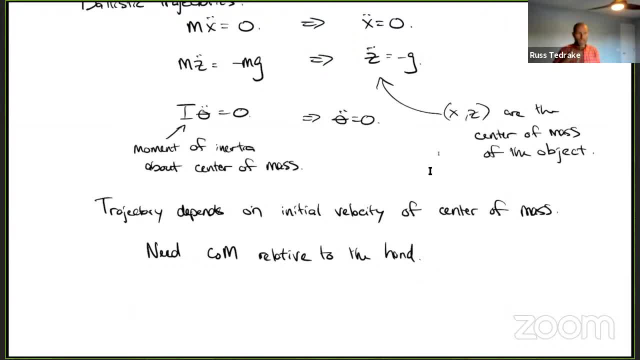 welded to the hand for now. so we won't assume that there's any dynamics of the sliding, although if you can measure this, the, the any movement in the hand, that would be enough. okay, um, but let's assume it's fixed. that just makes my equations easier and we're going to shake the robot, the. 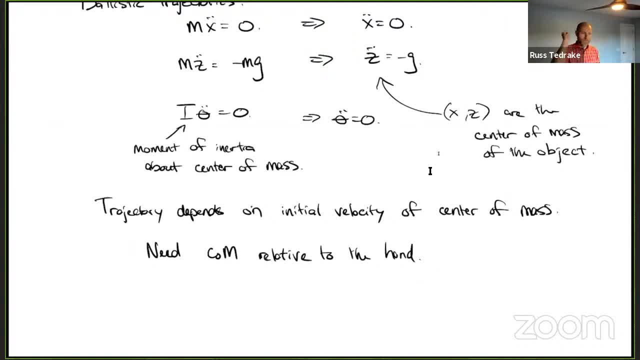 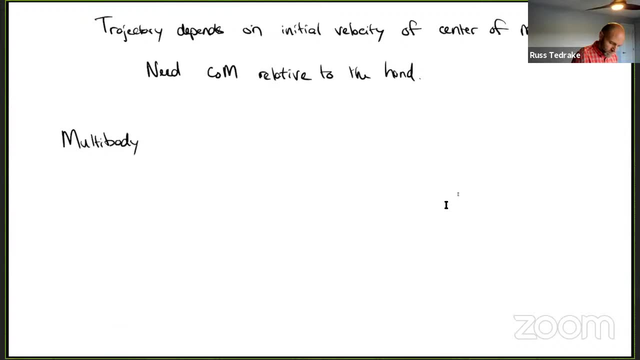 object around, try to estimate its parameters, and then you know, then we can. we can do our throw. so let's dig in a little bit to the structure of multi-body parameter estimation. so, um, if i just think of this as an arbitrary bag of equations that i can learn with a deep 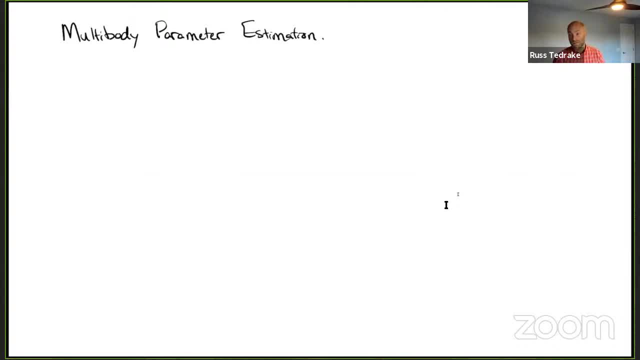 network. i don't doubt that we can learn it with a deep network, but you're, we would be missing out, in fact, in the naive form, um, you would be learning a much harder equation than than you, than you need to learn, uh, and let me try to make that point. so i'll start just with a super simple example. 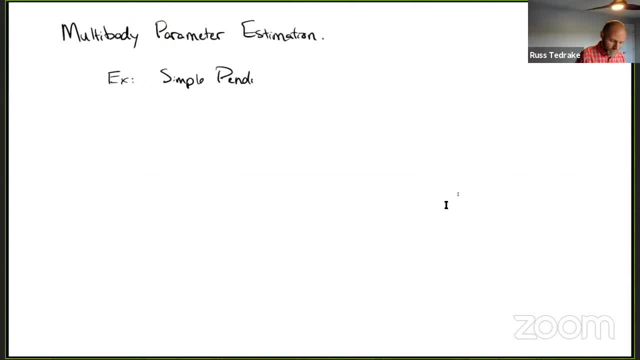 i mean. so the key idea- actually let me just the key idea is that the inverse dynamics- not the forward dynamics, but the inverse dynamics- are actually linear in the parameters, in the lumped parameters, and i'll tell you what that means in a second. okay, in fact, if you take the forward dynamics, if you take your simulator and you try to learn, 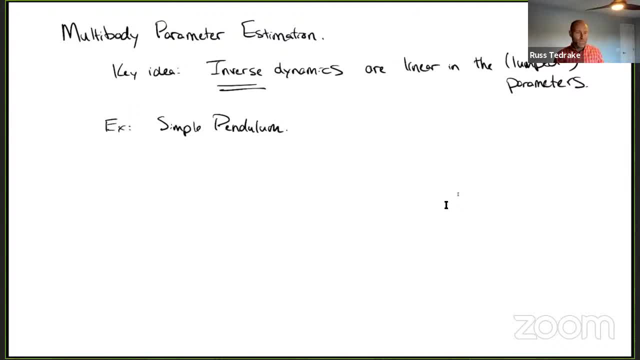 the forward dynamics directly, then it's no longer linear in the parameters and it's a much worse problem to do so. you're actually much better off staying in inverse dynamics form than to use the forward dynamics model, and i can. you can see that even just on a simple pendulum. 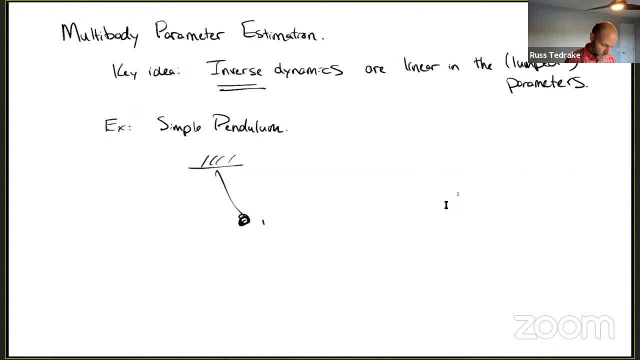 so if you remember my mass length, gravity, theta, equations of motion- i've got some damping here, okay. so let's say we don't know mass length. i mean, okay, if you don't know the length you should just buy a ruler, probably. but but let's say we, um, we have to estimate the, the parameters. 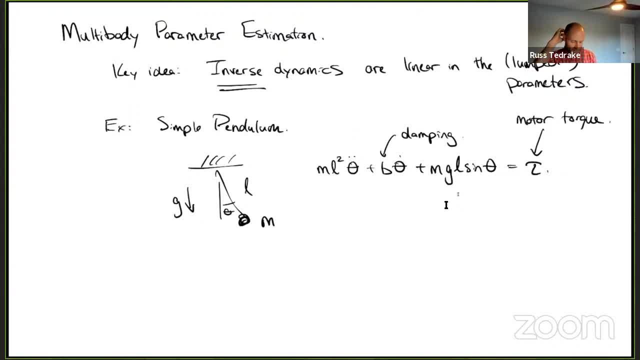 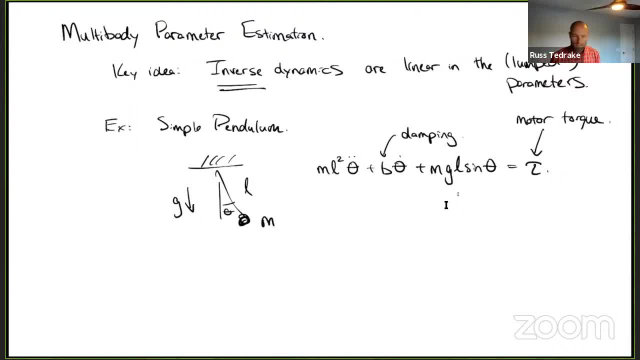 so if we're going to get our data, which in this, in a system identification or parameter estimation, is our thetas, theta dots sine data's, all you know our theta and our and our tiles you know with our parameters. so let me rewrite this says: wow, theta double dot, theta dot sine theta, all my terms that are sort of dependent on the. 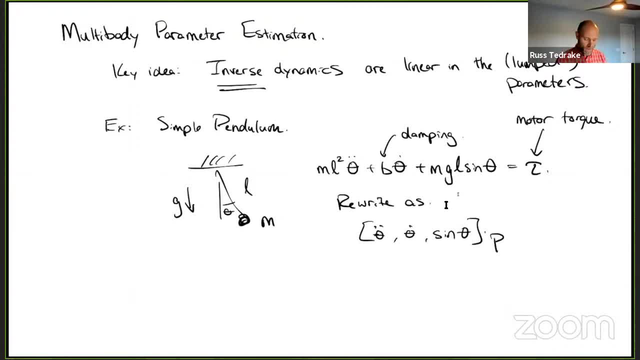 on the data times. some parameter vector B equals tau. Okay, Just simply rewriting the equations, right? Clearly this is a linear set of equations in P, rather, And this when I have data from theta and tau and theta dot, for instance, then this is just a I can. this is just numerical. 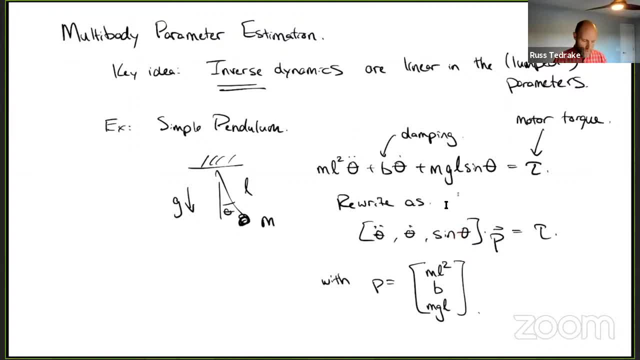 So sine theta is just a constant. also, it's just my data. So this is just a big- gonna be a big- data matrix if I list out a bunch of them. okay, This is just data And the only thing I'm trying to solve for is a vector P. 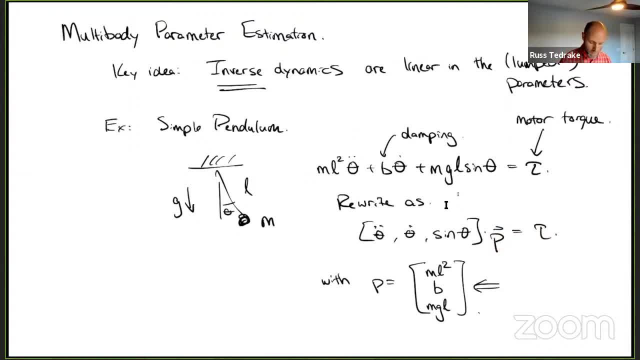 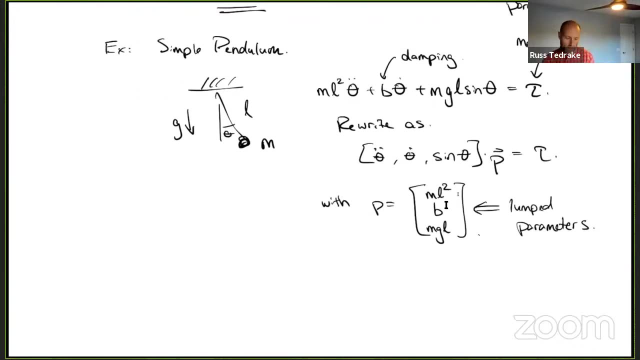 and this vector P. these are the lumped parameters And for most of the work we'll do today, we're not gonna estimate mass specifically by itself. I'll talk about a little bit about when you can or the length individually. what we're gonna estimate are these lumped parameters. 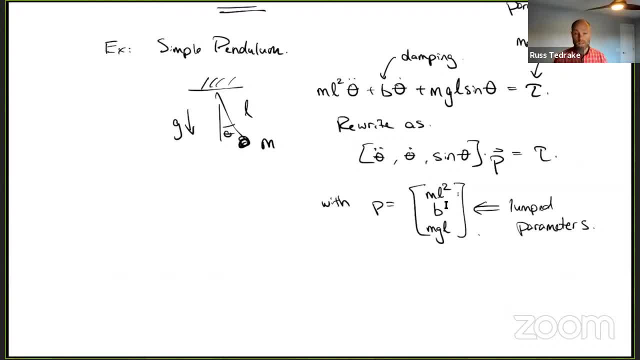 and or, even more accurately, we'll be estimating a subset of those lump parameters, or a low dimensional version of those lump parameters, which are the identifiable lump parameters, And that's something there's a lot of understanding about and it's not somehow. I mean, there are a few cases. 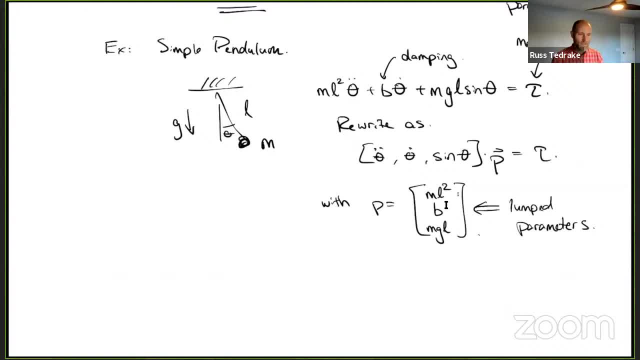 where you might actually need to know mass and length by themselves, Like if you wanted to write your results of your system identification to an SDF file and then send it to your friend or to your other process and to your controller, or something like that. 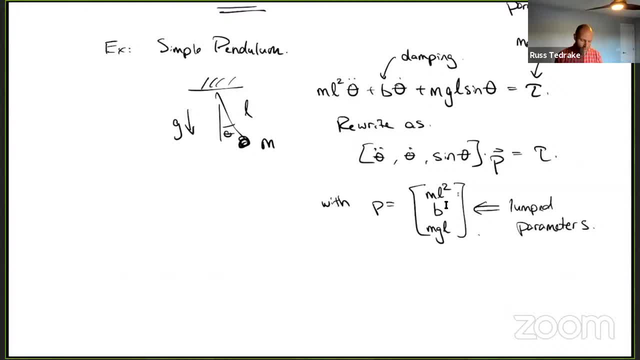 there might be reasons like that, but actually it's only the lump parameters that affect the dynamics. So they are the only things that you can estimate from the data And they are the only things you need in order to predict the future. So, if you have, you know. 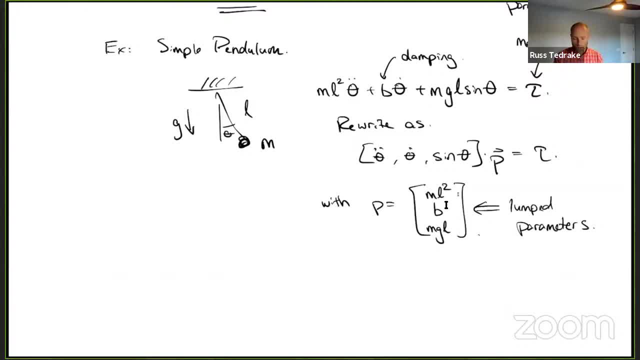 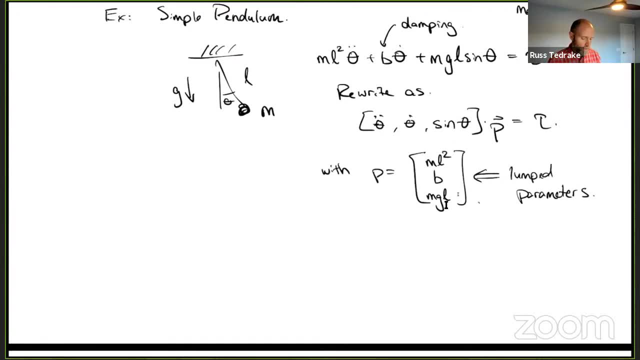 if you havestart in MGL as independent terms, then you know you have everything you need to predict the future in these equations. It's only you know somehow. the natural parameterization that we write in IRDF and the like is: 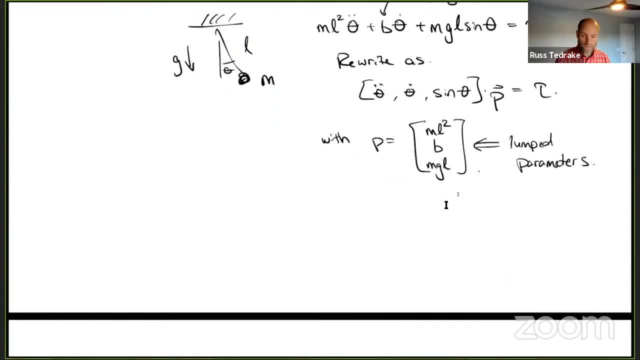 in some sense in overparameterization of the problem. Okay, so yeah, in this particular example, if we assume we know g, then we could get everything. but that's just unique to this example, i would think. but is that if you assume you know g, then you could? you could? 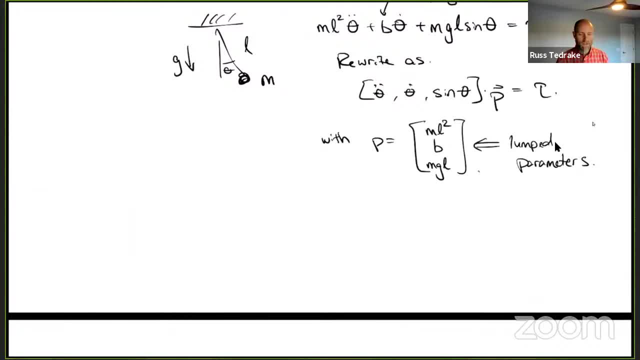 back out m and l, yes, and then, and then you could get everything. that's true. this, this particular example, um, yeah, that's just this example, and you have to, yes, so, um, for instance, if you can check, check, i'm just checking my physical quantities, but you know, if torque was zero, we wouldn't be. 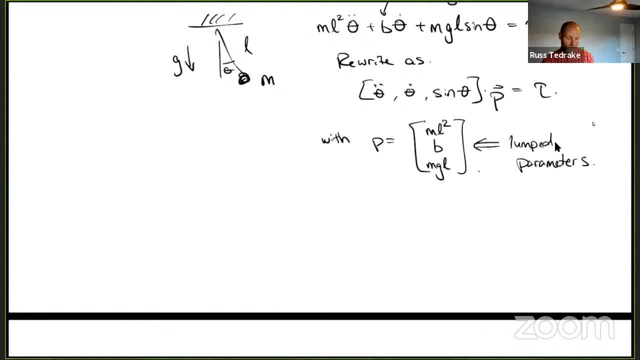 able to estimate. we shouldn't be able to estimate the mass of the pendulum, and that is true um. but you're right, if in this case we know g, we could actually back them out. and there are cases where you can back it out exactly, but they're rare and i think the more important case is when you can't. 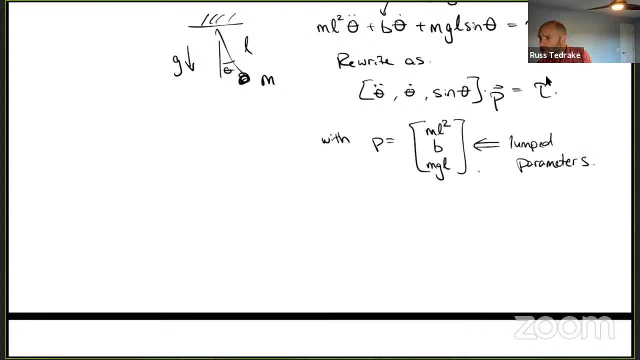 the more general case- i'm sorry, i just saw the chats- uh, since gravity acts on the center of mass even in the 3d case. oh, i just said. i just said this in the planar case, so i didn't have to write a 3d uh rotation. that was just yes, but you're absolutely right, same thing in 3d good. 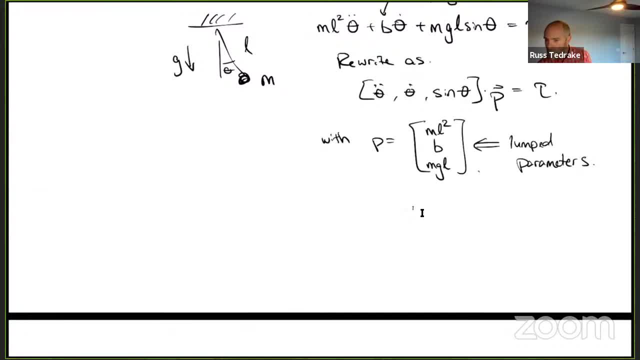 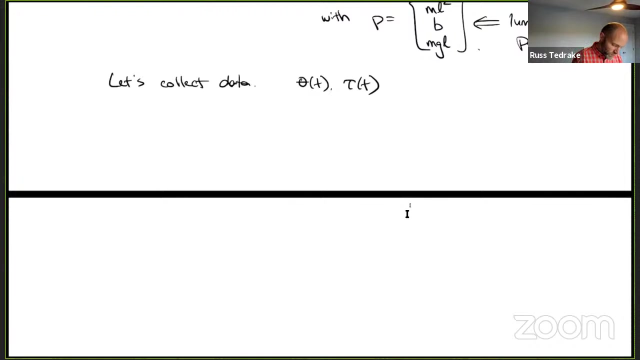 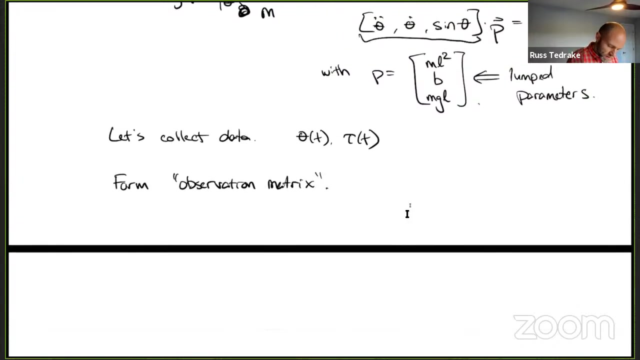 yeah, um, okay, so. so let's collect data, which fundamentally is in the form of trajectories of theta and torp, and then we'll um form the data matrix or the i will form the observation matrix- can i call this this term here w and we'll form the observation matrix, big w. 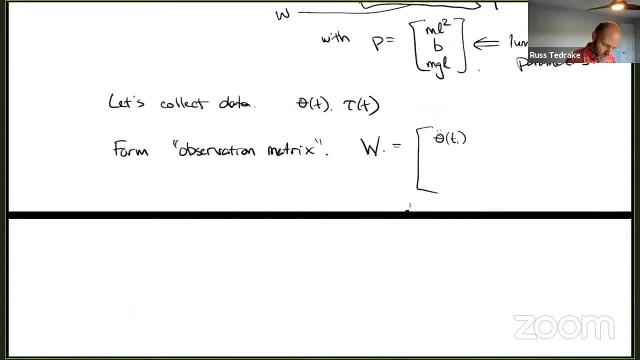 which is just going to be all of our data stacked and stacked up like this: okay, and then um same thing for tau on the on the right hand side, and we now just go ahead and set the thing up. so we're going to do this and we're just going to. 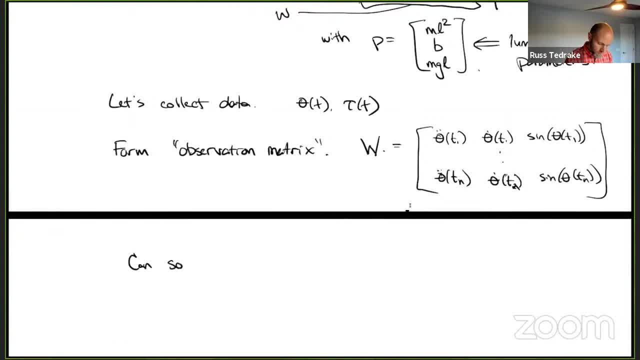 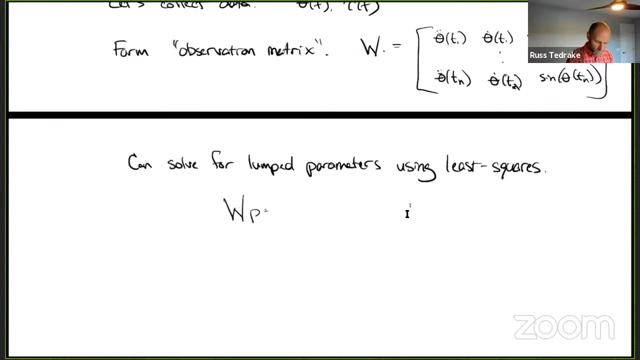 can solve for the lumped parameters using least squares. Okay, so this just becomes a big WP equals general. call the right-hand side Y, but let's call it tau for now. Now let's think a little bit about what that least squares. 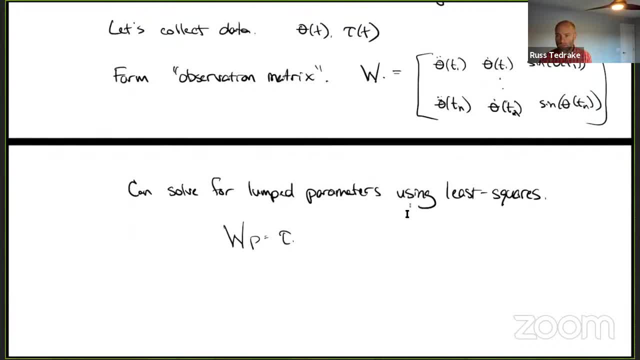 problem is going to look like right. So, like we said, there can be cases where not everything is observable. So, for instance, or is identifiable, I should say, for instance, the mass of the ball should clearly not be observable if I just observed it flying through space, right? 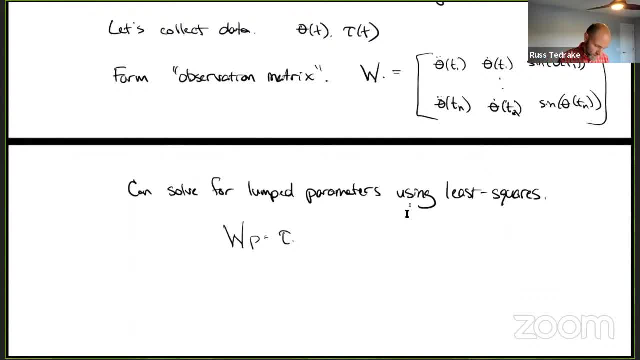 So if I just observed it flying through space, how would that play out? So if I had M, X double dot equals zero, right? Then if I write the data matrix, whatever, I'm going to get a bunch of X double dots. 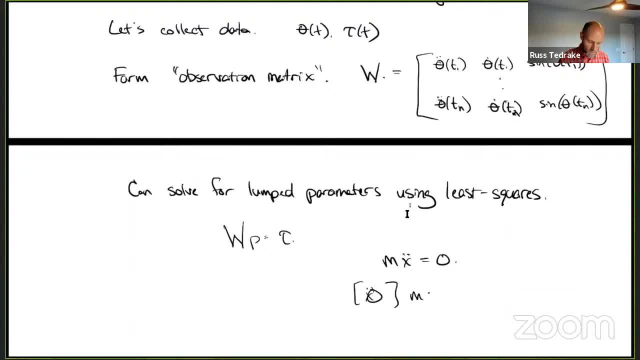 which are going to be zero. right, I'm going to get a big zero. matrix times M equals zero. It's going to be deficient, right? And there are other cases where you would expect to be have written down your equations that have parameters. 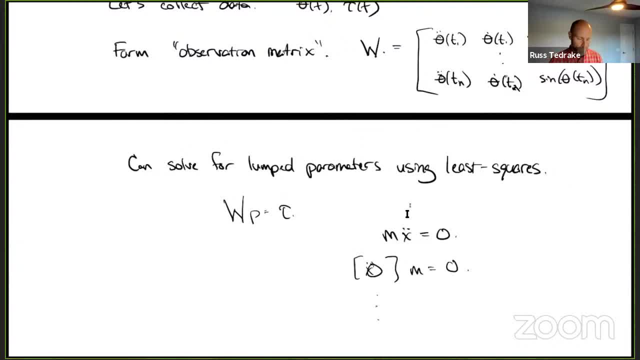 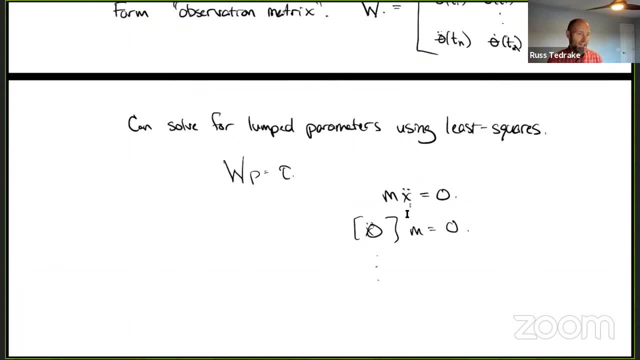 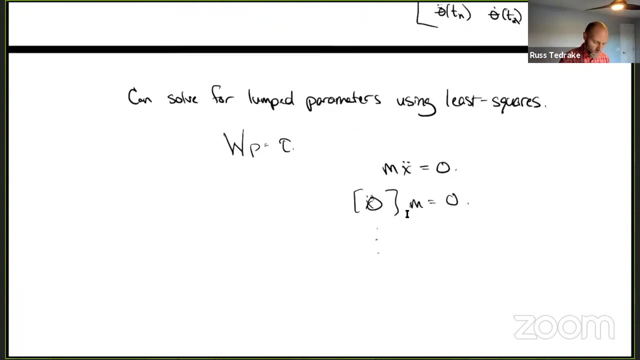 but there is nothing about the trajectory you're observing that can account for it. Like we said, if the torques were always zero and you dropped your pendulum, then you would not be able to actually estimate those parameters. So what does that mean, sort of in terms of well, 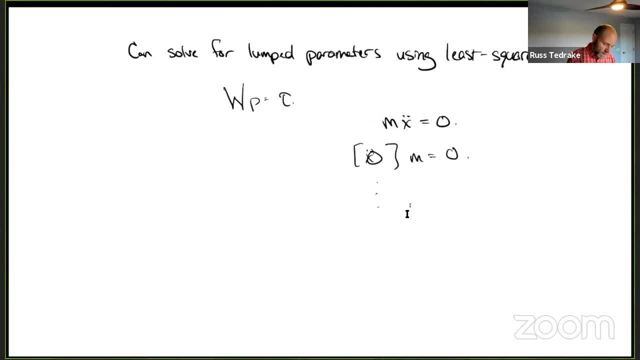 in terms of practice. somehow, identification is going to require some sufficiently exciting trajectories, As in parametrically exciting, I guess also, you know, for personal interest, exciting- but some sort of sufficiently rich trajectories. they can sometimes called parametric excitation. 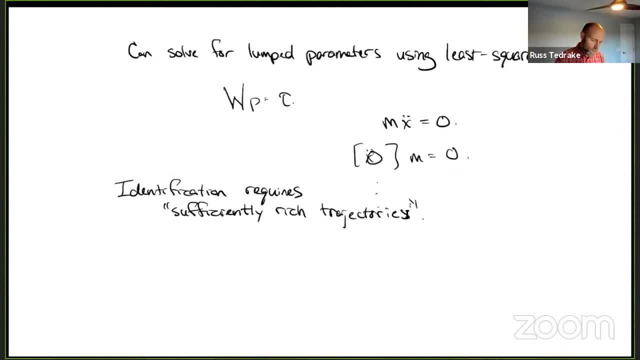 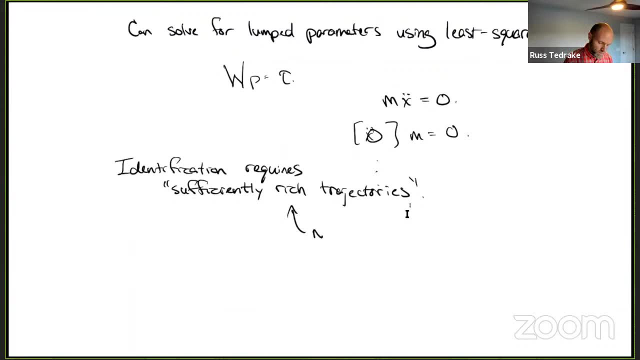 And actually the some of the some of the equations, well right Will show, will give a prescription for how you might do that. In fact, You know, this can be actually a nice motion planning problem. For instance, people will do trajectory optimization in order to find a trajectory which will move the robot through. 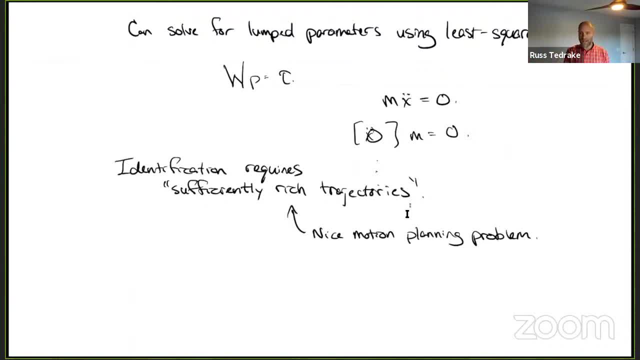 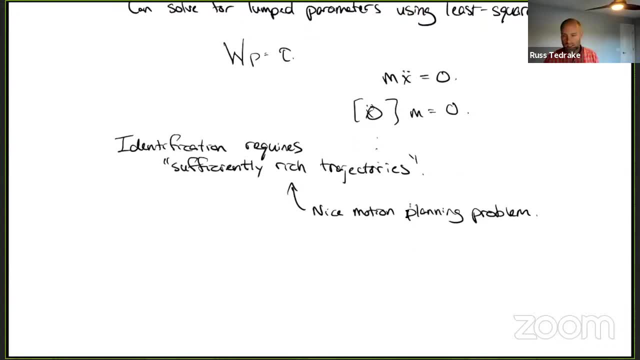 In order to maximize and information metric on the rank of that data matrix. Basically, somehow that could condition number of that of this data matrix. you can actually design a torque so that that matrix has a lot of information in it. Okay, but You know, we, we, we, you know. 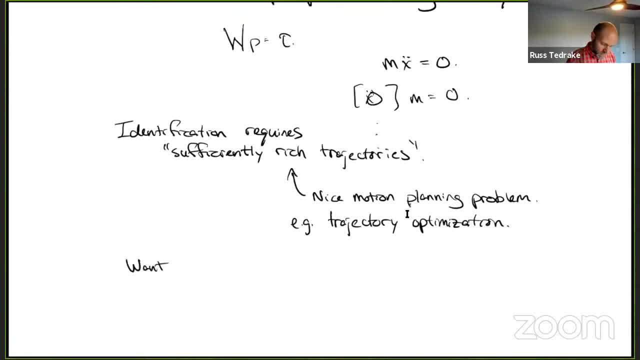 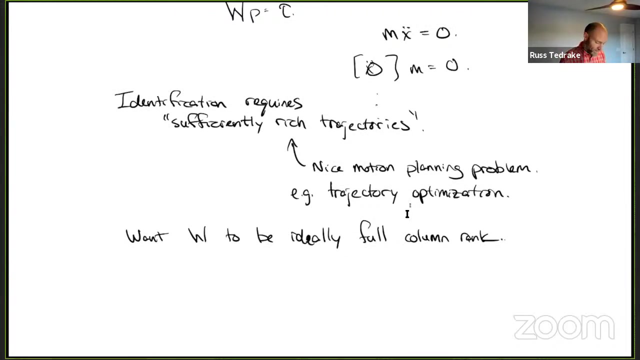 We would like, Ideally, full ring. We can't always achieve it. A lot of times there are parameters that you just simply can't know. In that case, We talked about the Identifiable lumped parameters, Which, in practice, we don't get. 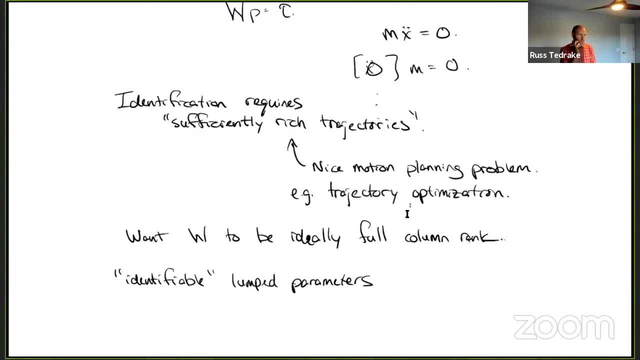 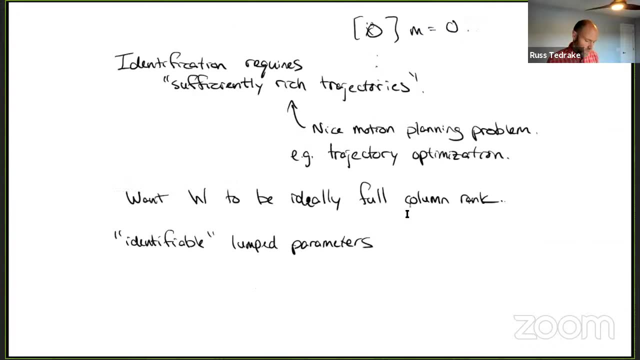 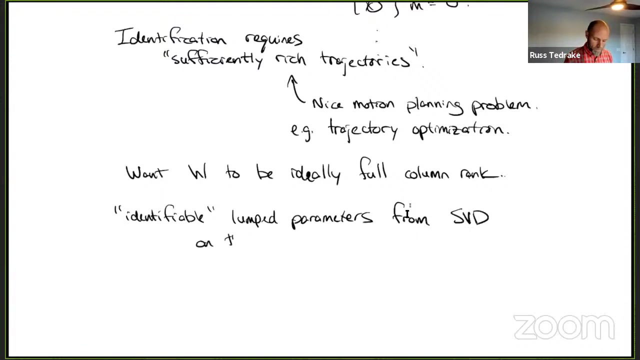 The state of the art algorithms for for finding which of your parameters are are identifiable, typically runs through getting a data matrix And just look, just doing numerical linear algebra on that data matrix, to basically SVD on that data matrix, singular value decomposition, And that can tell you the 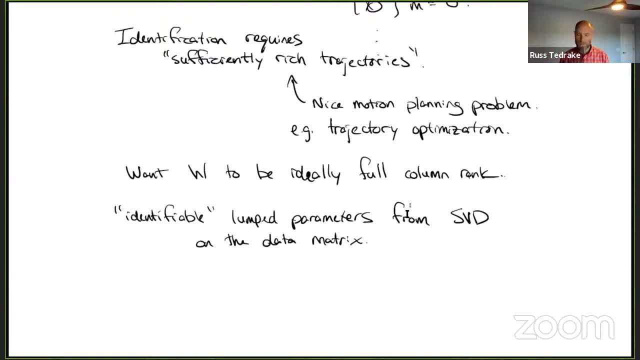 The subset of your or the subspace of your, Of your lumped parameters that are purely identifiable. So Take an example, for instance, the equations of motion for our Ewa right. so so in the URDF we clearly have, you know, moment of inertia for all of the links we have there, the kinematics of the arm and the like. 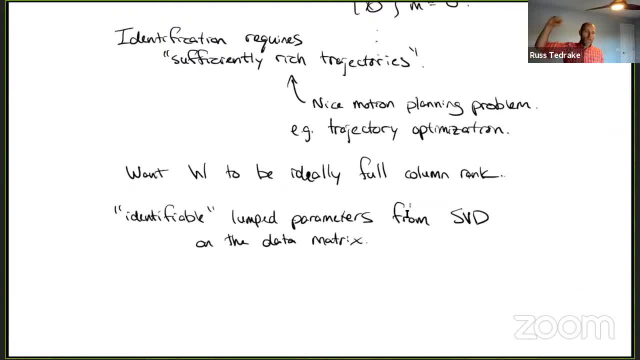 But if you think about the first link, right, nothing we are ever doing with the robot is going to it's only. we're only ever rotating that first link around one axis. right, because there's only one axis between it and the world. We are not doing a method. 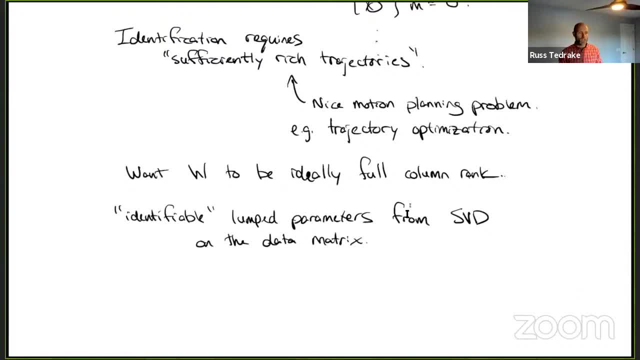 So. So there are directions in the inertia matrix that we simply cannot measure, cannot excite, right? so any reasonable sort of natural parameters asation of the Ewa Identification problem is going to need to admit that he can't estimate those parameters. And it's not bad. You don't need to estimate those parameters in order to predict the motion of the Ewa right there, and somehow you just never needed to write them in the 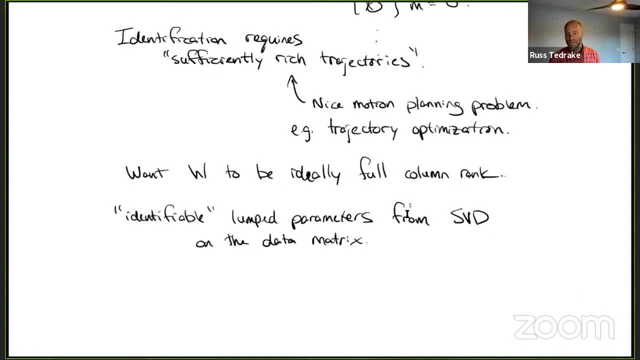 In the URDF, There, there, There, there, there, there, irrelevant, until you need to like, carry the Ewa to the other, to a different lab. Okay, so you know, that's the very basic setup. is this idea that we're gonna write the lump? 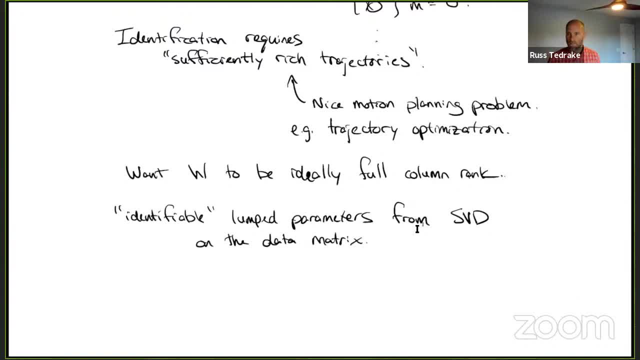 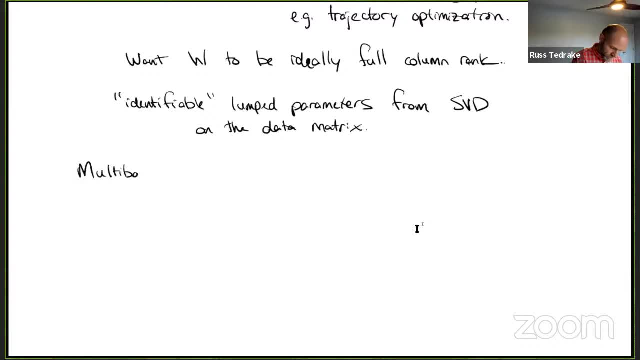 parameters. Let's think about how it looks in the, in the multi-body case, in the more than the pendulum case. Okay, so the equations I've written a few times throughout the term here of our mass matrix plus our Coriolis terms. I will not include contact forces right now, although I think actually you can include them. 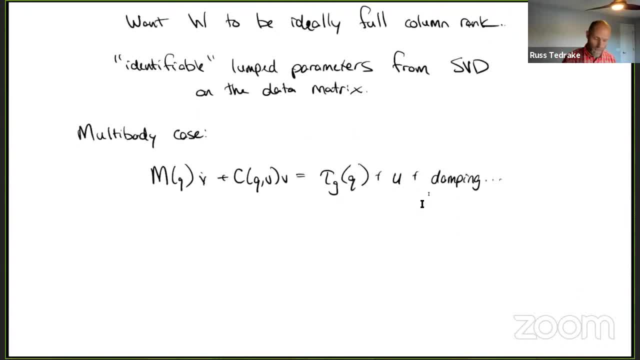 if you can measure them, but let's, let's not include them. yet It turns out even in the more complicated cases we can actually still write the equations as linear in the lump parameters. So this is now a big, complicated equation matrix, right um, with ml squared and stuff like this inside it, but it turns out all of the terms. 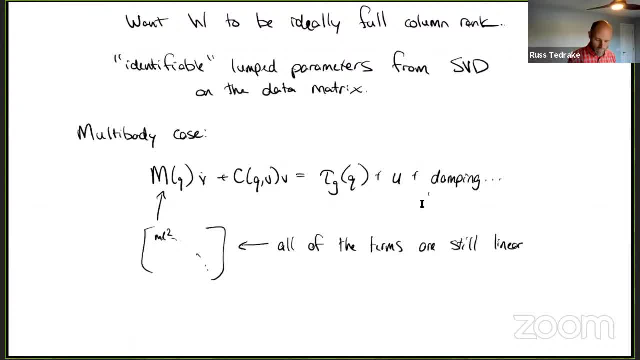 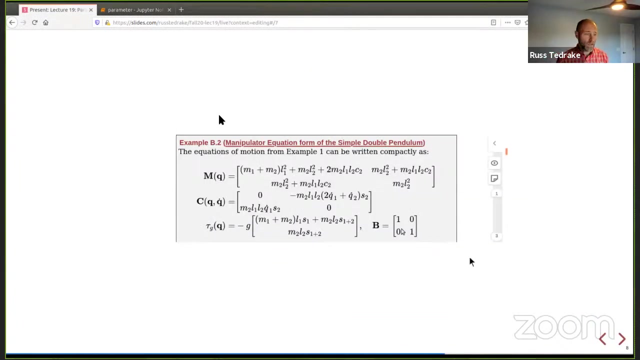 are still linear in the lump parameters. Okay, so, um, let's look at, for instance, the equations of the simple double pendulum, which is, um, just the two link arm. I'm sorry to scroll up here, but this is it's this arm here. right? so it's our the two link version of what I. 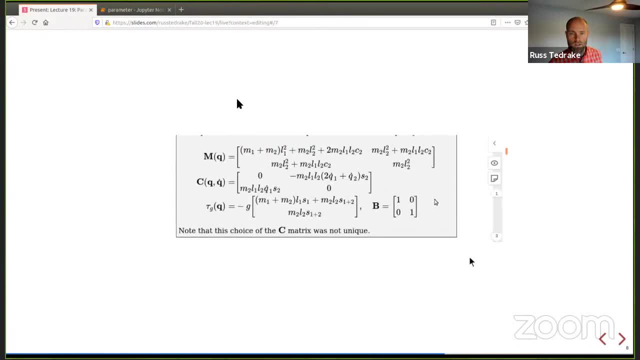 just wrote um the equations of motion. if you write them out like this, you know you've got a bunch of m? l squared kind of terms, you've got some cosines appearing, you've got some sine appearing. remember I use c and c, two for cosine, theta two s, two for sine s of theta two right. 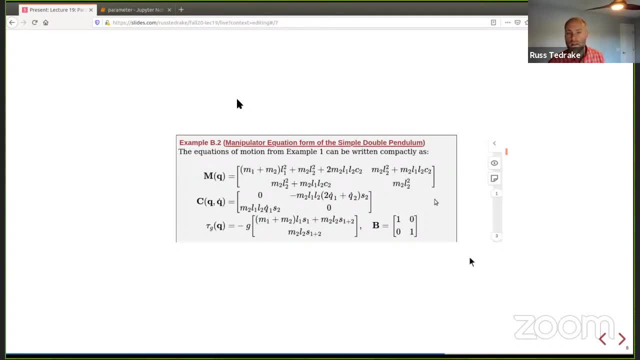 there's- you know it starts getting complicated, but still there's a separation that that occurs in all of these, uh, Lagrangian mechanics problems where the um, the, the variables of your state, are multiplied by your um, by your parameters, but in this sort of simple way. So I mean really, 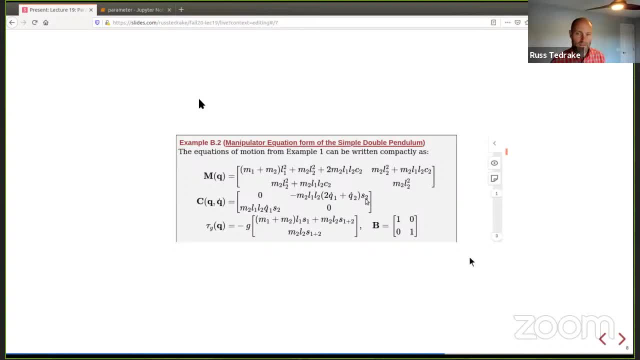 what it means is that you're never going to have your. you get sine of theta, you know cosine of theta kind of terms- sine of theta one plus theta two down here, but you'll never get sine of l theta or sine of m theta right. these things are always separable. I actually made that point when we were 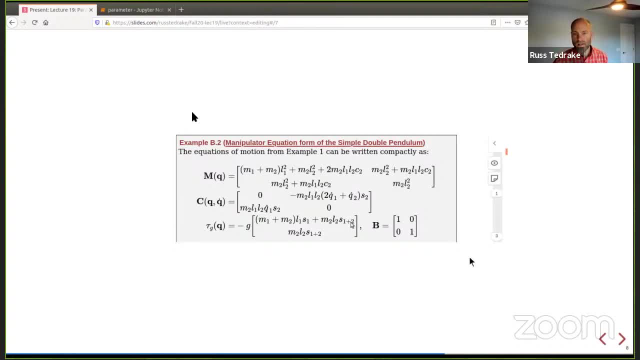 talking about kinematics being polynomial before right. somehow it works out that the terms are always simple in uh, simply divisible between theta and cosine. So you can get the terms of theta and uh and masses and lengths and stuff like this. So in practice we can actually still um do this lumped parameter trick. 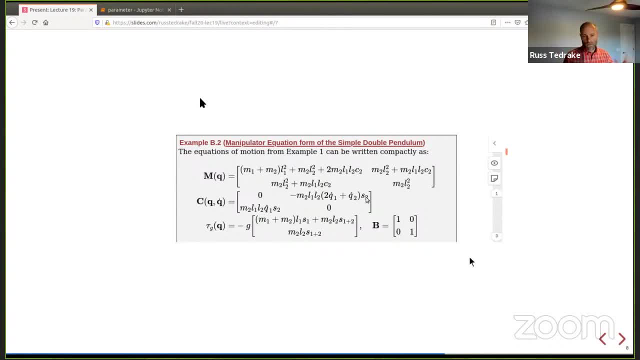 in a much more complicated um set of equations potentially right um, you now have a set. you know this is now a series of equations right in the two link there's two equations um for each, but you can still separate them out. the all of the you know, cosines and the like times, a single per. 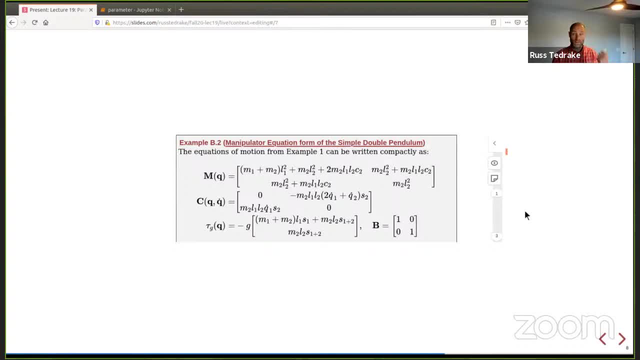 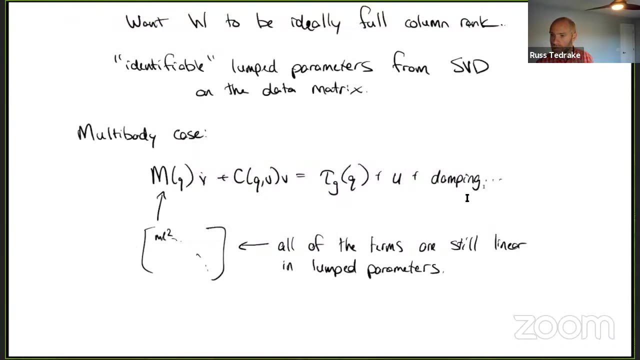 parameter vector equals my other, and I'll just have two equations now instead of one. Okay, and then I will copy all those equations down for my data matrix. I think that's sort of crazy, uh, and and super nice. So, um, if I did my forward dynamics. 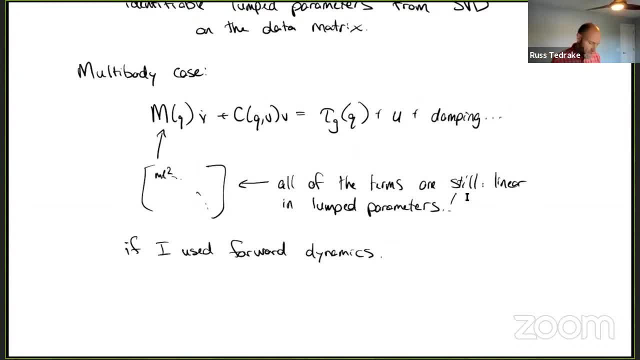 which is what I have in a simulator or something like this. right then I've somehow taken an m inverse and I have v dot equals m inverse times, all this other stuff, u minus or plus tau, g minus c. okay, this m inverse is um, you know, makes the the either. I have to somehow come up with. 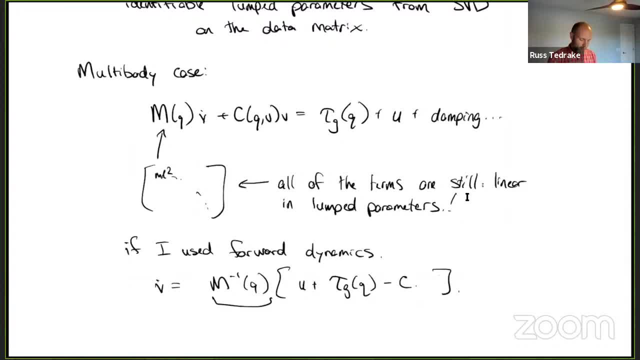 rational lumped parameters or. but even then I've got sine thetas mixing in weird ways that breaks the linear in the parameters property. okay and um. so if you don't sort of stay in torque space and you switch to acceleration space, then you've lost all this beautiful structure. 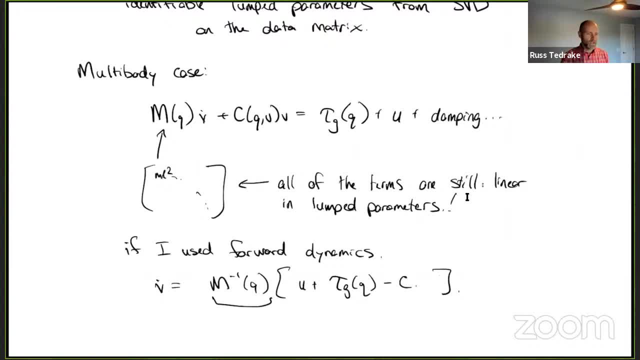 So if you're doing, you know, residual learning or model learning or whatever you know, I I think it's a good question to ask: is you know should you be doing it in q and in theta, in q double dot, or should you be doing it in torque space? because it's even if you don't start as a 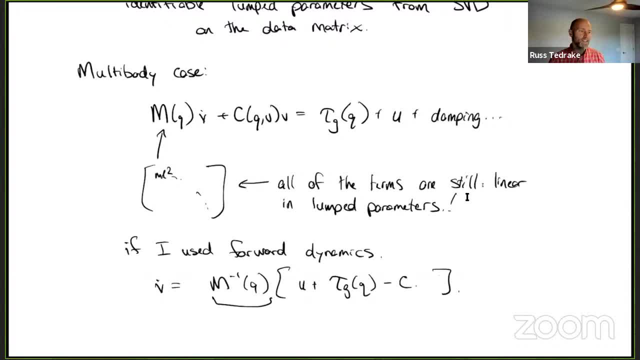 with a parametric model. um, it seems like the equations should be better in this space. So, um, let's stop for a minute and think about how you implement this right. so, um, it's actually relatively hard to type something like this in. uh, in the past, I think it would typically involve: 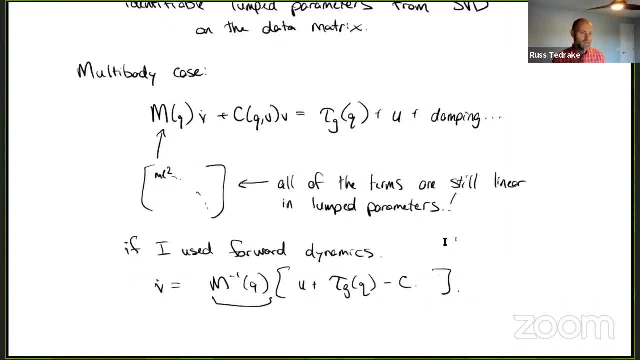 a small labor of love which, with um, you know, writing out the equations yourself, even for an eva or something like this, and and typing them in. and even today, there are very few people who are doing this. right now, There are very few um simulators that can give you, uh, access to the, the equations of motion, in this form so you can manipulate them in this way, um, but we do have a symbolic back end in drake, so let me show you that and 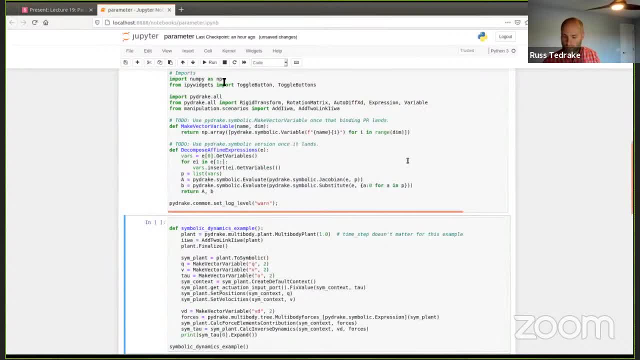 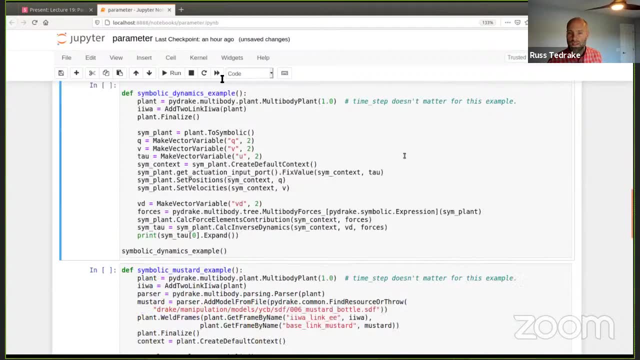 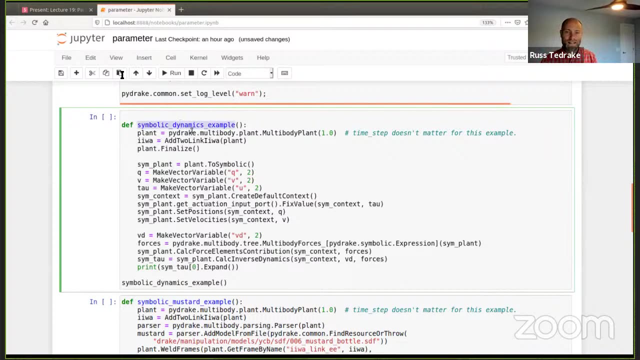 here's a jupiter notebook, okay, so I will. I meant I hoped to push it to you before lecture, but it's not quite done, almost done, all right. so, um, but let me show you, uh, that we, we have symbolic dynamics uh in in drake. so, for instance, if I just want to take my two link: 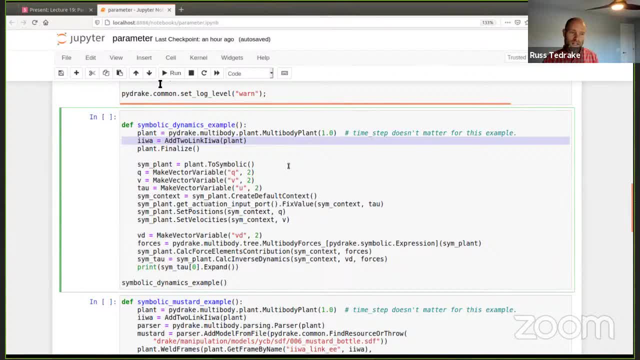 we can do symbolic dynamics for bigger evas, but you don't want to see me print it out, um right, so the equations get pretty big, pretty fast. We have this fancy thing right here at f and we just did it run out. let's start with f. w. Do i need everyone involved? It's not all the way done. okay, it looks more like it's generating moreと思- heißa lot of the material than i imagined, so let's try this. used해서what'i'llmex, cuidadoasd MaryseR. 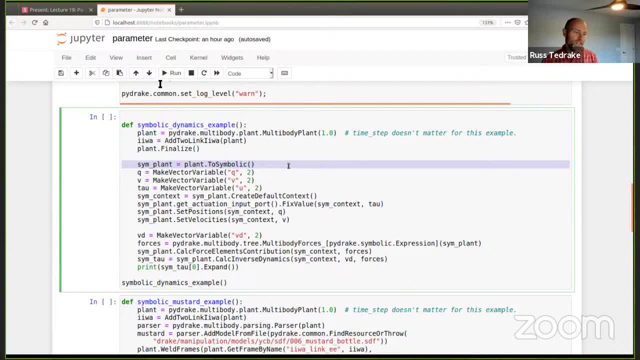 fancy thing which is changed to symbolic and you get a symbolic version of your plant, And then so, by default, the symbolic version of your plant just has a bunch of symbolic variables that are holding double values, and it will act like the original one. 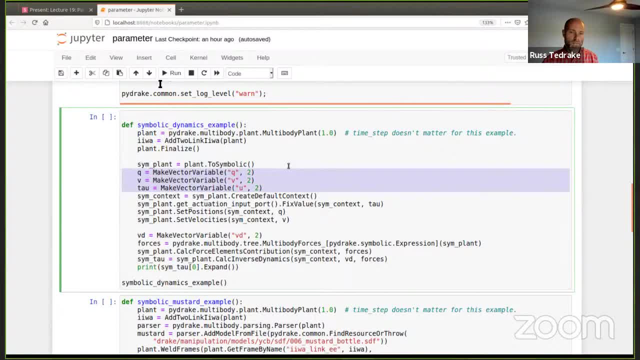 But if you go in and say you know what, I want a few of these elements to be variables so that I can track them, and you write those into the context, then you can calculate the inverse dynamics and print it out and get you know. 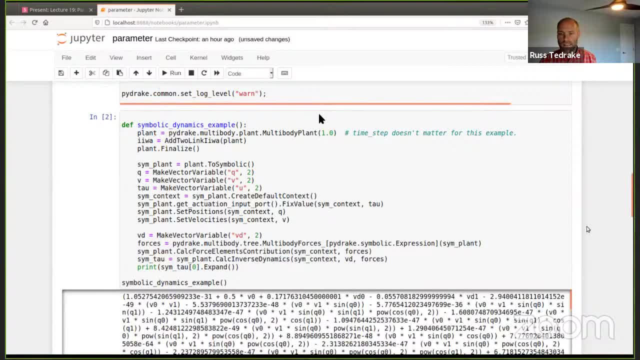 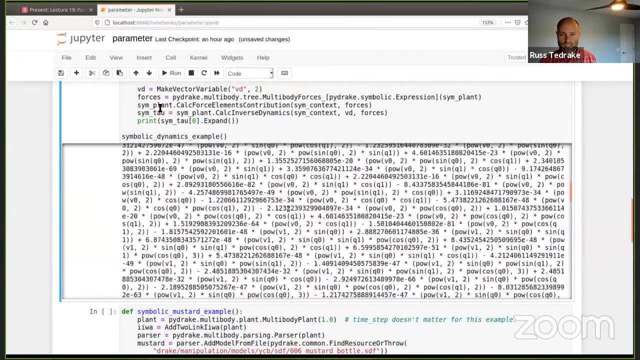 for whatever robot we're working on here, you can get the symbolic form of the equations of motion. If I were to, you could see it's already pretty big. Admittedly, there's some simplification that I didn't run, but you know there's some small numbers and everything. 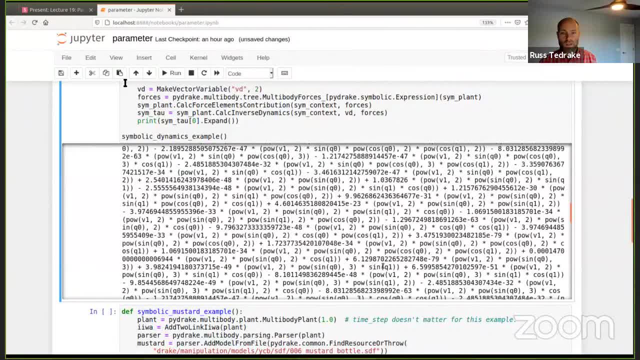 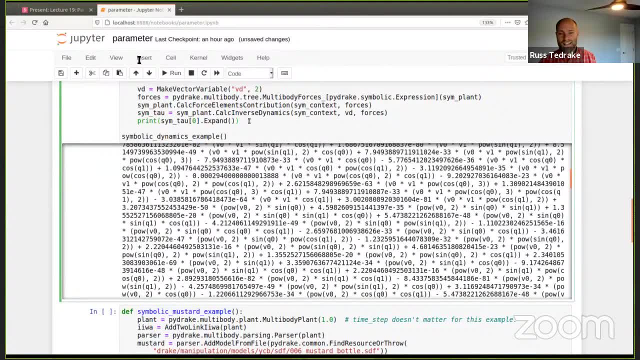 but equations of motion get really big really fast. If I had taken the M inverse, it actually I think it might've complained. Now the two by two case it'll do. but we don't even support the full M inverse because symbolic matrix inverses are crazy. 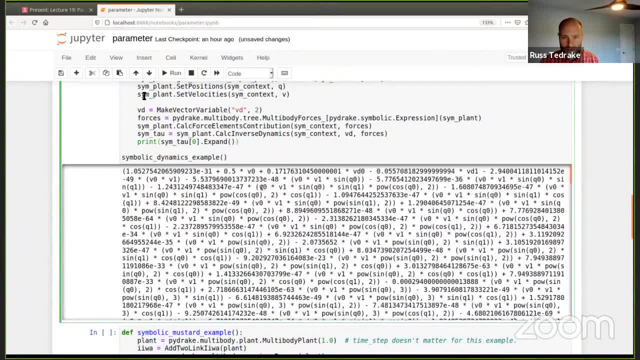 Okay, so this is cool, right, So I can actually see. you know the equations of motion and what's also interesting. So this is one that we could have zeroed, and we do actually have tools. I should have just written that. 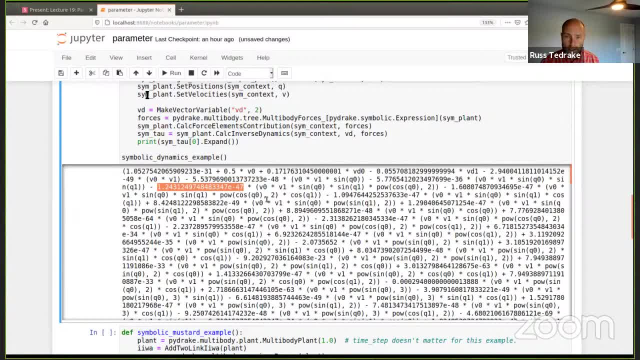 to zero out the small coefficients. But I can basically, you know, write out the full equations of motion, but in this example the masses, link, lengths and everything were just numerical values still. And so I get a numerical coefficient times this: 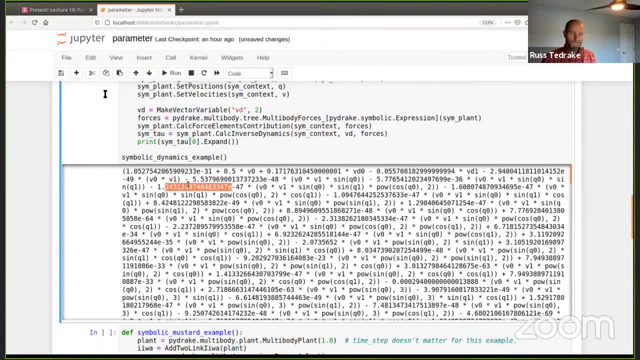 Now that's super important. is this interleaving? If you compare this to like Wolfram's symbolic engine, Wolfram will do everything in rational arithmetic. It's like, I think, the best out there. you know, in my experience it's incredibly good and super powerful. 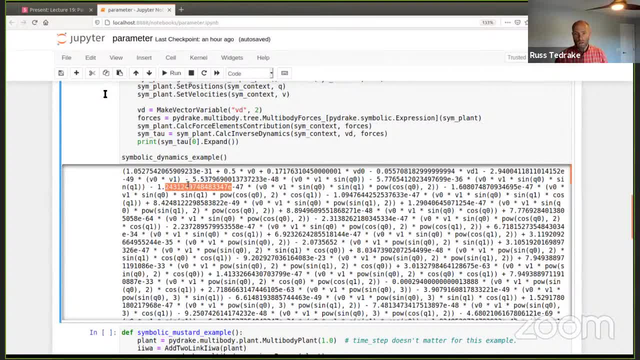 if you want to prove things and the like, but- and they have made it scale beyond what I would think you'd want to scale- but this is the symbolic we've chosen to implement and a lot of other packages that do symbolic will implement is a combination. 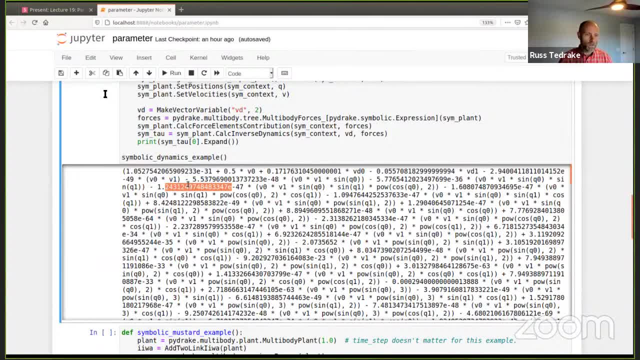 of floating point and symbolic right. So it's not trying to prove something absolutely. by keeping explicit rational numbers We've accepted there's some floating point errors. We have either the minus 47 garbage, but this will scale a lot better. We can take advantage of floating point arithmetic. 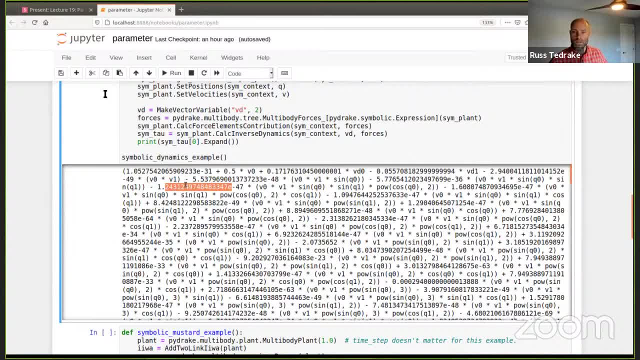 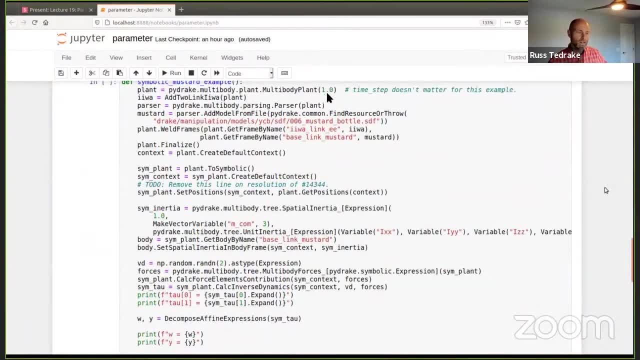 for the things that we don't care about, the symbols for and use symbols for the rest. Okay, so how would I set up the data matrix for? so if I've now taken a two link example- although this one I could have done- end links. 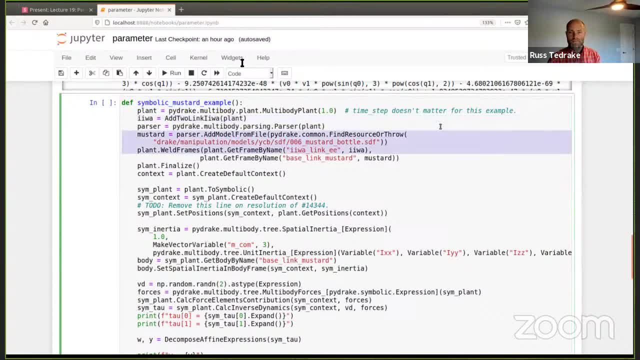 the full EWA and I'm going to just take the mustard bottle and weld it to the hand, why not? And then the interesting thing will be: can I wave it around? and without knowing the parameters of the mustard bottle, can I? 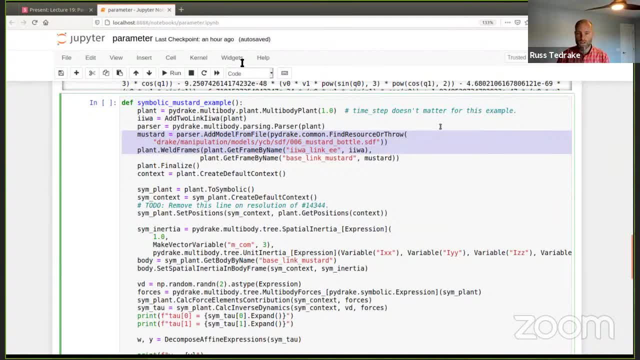 back out the inertia and mass and moment of inertia, sorry, the center of mass moments of inertia of the mustard bottle. Okay, so slightly different workflow. I'm going to change it to symbolic, create my context, And then I'm going to make the spatial inertia. 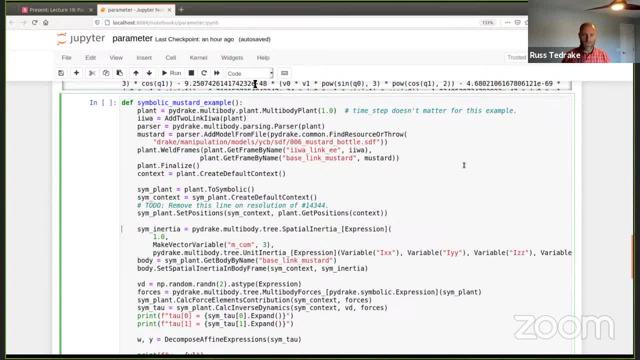 I'm going to set the inertia of the one body that I care about to be the variables, So I can even let me do this Slightly different workflow Slightly differently, so you can see, I'll do mass and just center of mass. 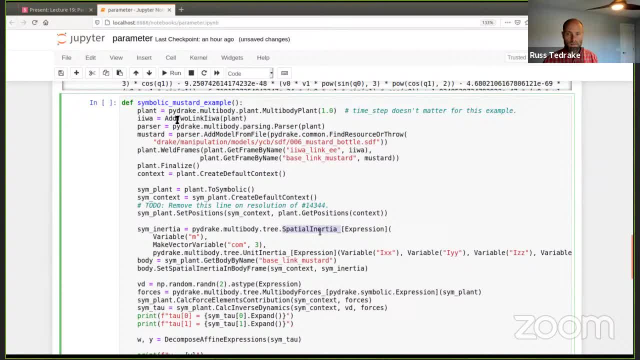 So this is. I know it's ugly reading code, but you know, I've got a spatial inertial logic which takes the mass, center of mass, And I made variables for the moment of inertia. These are the kinds of variables you'd see. 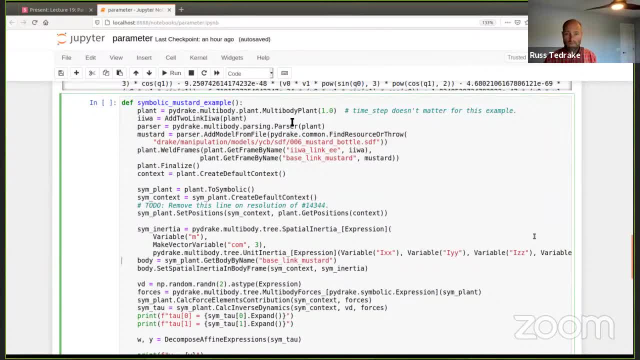 in your URDF file. okay, And I just set the spatial inertia in the context To be the symbolic one. So I'm going to track just that And then I'm going to again make some. just I'm just evaluating it at one point. 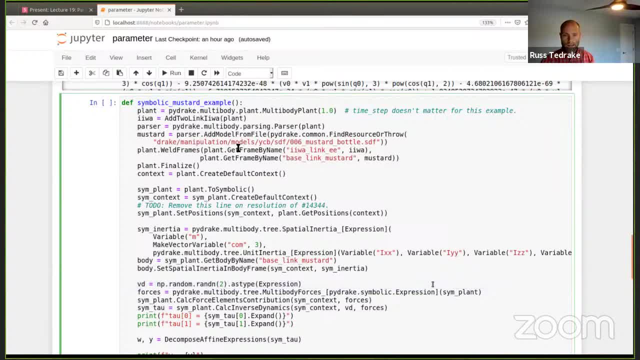 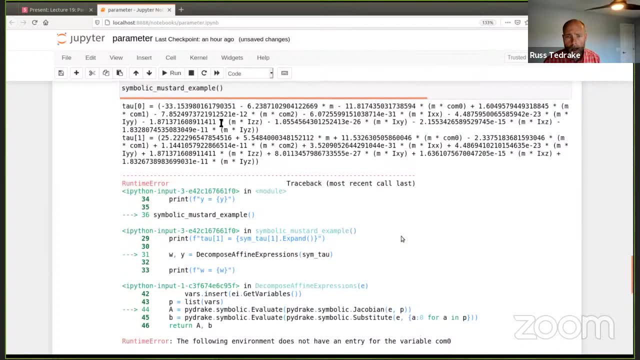 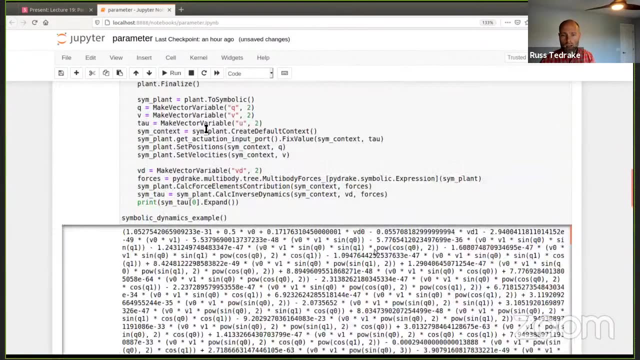 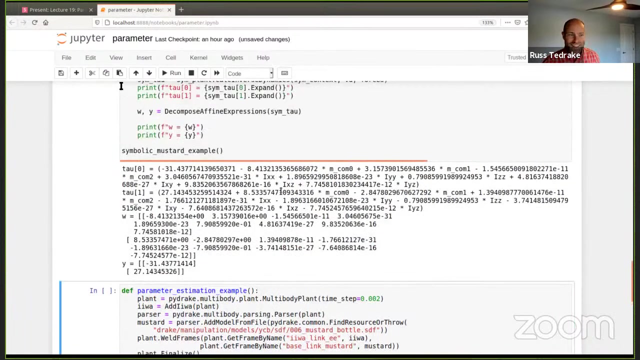 with some random accelerations, some random forces, and then we'll see what I just broke. it Did I. I'll do the one that worked best first, and then I'll change it. Okay, So there's two equations, right? The first one is: 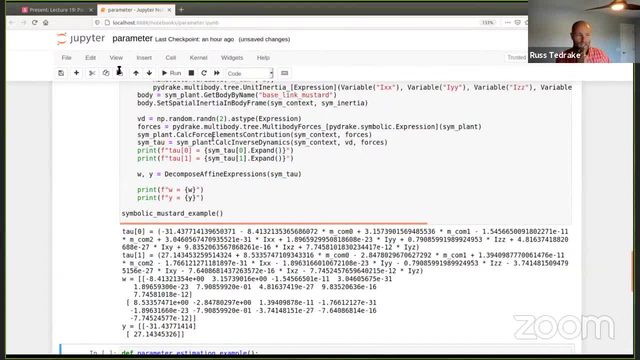 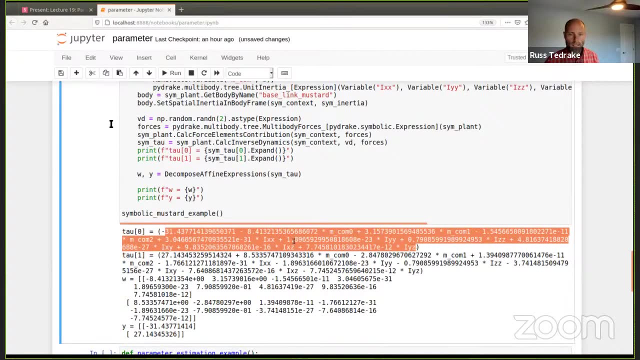 corresponding to tau zero. okay, That's the equations of motion of the first link, and tau one is the equations of motion of the second link, because the inverse dynamics are in tau, in torque space. right Now I get a more manageable set of equations where I took advantage of the floating. 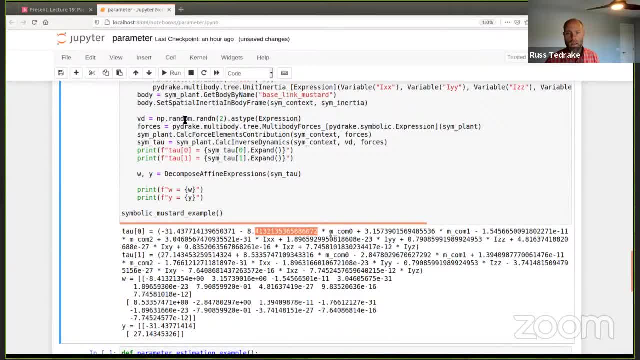 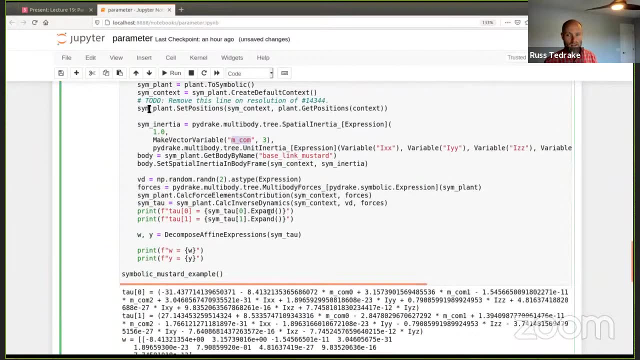 point arithmetic to do all of the floating stuff. okay, And I just have the mass center of mass, I and the like up here. Now the reason I set the mass that I had gone back through and set the mass equal to one and lumped in the mass center of mass is because I just cheated and did the lump. 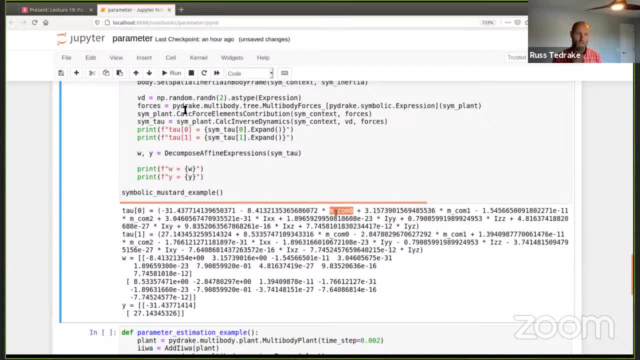 parameters myself. We have code actually that will extract the lump parameters for you and do the insertion, but it's just a few lines that we didn't need. It was trivial in this case. The only time we did that was when we did the insertion. So we did the insertion and we did the insertion. 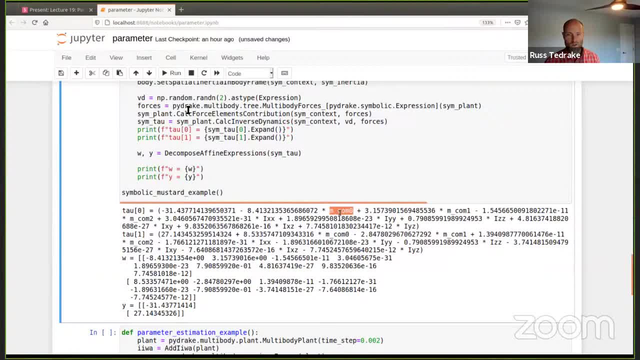 and we did the insertion. So we did the insertion and we did the insertion. So the only time the mass entered the equation was over parameterizing. It was multiplying times: the center of mass and center of mass zero, one and two. okay, So I calculate the inverse dynamics and I printed 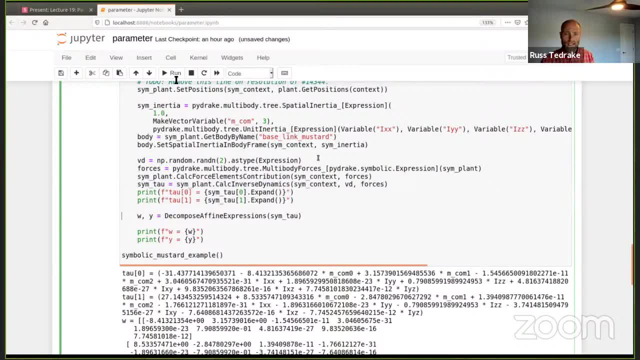 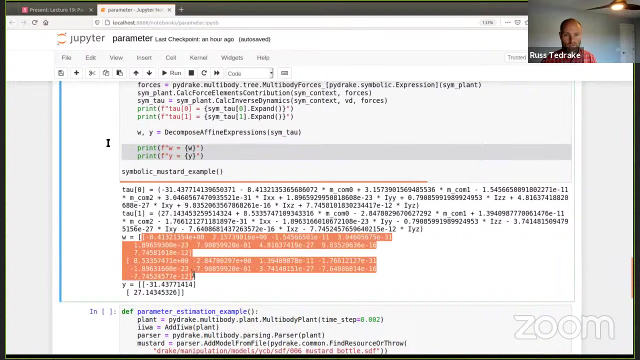 out tau zero and tau one And then I can extract. so from those equations I can extract basically the A and B, the data matrix and the Y matrix. okay, So I've got my Robert Alverson- Why? and then my my w and y data matrices and they come out like this: So I get: I expect w for this for this system to be a two by. 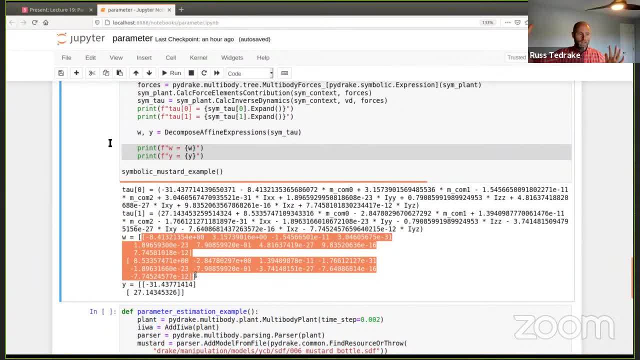 Robert Alverson- By number of parameters, Robert Alverson- And my why to be to like that? two equations? Yeah, Robert Alverson-. So if I now want to estimate mass, centered mass and the like, All I have to do is run the robot a little bit. 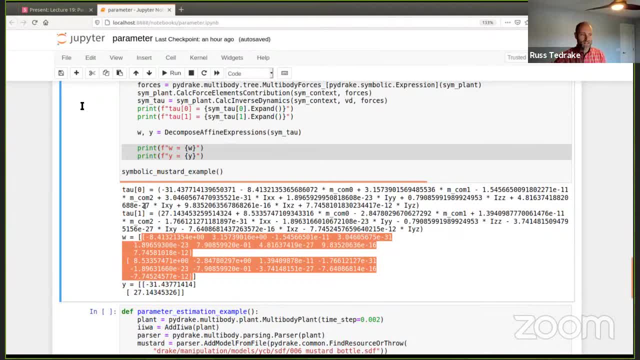 Robert Alverson- You know, move it around. have it be sufficiently exciting? If I just set torque to zero and let it fall, that might not be enough to recover the parameters. I would see that the data matrix has Robert Alverson- His insufficient rank. But if I wiggle it around enough, especially with the 3D robot, and you know, just do these squares on that- then then I can recover the parameters and I will 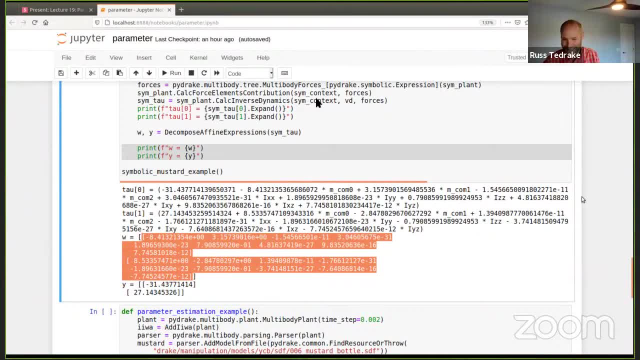 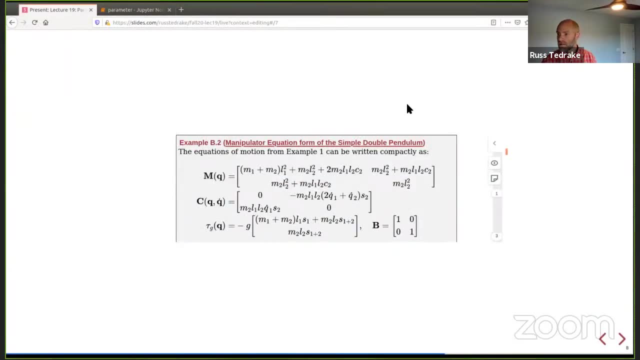 Robert Alverson- Will provide that tonight. Robert Alverson- I got it almost. Robert Alverson- Had to add some bindings late last night. Robert Alverson- Okay, so um any questions on that? I have a question If you have. 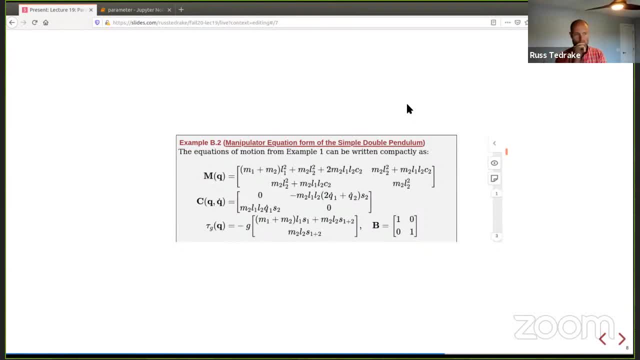 Enough samples, such that the problem is like over constraint, like in this specific simulation setting. Robert Alverson- Um, it's the error of the least squares problem going to be zero, like Robert Alverson- Your model is exactly what you defined. Robert Alverson- Does that make any sense? 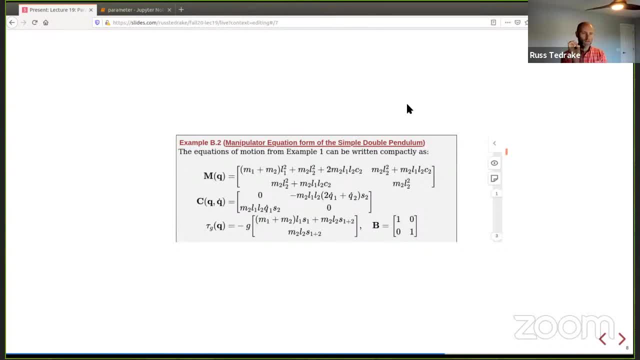 Robert Alverson- So, okay, if my accelerations were perfect, Right? So, Robert Alverson-, Then you could get, could obtain zero error, Robert Alverson-. But that's absolutely a weird corner case. I think even in simulation, If you simulate trajectories with some OD solver and then tried to back out the accelerations, for instance, you would see some residual there. 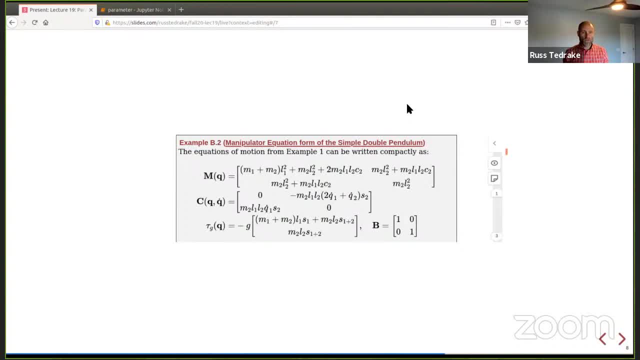 Robert Alverson- Having, Robert Alverson- Having too many rows in the matrix is what you want, Robert Alverson- Right, Robert Alverson-. You want to be in the case, Robert Alverson- Where you use the power of the data to be fighting down any of the noise in your in your measurements. Right, And certainly there's cases where 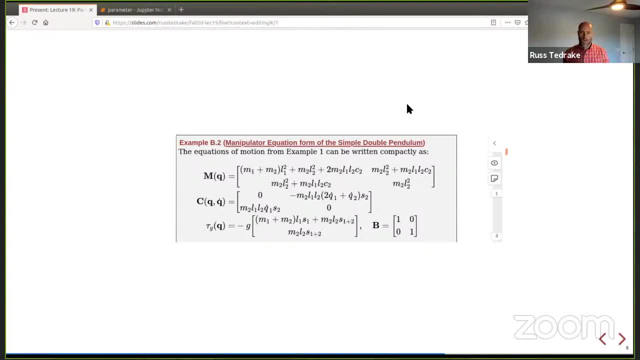 Robert Alverson- Yeah, I mean, we're actually going to. That's what I'll say. next is Robert Alverson- The formulation I've showed so far of using Q double that. that's something that's sort of reasonable to do in simulation. but actually you know there are better choices for for choosing those. 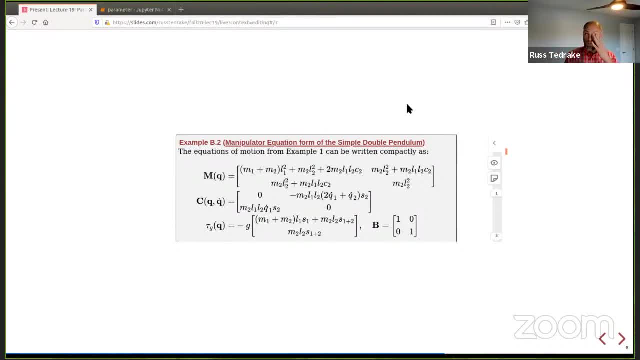 Robert Alverson- You know you want to assume you have accelerated noise free acceleration measurements in unreal robots. Robert Alverson- Right, Robert Alverson- So so yeah, I think in the one corner case where you've calculated everything perfectly, You can put it into the matrix and come back. you'd get close to zero error. 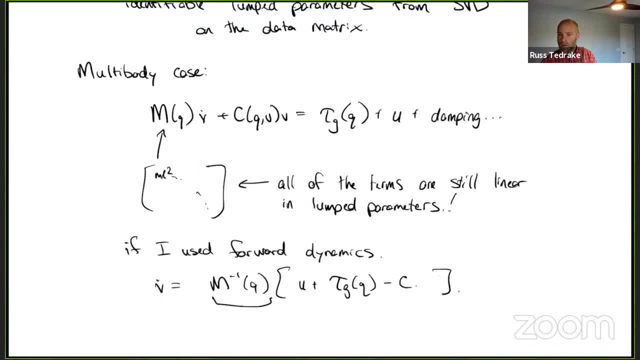 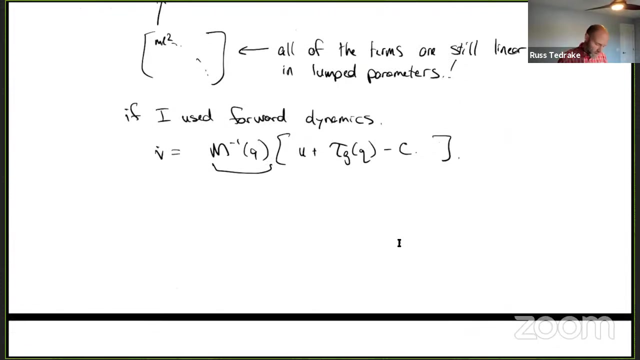 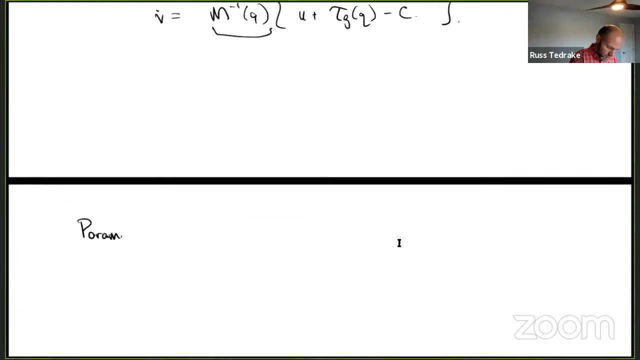 Robert Alverson- Okay, Robert Alverson- Okay, Robert Alverson- You, Robert Alverson- Okay, Robert Alverson- Okay, Robert Alverson- Yeah, All right, so the parameters I wrote there and, in general, the parameters of the 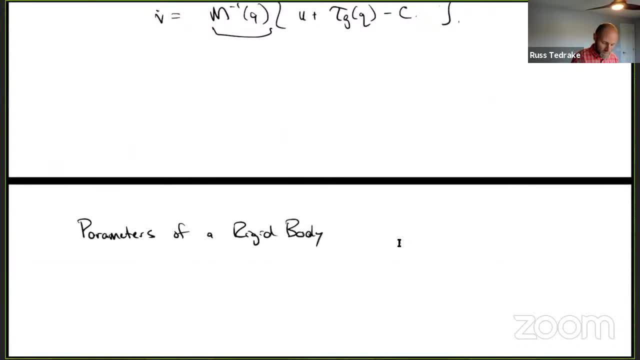 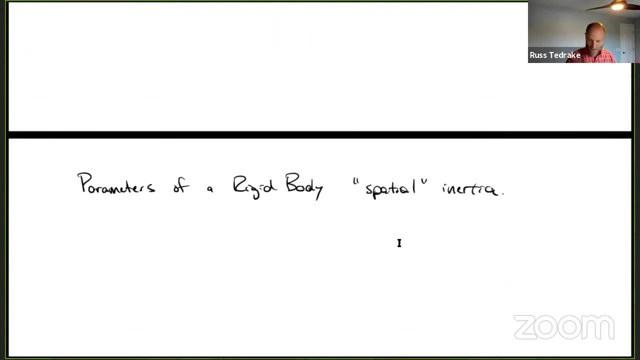 single rigid body, spatial inertia, which is just the six by six version of the concept of inertia. you know it lumps the center of mass and everything together. So the parameters are, you know, the mass, the location of the center of mass and the 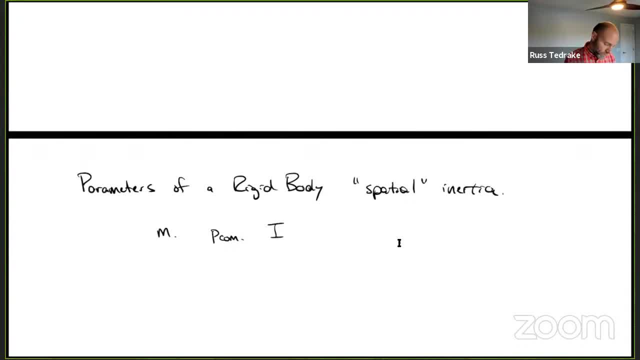 inertia of mass. The unit inertia which we tend to parameterize is a bunch of parameters: i, x, x, i, y, y- This is how I wrote it down just a minute ago. So six inertial parameters. Now there's a couple of things about that. 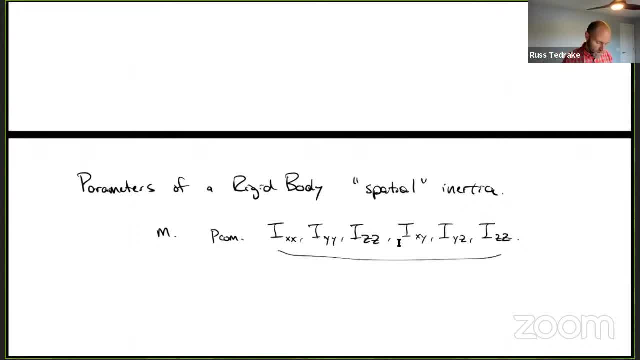 So I already said we can't- I separately identify these from the mass. So it makes sense to lump in the mass and the center of mass if this is somehow an overparameterization. So I set this to be one and allowed the center of and instead wrote m times p, center of. 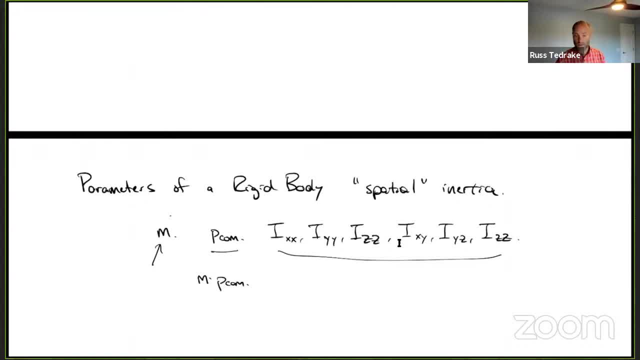 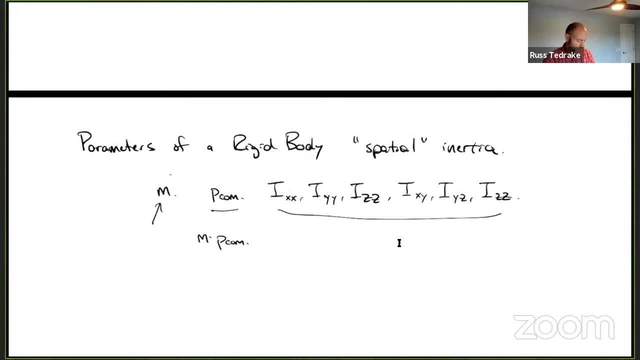 mass and this would be sort of m times the unit inertia. Okay, But even then there are more advanced things I could do. I think the the approach for for doing the mustard bottle and figuring out or even throwing a banana. I think probably just doing least squares on this is going to be just fine. 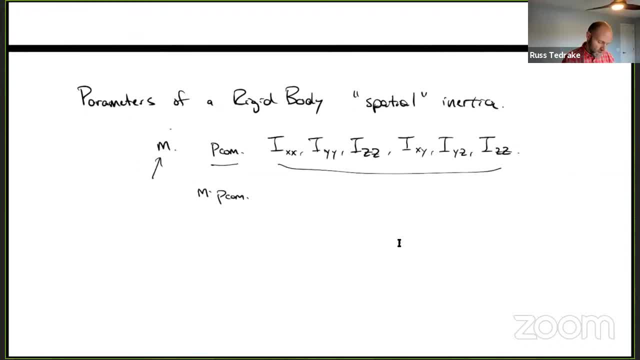 But, more generally, there are things to be careful about, right? So this is, this is six numbers to represent a three by three matrix, because we're assuming it's symmetric, Okay, But not all values of this will define a physically plausible inertial matrix, right? 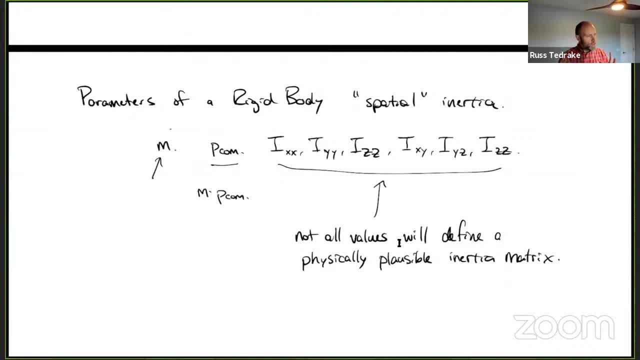 There's, there's. if you're three by three, matrix has to come out. Okay, But not all values of this will define a physically plausible inertial matrix of, of, of something that has mass and density, you know then, then it can't. actually there are extra constraints. 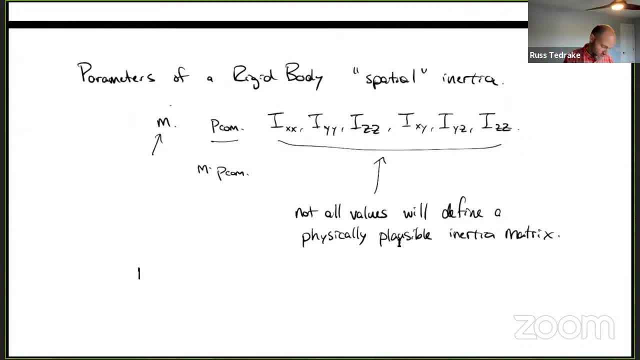 besides it being a symmetric matrix. There's a nice paper from Patrick Wenzing who was here in Songbei's group a few years ago. I'll cite it in the in the notes you could add that to the add the constraints to make physical plausibility for the inertial. 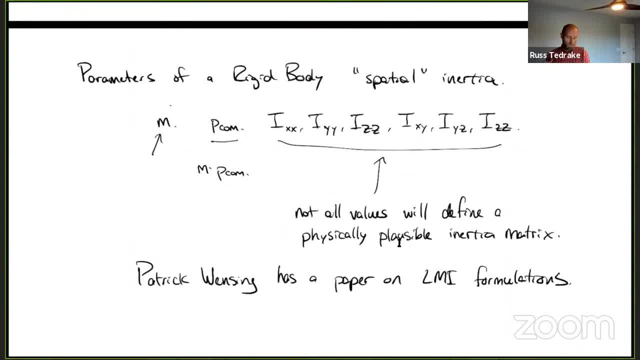 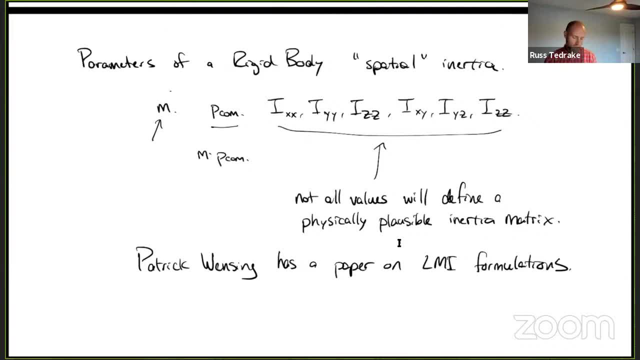 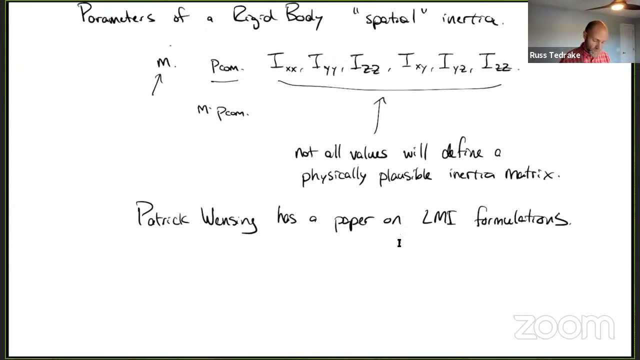 matrix, you know, add that in and try to solve the for only physically plausible inertial matrices. that's a detail that most people don't include. it's a. it's a nice thing to include. okay, it's cool that it's easy to easy to add. so, like, I don't know, so it's, I think it's super cool that. 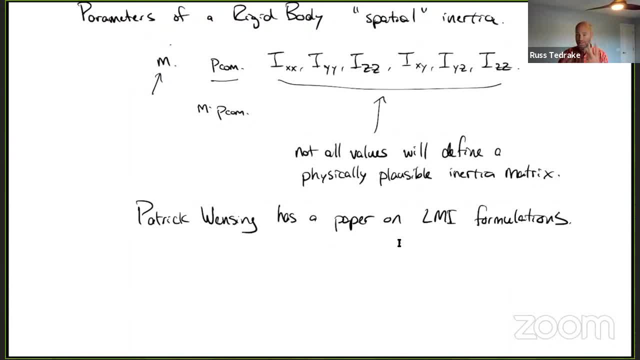 we have like lmi solvers and symbolic equations of motion and you know, and all this like sitting in one toolbox because you can, you there's things like that that you can kind of, oh, I can put that together and it's pretty easy, which is pretty rare, okay. so the but the biggest problem with 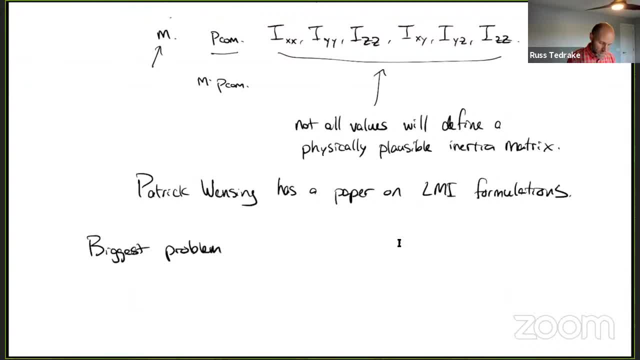 what I've written above is assuming we can measure clean estimates of the acceleration, and there's a bunch of different approaches that will that people consider to be better. you know, just flat out superior to assuming q double dot. you know, as I was writing this up this morning I was thinking: 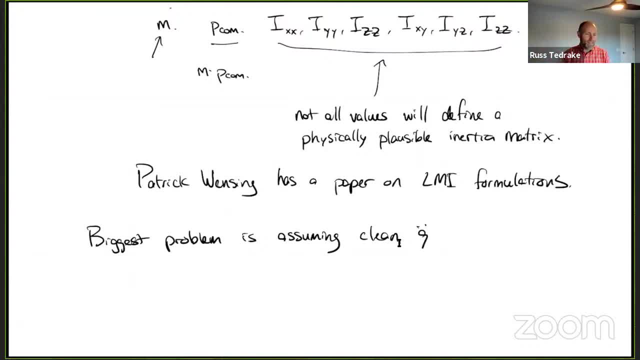 that you know, there might be some, some time and maybe it's, maybe it's even here, maybe at some point, maybe we're gonna. that's just gonna be an old, too old thing. maybe we can. just you know, we have high enough quality sensors and we can. they're running at high enough. 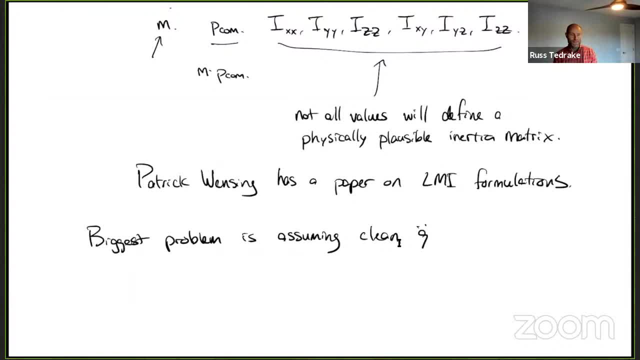 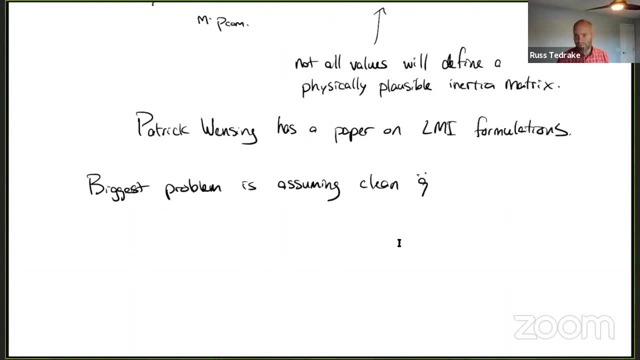 rates that we can somehow get accelerations perfectly, and- and everything I'm saying is is like old school, I don't think we're there yet. I think right now it still sucks to to use accelerations. so there are a couple different alternative formulations. it turns out that there's a, there's a way to basically- I mean, you fundamentally can't ask for. 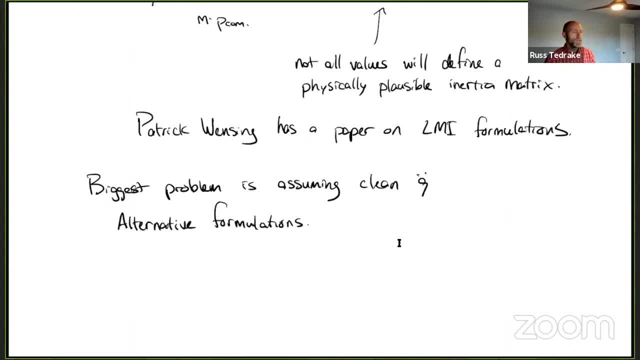 the torques to match the accelerations anymore. so what do you do? what do you do? what do you do you do? well, you can. you can filter both the left and right half side of the equation and look at basically the longer term effects of the acceleration changes at the torques and and. 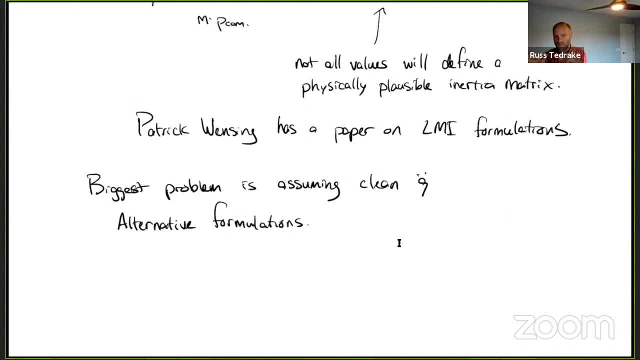 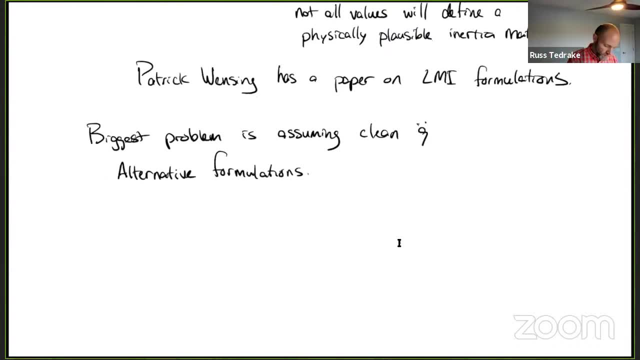 that is a way to actually, you know, you have to sort of convince yourself in the algebra that it is a removed q double dot in any effective way. but so slow teams that often tend to utilize a buffer of some sort. so what you can do is just 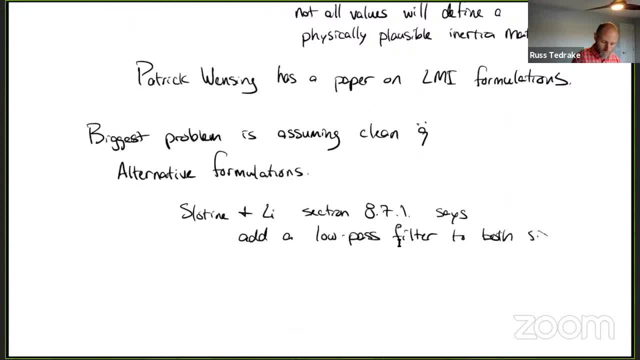 you can sort of look at these based on the above and below and you can look at your ownomi and you can. you can take a look at your ownomi and then you can look at the speed at the point that you're taking. i don't have a super fast. enough to build out, but looking at the point that you're taking, i'm going to pick good. so what we're looking for is is is a fixed set of accelerations, and getting the acceleration would be a good thing. i think it's a good thing. you're going to have to use it again. 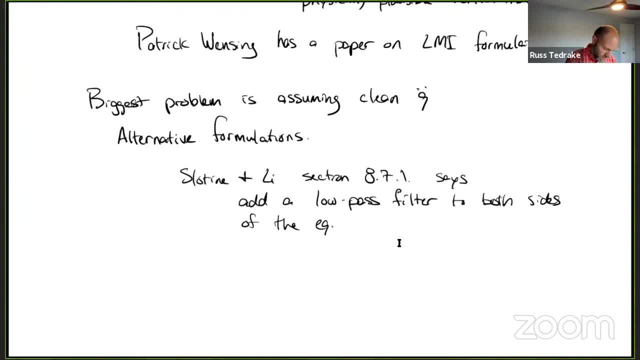 but the i think the more common solutions that you can look for are these ones that are solution to this, which Slotin also mentions, but is to switch to writing things in terms of energy and power and change of energy, instead of doing it in terms of torques and accelerations. 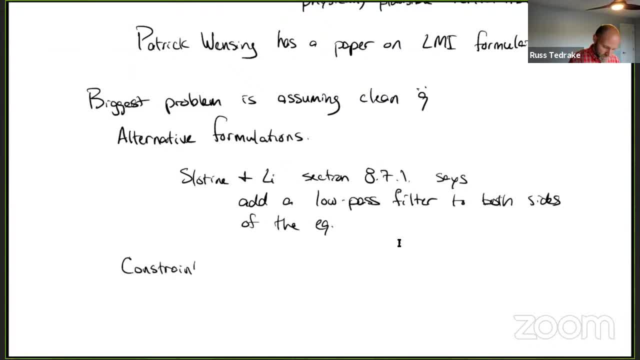 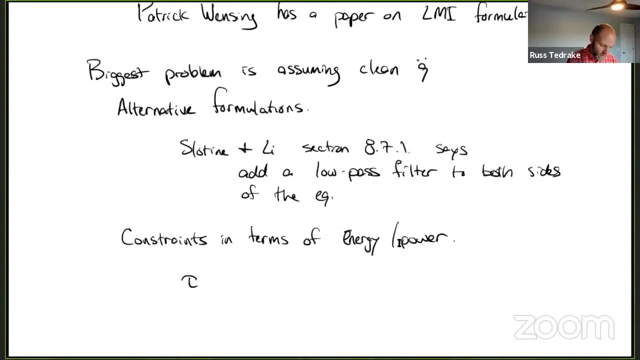 So if your constraint equations, and this is called the power formulation, if you, instead of writing, torque equals something, you can say that my torque times velocity, which is the total power, has to equal the time derivative of change in energy that you expect And in all the physical quantities we have in our equation. 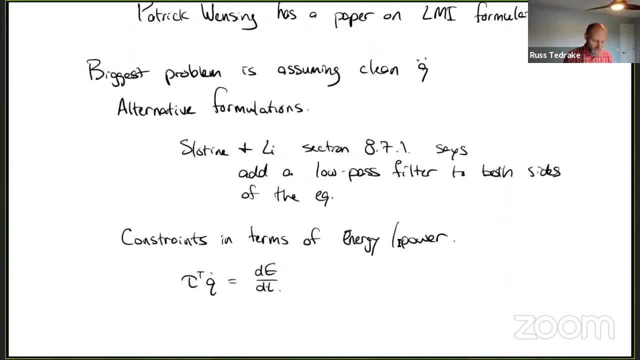 we're derived through this Lagrangian, then we can write our expected change of energy as a function of those mass parameters, And this fundamentally gets rid of q double dot. It's a different mathematical object, right? So somehow we did have n equations. 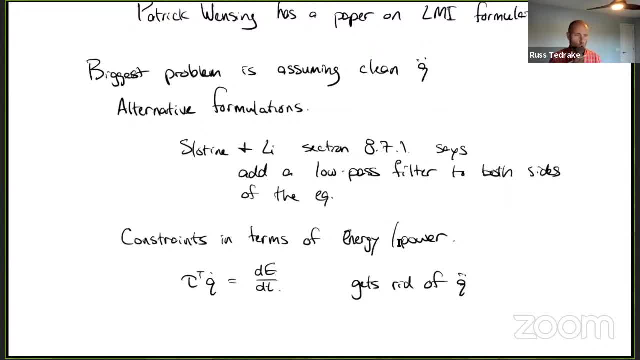 for every data point And now, if we're just checking the total power, we only have one equation for every equation Time sample. So it's a different thing to work with, but it seems that people consider it superior, mostly due to the fact that you don't need the q double dot. Mostly favor these sort 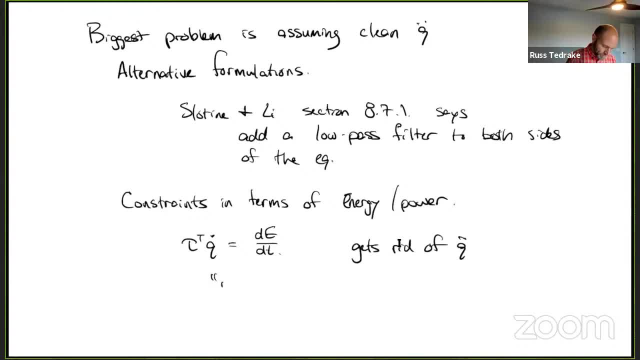 of power formulations In practice, does it change how much time you have to spend waving your object around before you can do anything with it? Yeah, I've never seen that articulated as a limitation of it. I mean, does it take n times? 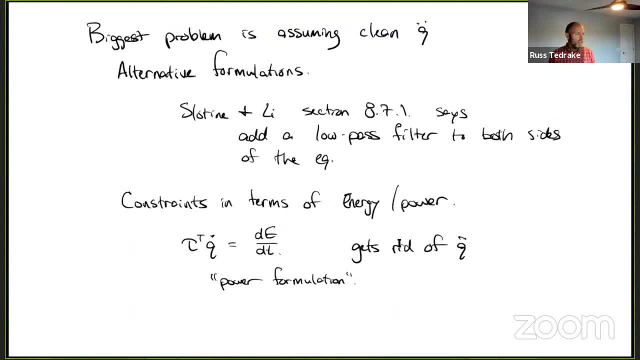 as much data? I'm not sure, Because it excites the parameters in a different way too right. So I think the time that you're spent is probably not dominated by the number of sample points, but how long it took you to get to different parts of the trajectory that turned. 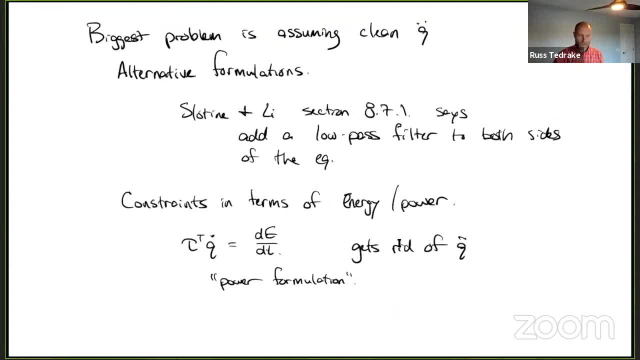 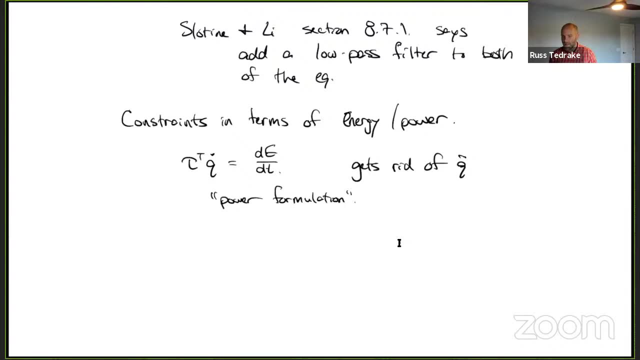 these things on And I don't, you know that excited with all of the parameters And I don't know that that's fundamentally different in this case, But it's. it is a good question. Okay, There's a like, a bunch more things to know. In fact, like, if anything, I would say: 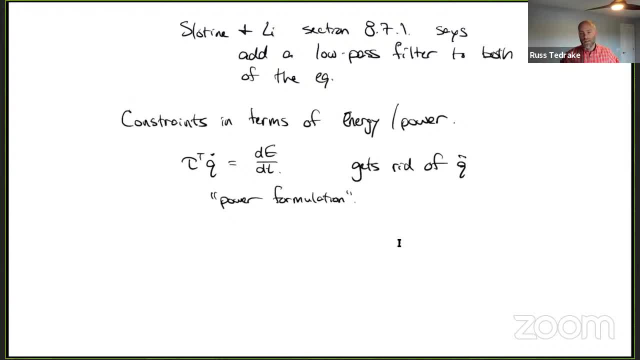 I want to give you the sense that people know a lot about this. They know, you know exactly about the. you know what sort of identifiable lump parameters happen on different robots. They know how to find them reliably. You know. they know how to find them reliably. They know how to find them. 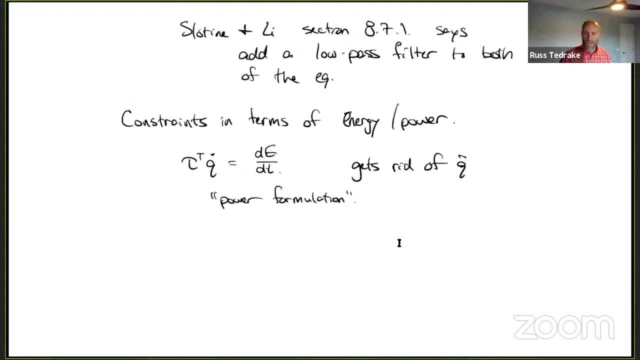 reliably. They know the numerics of these different formulations right. So I don't want us to throw all that away and learn. you know, I think we should use deep learning to learn residual networks, but probably the coordinate systems you choose matters And the you know. 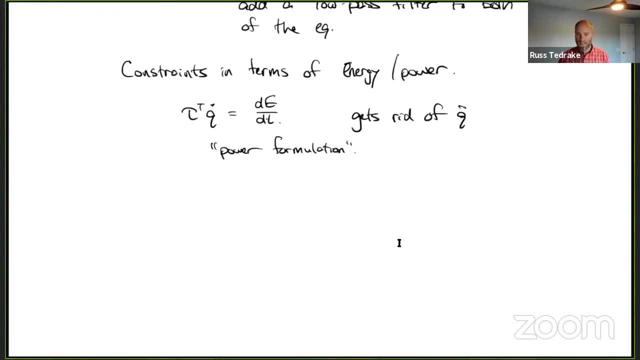 exciting trajectories is going to matter. That's a fun, that's not a some problem of our algebra. That's a that's going to be like a function of what's identifiable And the deep network's not going to do. you know what's identifiable And the deep network's not going to do you know. 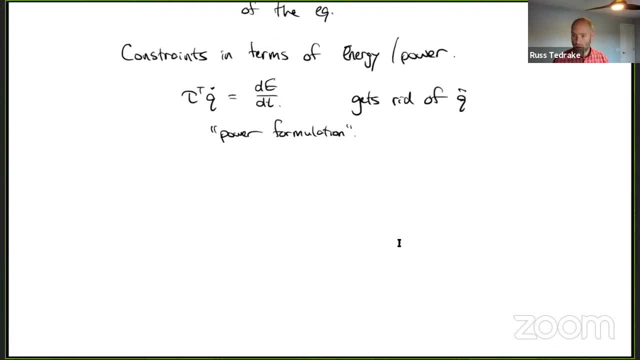 more than these methods on that. So I think there are there's a lot to know here. There's also something sort of fundamental here that I want to call out to. So the one thing that I think is a major limitation of the parameter estimation I'm talking about here. 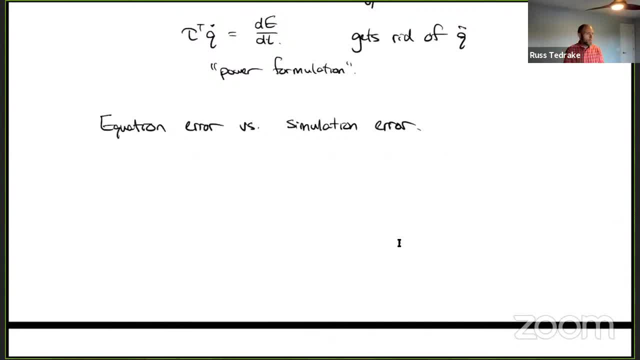 is that this is taking a view that you're you're only comparing the difference between your model and the data effectively one time, sample at a time, or at every time, sample independently, And so so that is somehow. people call that an equation or there's various different names for it, but you'll see it in all. 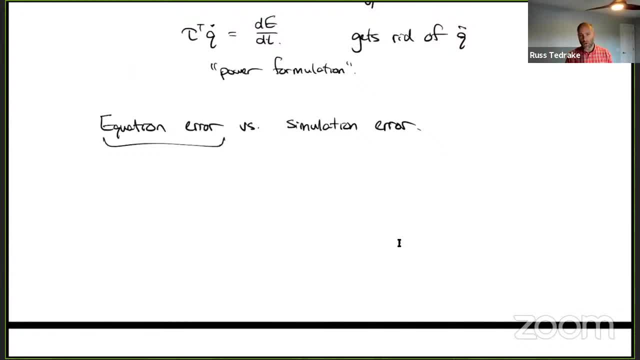 the system ID literature There's always grouped into these two different approaches. One of them is: how well does my model predict the data if, on every time step, I reset my model to the data and then do one step? I reset my model to the data, I do one step and that's what I've written down here, And that is the one that we can use least squares for. 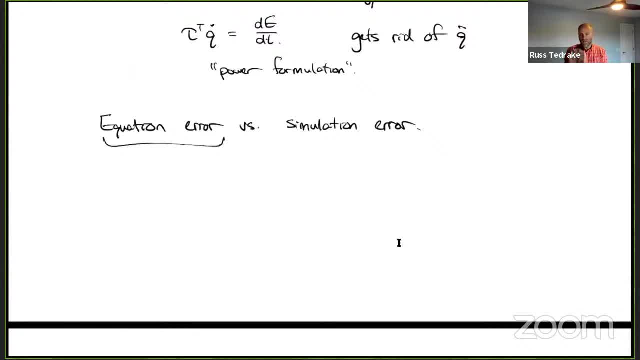 And that happens often in many of these system ID formulations is that you can have somehow a nice or a convex parameterization of the one step error, That the alternative is to say: I'm going to set up my model at some of the initial conditions at time zero and my data at time zero. 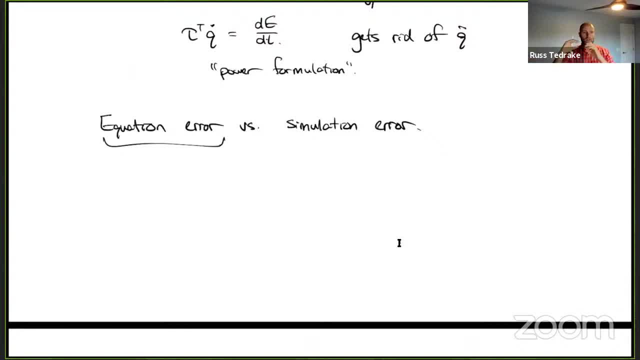 I'm going to integrate my model forward open loop and compare the integral error that has accrued right And that's called simulation error And it's generally considered to be a much more robust object. right So, but it's harder. 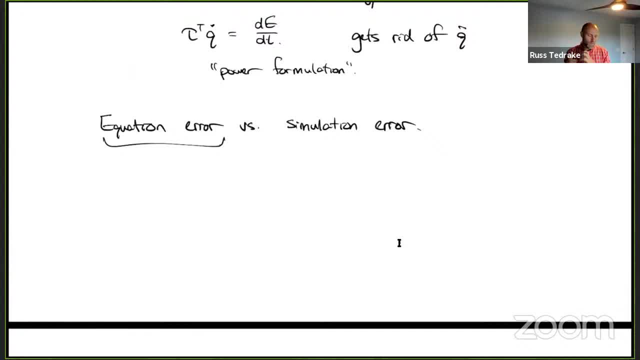 It becomes a non-convex optimization. So a lot of times what people will do will? they'll use the equation error and all this structure and math to find the initial guesses of the parameters And then they'll fine tune with a non-linear optimization. 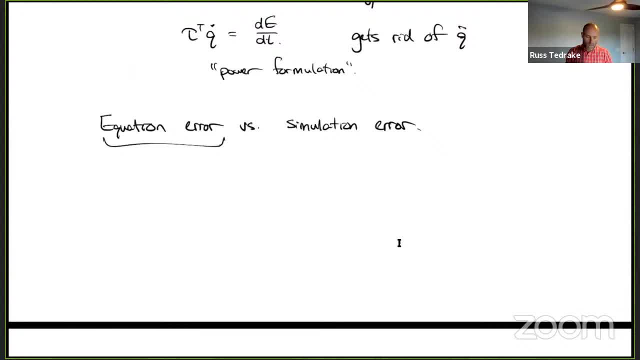 to do the simulation error. And the reason that those things are different is it is possible to describe your one-step data fairly accurately but get even an unstable like even in linear systems. people know this. You can find a linear system that describes the data. 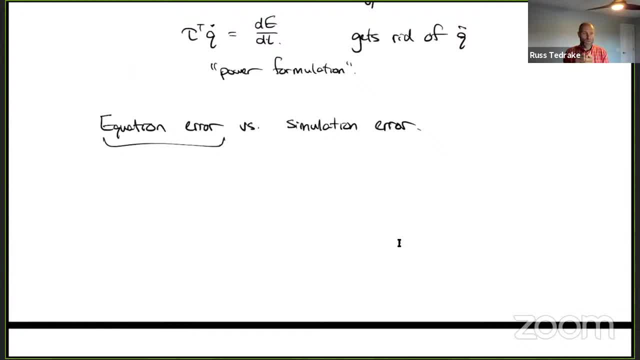 but is unstable And therefore we'll have a long-term error that is very big. So there's lots of ways around this. Some people try to do the one-step error times with some constraints to for stability of the system and all these other things. 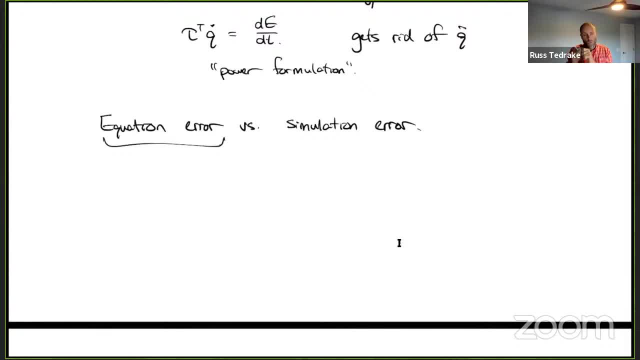 But I just want to call out that everything I've said so far today is this sort of one-step view of system identification, And there is a potentially more robust thing to do where you just simulate it forward in time. Okay, so if your robot only has position, 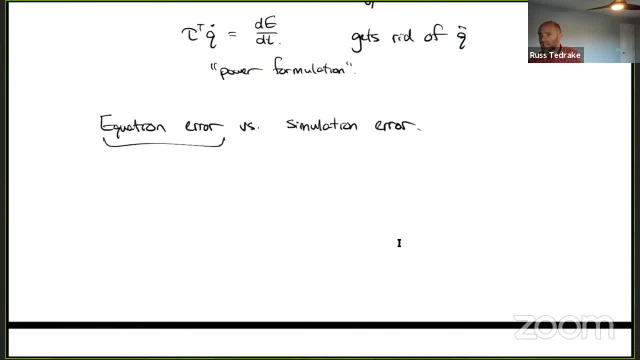 plus torque force tensing. can you simply pick a bunch of static positions and estimate the parameters in a similar way? Tell me what you mean, Sebastian. I don't quite get it. Yeah, so instead of prescribing or measuring the speeds and accelerations, 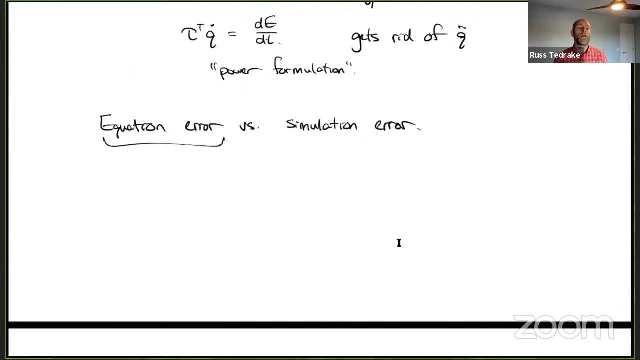 if you just move your robot to a bunch of static positions and just compare what the gravity torque to hold up the arm itself, plus whatever it is when you're holding the object and grasp, and just getting a bunch of those different positions and formulating similarly squares. 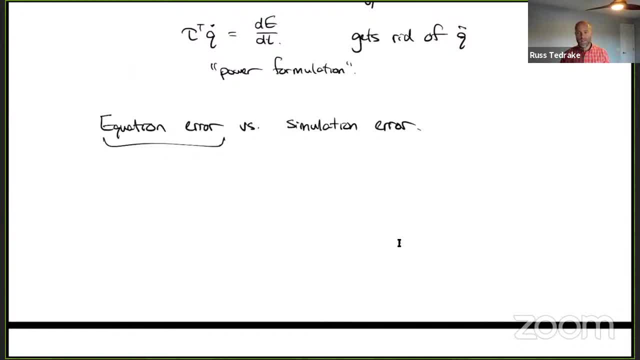 Cool, Yeah, yeah. So I think the way you said it is perfect and that you can tell there's going to be some limitations to that, So you can get all your statics from that, but you can't get your dynamic terms right. 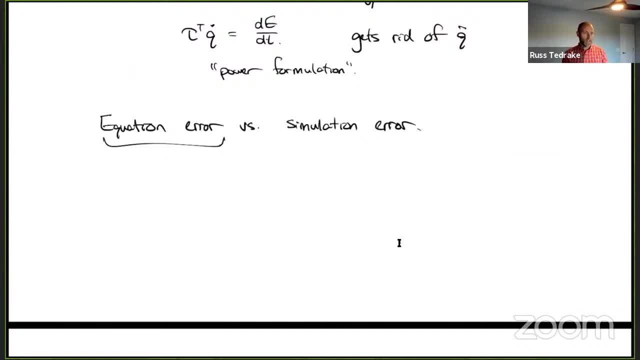 So all the velocity dependent terms would be hard to get that way. Joint damping and stuff like this would be hard to get that way. But certainly you can estimate inertia matrices that way. But if you're just estimating like mass and inertia of your ingrass object, that's fine, then right. 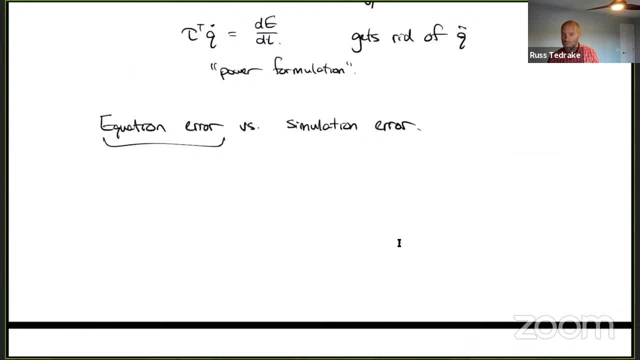 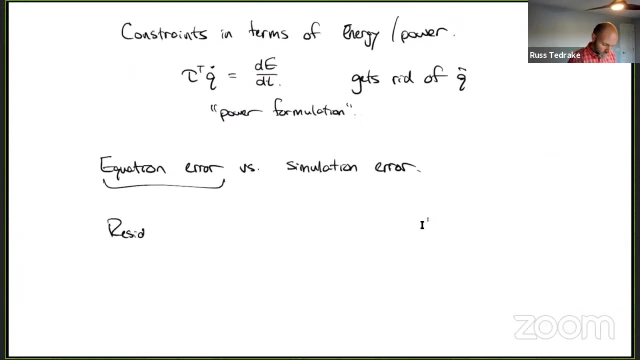 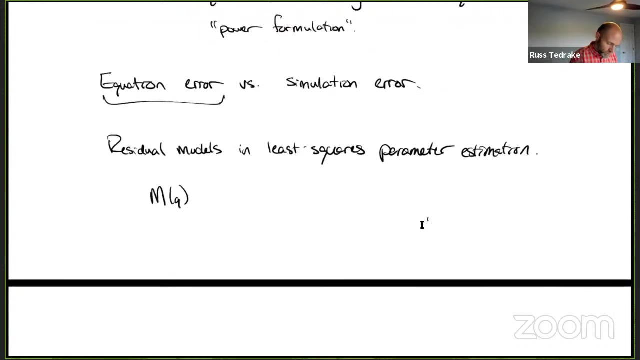 I think you're right. yes, Yeah, perfect, Thank you. Okay, So people also write in residual models in this sort of least squares parameter estimation framework, And it won't surprise you really, but you'll put a term like this in. 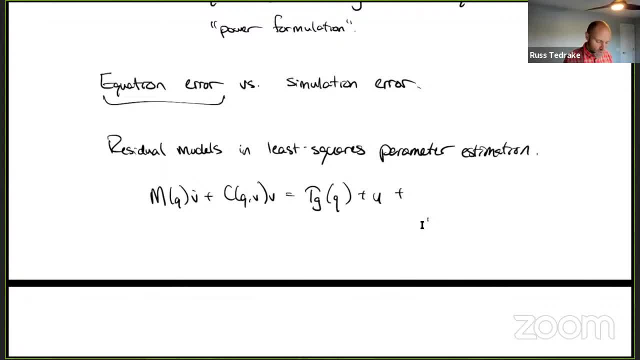 and then you'll put in some huge, potentially huge set of parameters- times, some nonlinear basis functions, right, You could have it on potentially all of the terms. okay? So some nonlinear basis functions with linear parameters And the power of doing that. 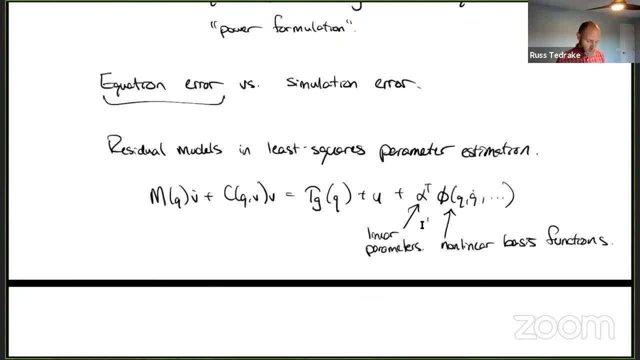 I mean, the alternative would be to put a deep network here. You can do that, But then you're in the space of doing gradient descent And in this case you can still do least squares, And these nonlinear basis functions can be surprisingly rich. 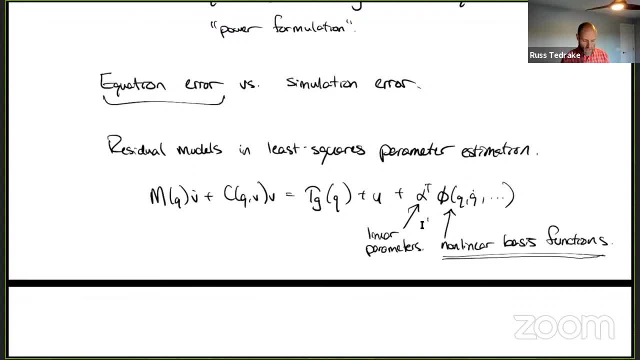 So there's a lot of work from Jean-Jacques Slotin and others of using, for instance, radial basis functions for this, using the wavelets like I showed for the airplane catching And I don't know. I think it's extremely interesting to ask. 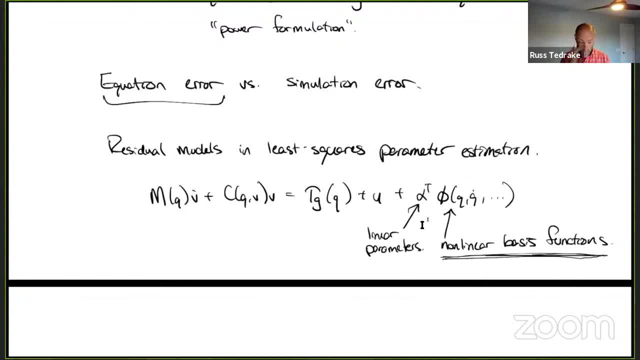 how much we've gotten. what is the gap If we were to put all of our best tools like this at the tossing problem, for instance? I do think that the representational power of the deep networks is going to be stronger. So I think this case. 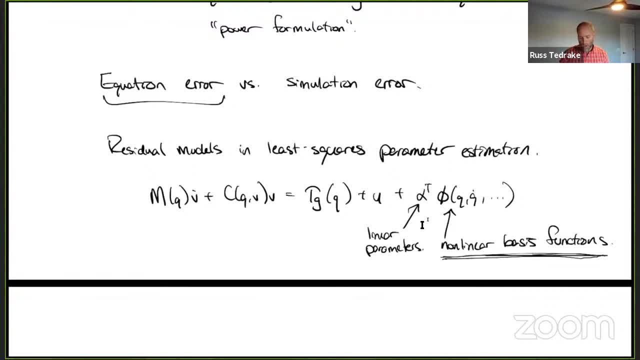 so I think in the Andy Zhang version. from experience I can learn some parameters of my throwing, so I don't have to do any online identification. In this case I could pick up any object I haven't seen before. no learning required. 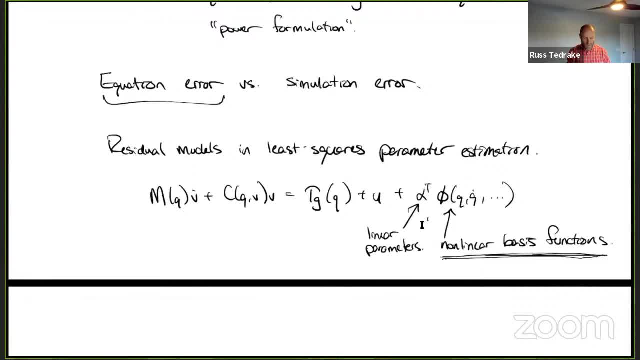 and do a little estimation and then throw. So there are slightly different things, But I would love to put them head to head and really understand what the best version of this could do compared to the best version of this. So I think that's a great question. 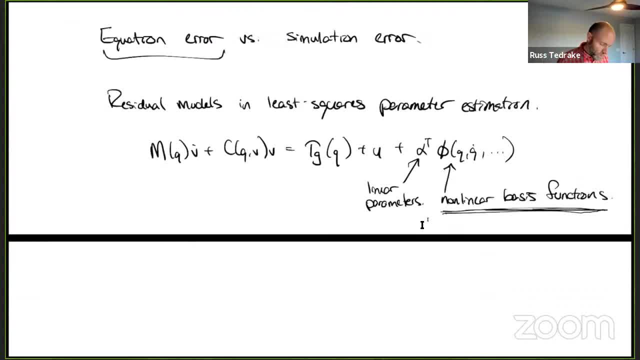 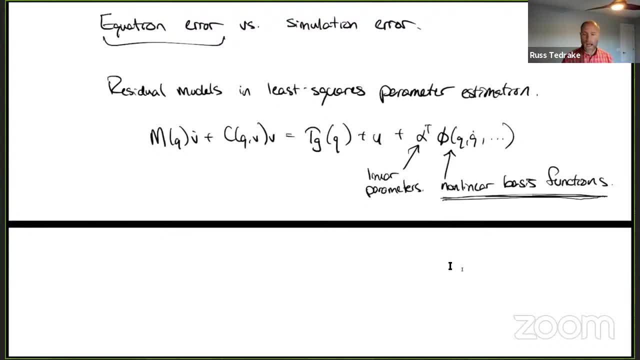 I think that's a great question. I think that's a great version of the learning solution that Andy did. Okay, Let me just give a bit of a teaser for how this plays into some of the better results in adaptive control. Really, it's like you know. 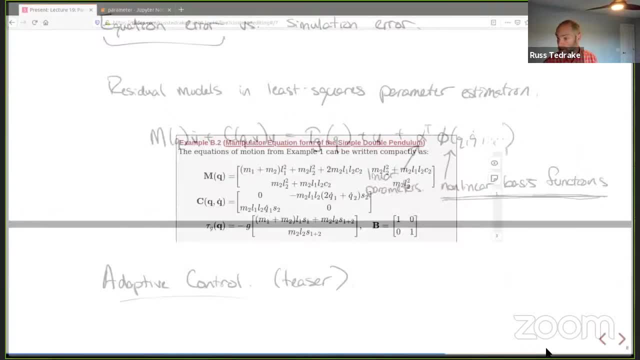 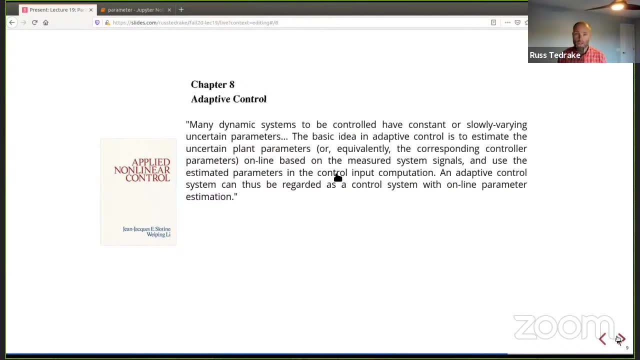 go take the course if you're interested, because it's really a good topic. Okay, so John Jock wrote a great, influential book. I thought the chapter introduction was as well as I could possibly have said it. So for constant or slowly varying, uncertain parameters. 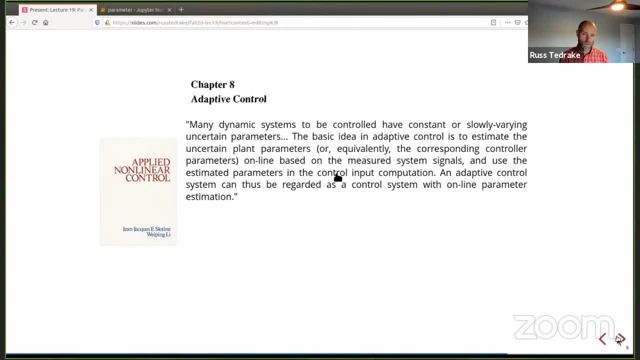 we're going to estimate the uncertain plant parameters or the control parameters online based on the measured signals. And basically, adaptive control system is a control system with online parameters. So we're going to estimate the control parameters based on parameter estimation, right? So what is a parameter versus what is a state variable? 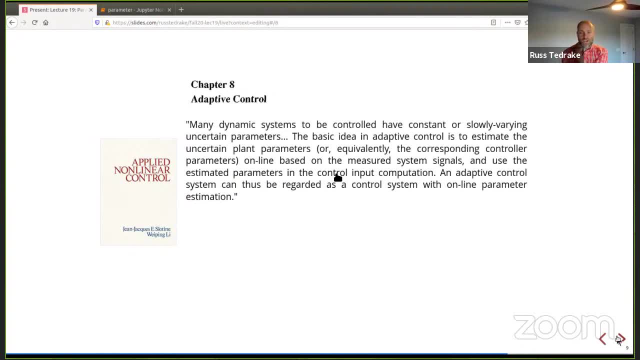 You know, you could argue it depends on time constants. but if something's changing slowly relative to the dynamics, then you call it a parameter and you maybe use different approaches to try to prove, to try to estimate those parameters online and converge to it. 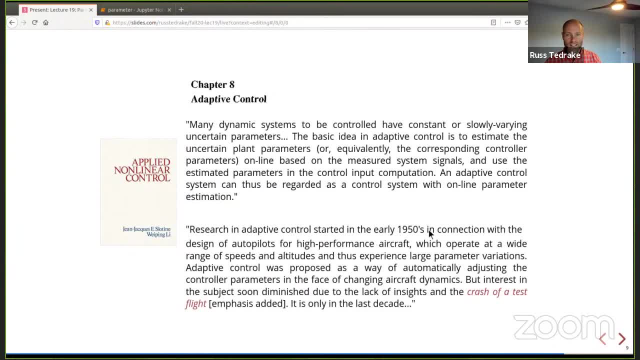 And it was interesting to see again in the history lesson in John Jock's notes. you know he says in the 50s it was super popular. but then there was that crash flight. There was a crash of the flight. 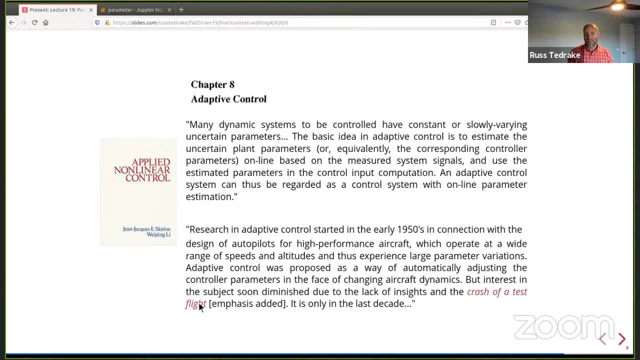 that sort of nipped it in the bud And then there were some theoretical results that led to his work in which was in the last decade, in 1991 or whatever. So you know it's an interesting history, but it really has a lot of similarity. 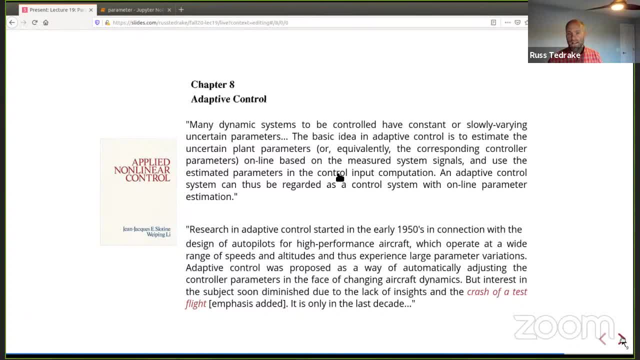 I mean, it is the reinforcement learning problem, if you will. in a lot of cases They have direct adaptive control, which is policy search, indirect adaptability, adaptive control, which is fit the parameters of your model and then use it in a controller. 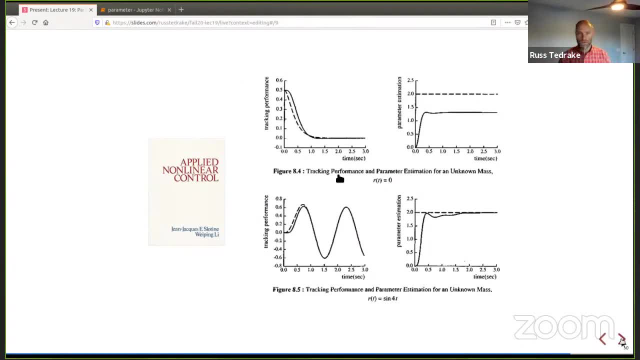 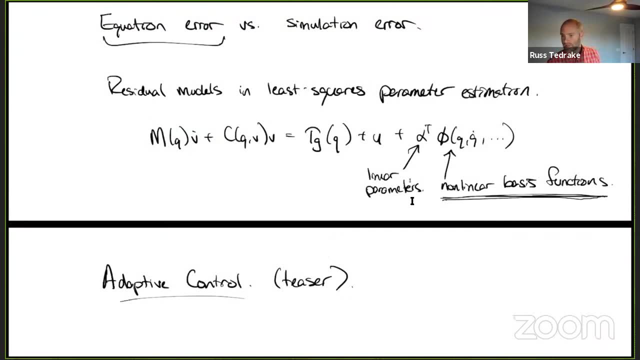 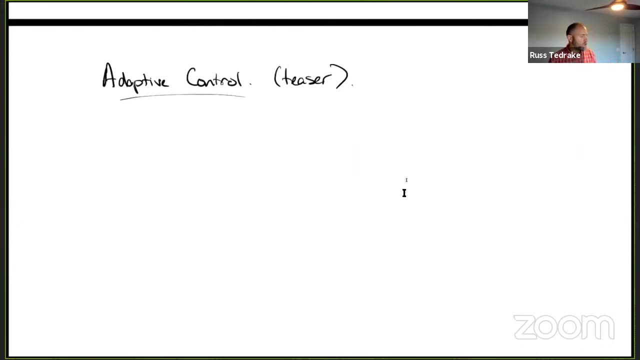 All the model-free versus model-based stuff. it's all in the adaptive control literature too. Okay, so let me give you some of the simplest examples. Okay, so there's, I think, the most important thing I mean. so adaptive control is doing the estimator. 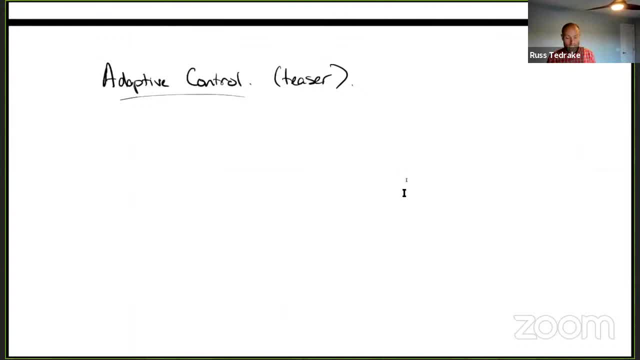 I just talked about the least squares estimator, for instance, but doing it online so you can write recursive forms of the least squares estimator, which are so you don't have to like just every time you get a new data point. 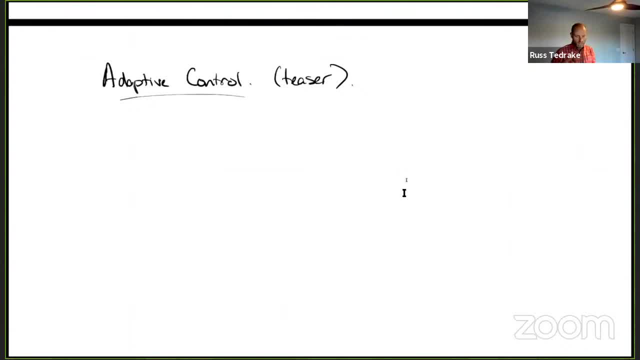 recompute your entire least squares, you have a least squares estimate that can be updated incrementally. They typically look like a small linear filter, but the equations are simple. How do you take that online linear estimate of the parameters and estimate the actual parameters? 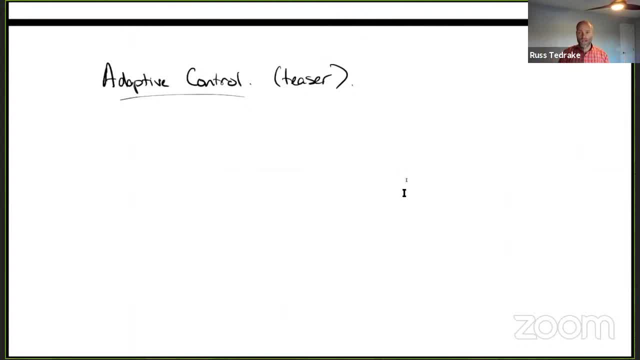 in while your controller is doing something and still prove that the system will do the right thing, Despite the fact that you're mucking with the parameters of the plant, as you're doing the control right. And it's a super interesting topic, I would say the one key idea of model reference, 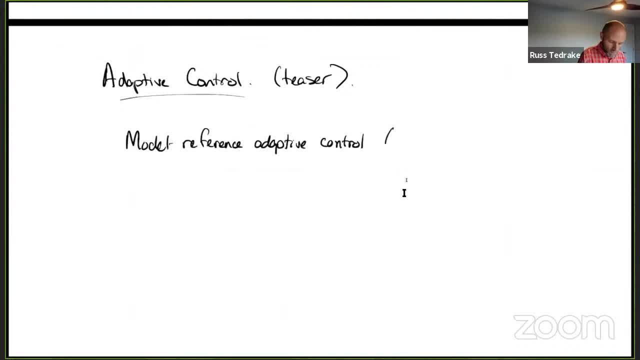 adaptive control MRAC versus the online- just online- parameter estimation, which the adaptive control world does too. but is that you know? in this case, in the MRAC case, the objective is not explicitly to estimate the parameters. 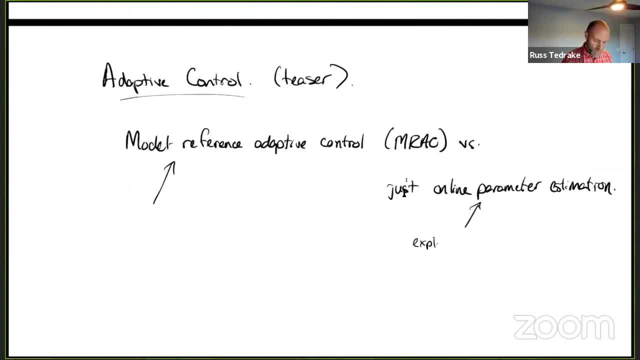 So so there's one form where you explicitly estimate parameters as well as you can And then use them in control. The formulation in MRAC and in a lot of adaptive control is just regulated. you know track a trajectory perfectly if you will and estimate the parameters as necessary. 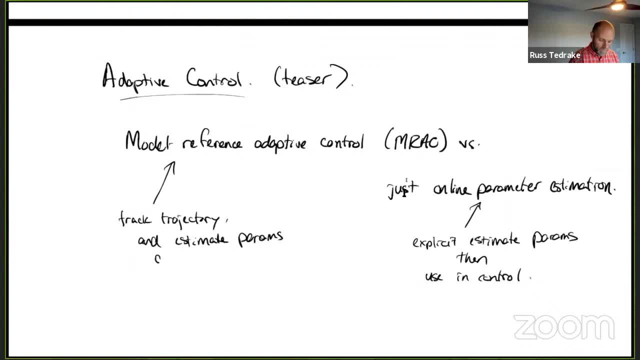 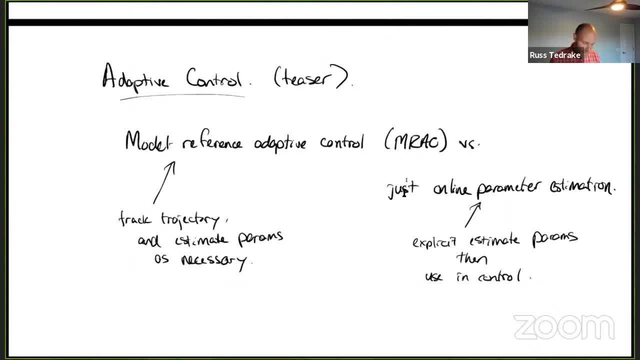 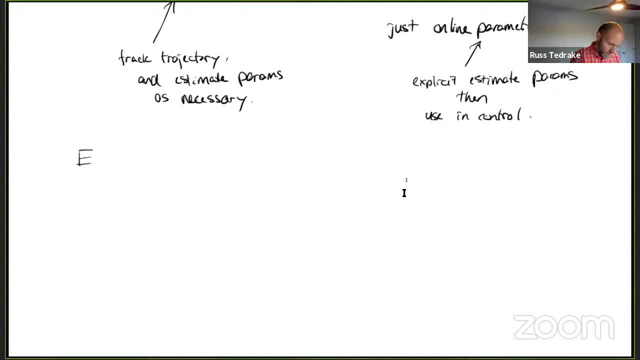 It's just a goal of tracking a trajectory, Okay, And I can give you sort of the simplest example of how those might be different. So if you think about a double integrator, which would just be MQ, double dot equals U, Okay. 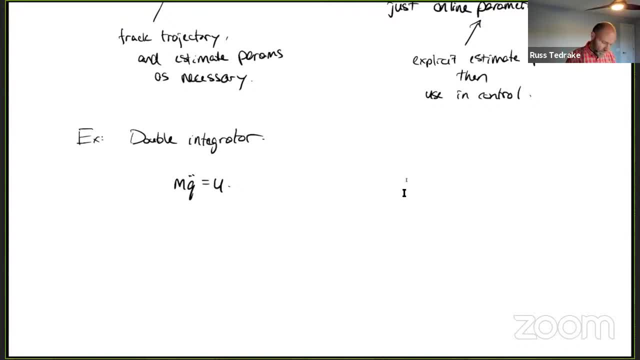 If I want to estimate the mass parameter. the parameter estimation might do something like M hat is U over Q. double dot could be close to zero. all these other things right. So what we we're advocating for instead is least square solution. traders, leash square solution. 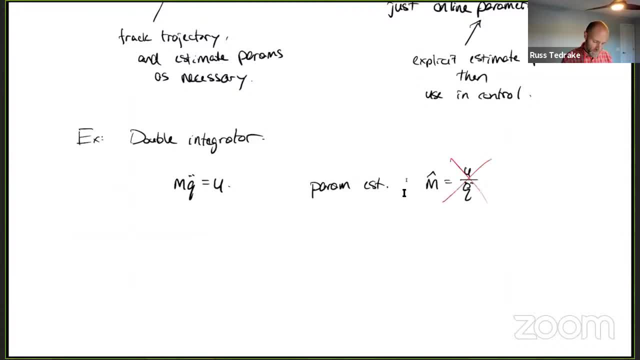 right, missing M, right. So that's a good use case. if anyone has a reading pointer, then F and you've got a couple ofgu levels. all of us will be right back in the�� and I'll natomiast them all. 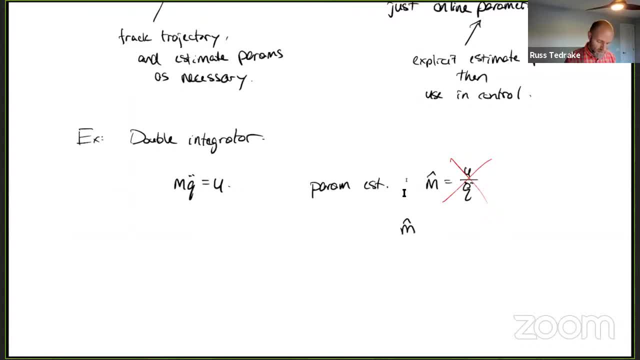 Very, very painterly. There're less than two degrees degrees on the new it. this stretch, Okay, All right, n over m over some entire trajectory, But I can explicitly write an estimator that tries to minimize m And, like I said, there's online versions of this. 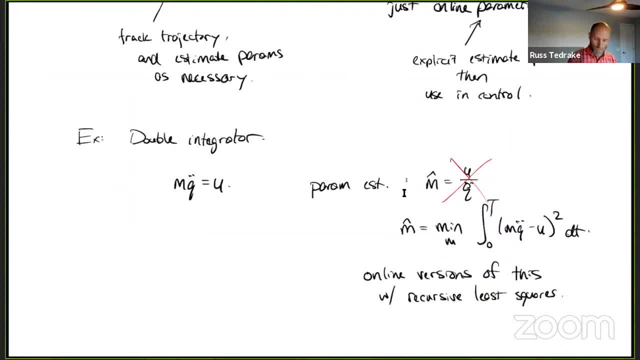 And when you're all done, you'll get the mass out. If you've written a sufficiently rich trajectory, that is, an algorithm that's running the explicit goal of minimizing some prediction error- The MRAC equivalent- you could write a controller that will track a trajectory of q double dot. 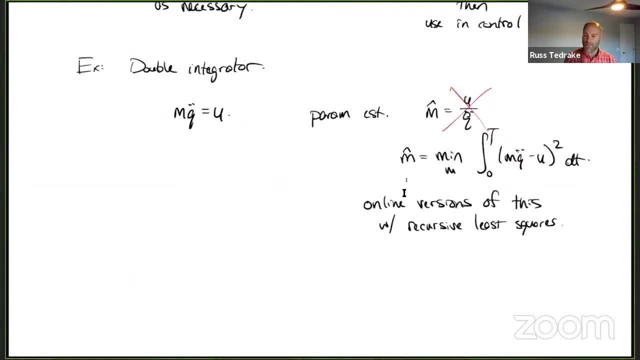 a desired trajectory And it may estimate the mass if it needs to. There are other cases where it doesn't. It doesn't need to estimate the mass And it can still regulate the trajectory. It just depends on what the desired trajectory is. 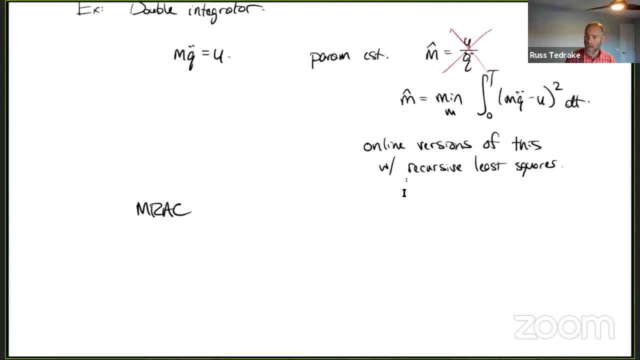 So the MRAC version would try to impose some second order dynamical system. OK, so let me just give you the basic form of it. I'm trying to see if I can skip some of the basic things. I can't see the jargon. 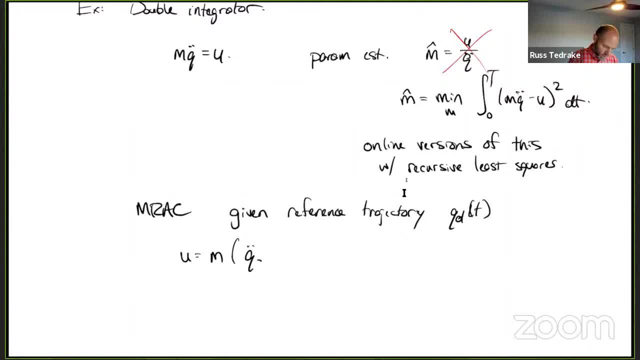 So if I were to write a controller, if I have a reference trajectory, you could write a controller if you had the model that would follow it, which you might write as something like q double dot m, You'd have q double dot desired, minus some feedback term. 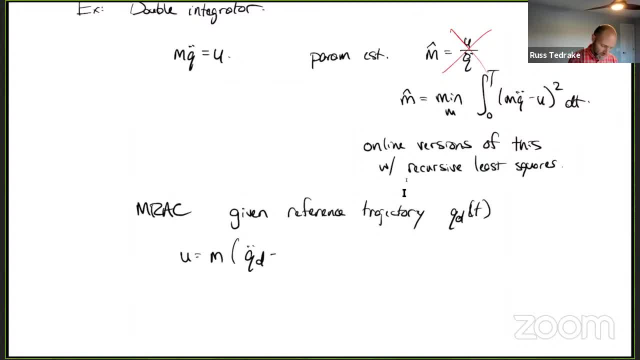 So this would make q double equal q double dot desired already. But if I have to reject any initial condition- error or noise or anything like this- I'll add some PD terms in here. Instead of writing the full PD controller, I'll write a critically damped one. 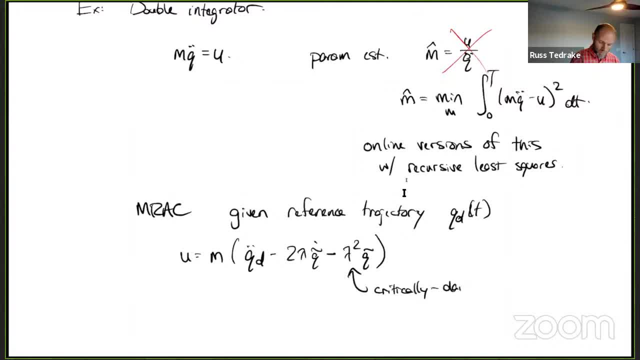 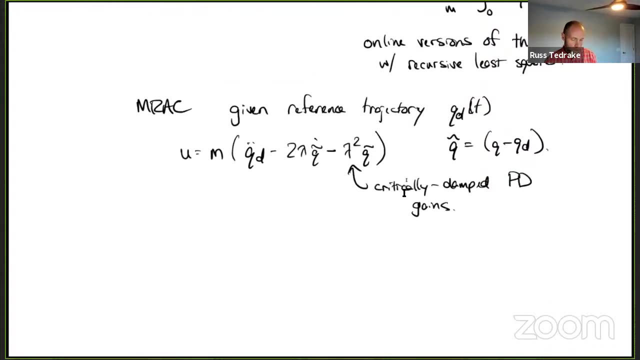 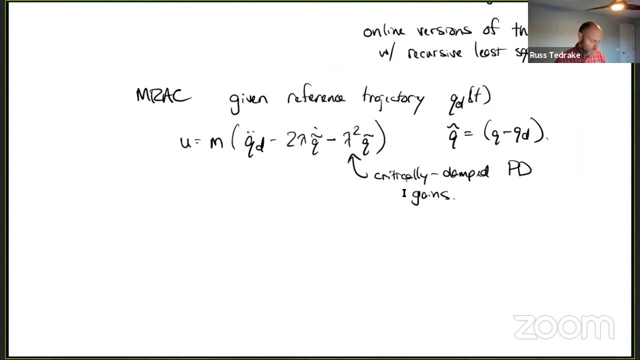 where q tilde is just q minus q desired. okay, it turns out. if you examine the performance of a controller like this, then you can write a much simpler um control law- that up there update law for m, which has the explicit goal of proving that the trajectory will converge and it has only a sort 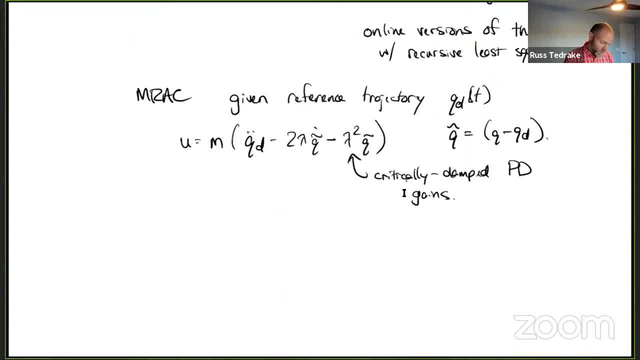 of a secondary goal of estimating m. so in practice the controller will look something like this: you'll write on control law which adapts. the form is going to look a little bizarre if i but you don't want to see all the sliding mode stuff that normally goes along with it. um, 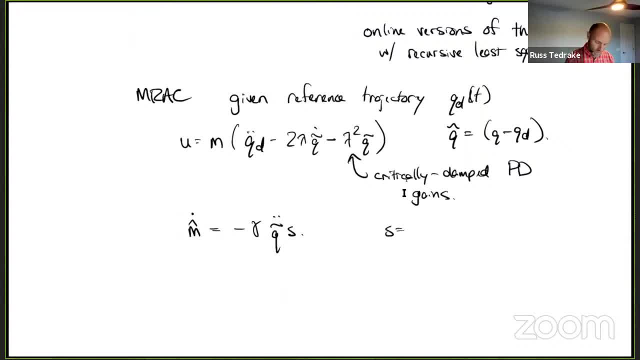 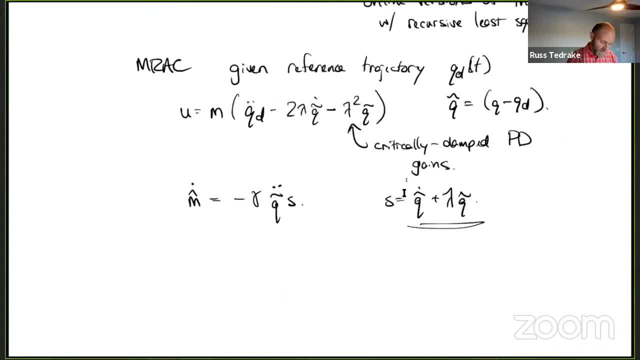 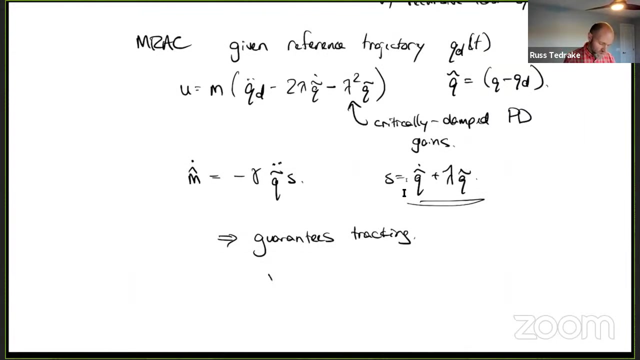 okay, but this gives us the guarantee in terms of you know, so it guarantees tracking. so this is what people do in the full robot case, to and all. but i just i think it's sort of easy to think about in the very simple case, because in this case there's a function like a cost to go function. so the optimal function that people will write, which is actually going downhill the error that you want, it has an incidental, an incidental term. 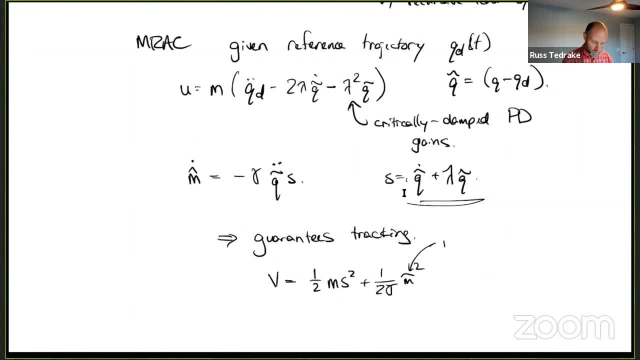 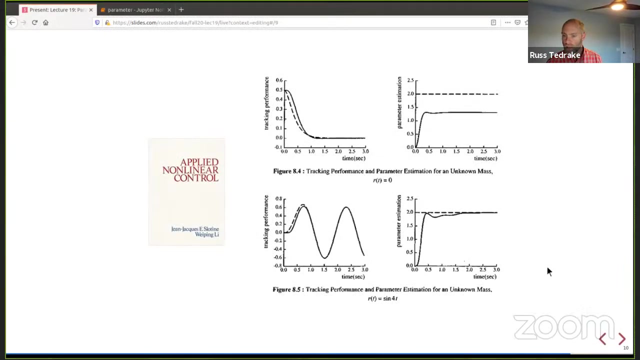 of trying to estimate the, the um math my uses and Baum or be is the error In your estimate, okay, And you can show that this goes downhill whenever. Whenever s is non zero, Okay. So the big point is that. 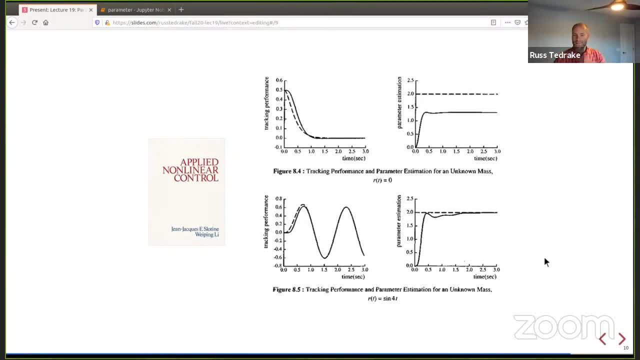 In code. big point there is that you can rate controllers, which will accomplish the task. but I'm ready for this To submit control Last or we'll see where data gets lost Next. So, but not necessarily, have to estimate the parameters. 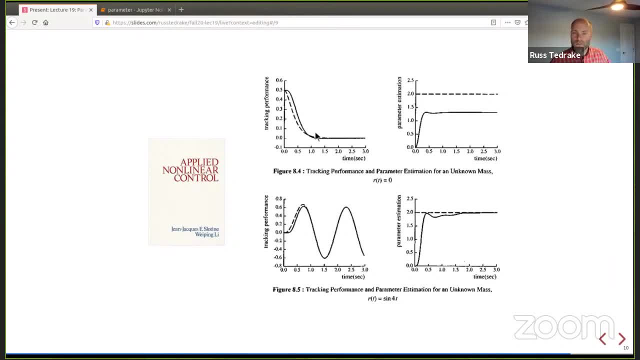 And the example from the book, which I think is quite nice, is even for this double integrator example. if you give it a reference trajectory which is just trying to drive it to zero, in fact it can converge quickly enough on that reference trajectory. 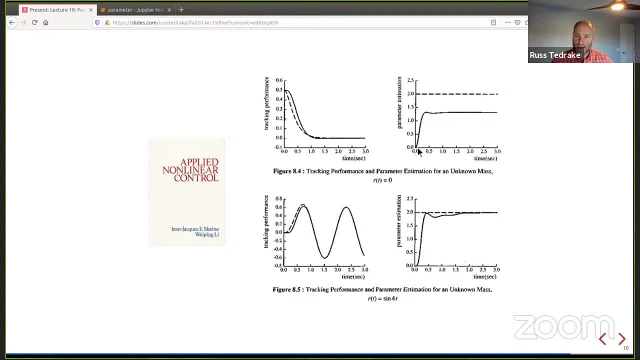 that even though it starts with an unknown mass- this is the parameter m hat estimation- it drives m up in order to try to converge, but at some point it's actually accelerating close well enough towards the origin that it's absolutely fine tracking. 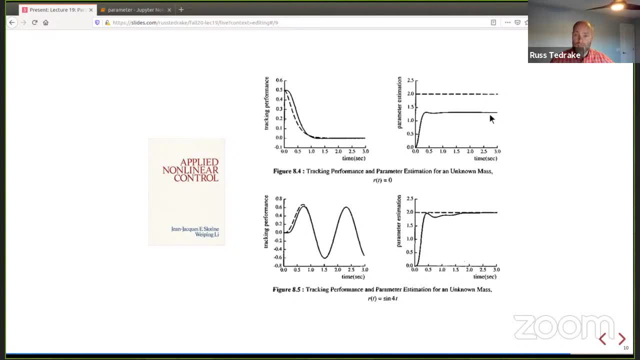 with m being the wrong value, it's still tracking the trajectory perfectly and it will never converge to the real solution. If you give a different trajectory, though that's trying to execute a more interesting trajectory, then it will actually in order to get the long-term steady state to zero. 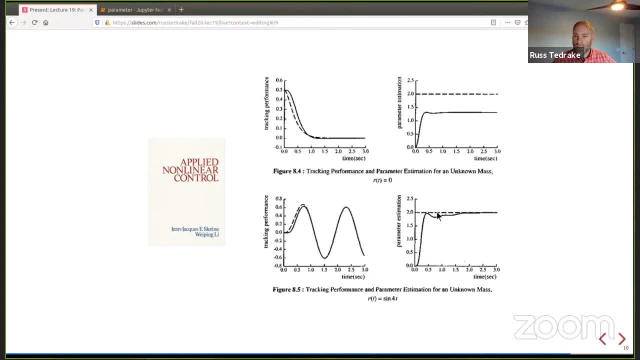 then it will drive the mass to zero. Now, this is a little bit like the topics that come up in reinforcement learning, about how you don't need to learn your model. I mean when people argue about model-free versus model-based. one of the advantages of model-free is: 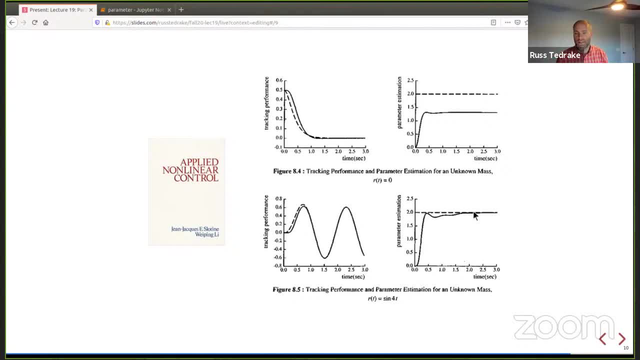 there might be things about your model that you don't need to do is accomplish the task. I talk to, I say that when you're, I say I'm buttoning my shirt and I don't wanna have to estimate the state of my shirt. 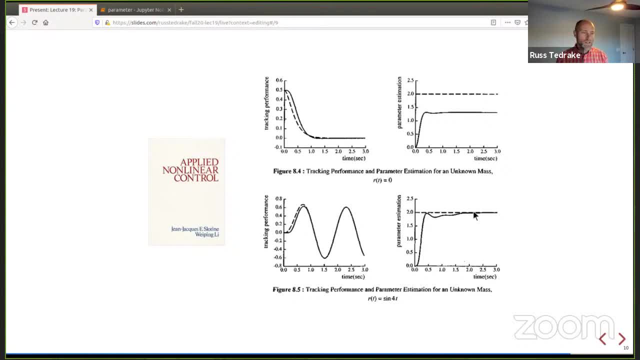 or the model of my shirt, right. So adaptive control can have that flavor also right. It can estimate just what it needs to accomplish the task And in fact the controller that we saw sort of for the for Jean-Jacques, you know. 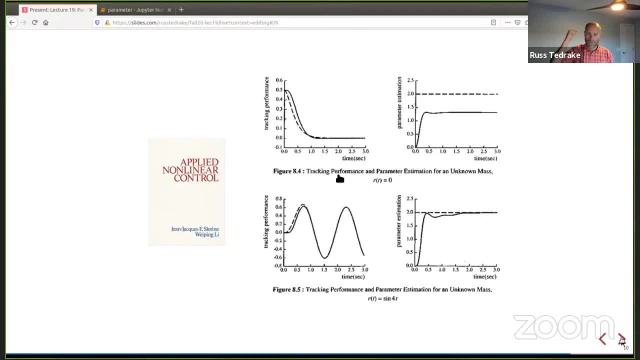 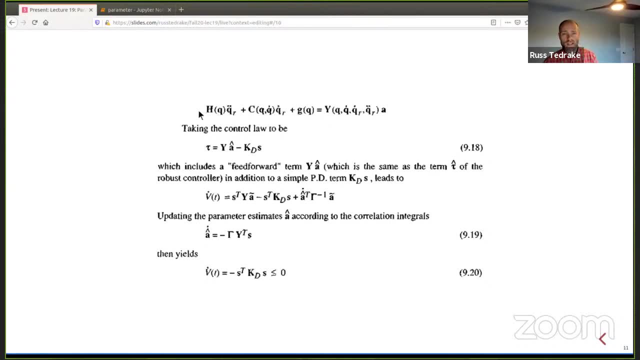 throwing the ball. I can assume he didn't. they didn't publish that version, but the paper catching and the like they were. this, the multi-body version of that, where it's almost exactly the same. He uses M instead of C or, sorry, H instead of M for this. 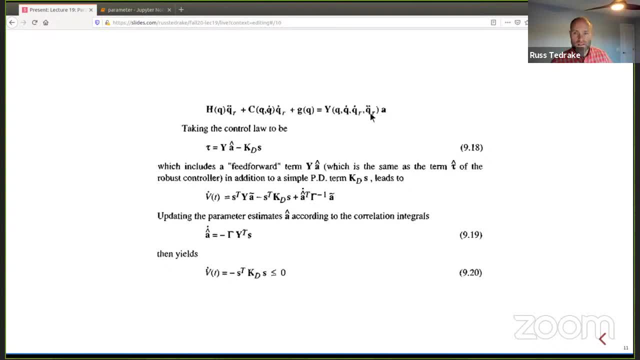 But, and gravity is G, but it's almost exactly the same. He's got his data matrix times his parameters. He adds a PD term on PD on top of a model, a forward model, And you get these terms. you get a Lyapunov argument of the form like this: 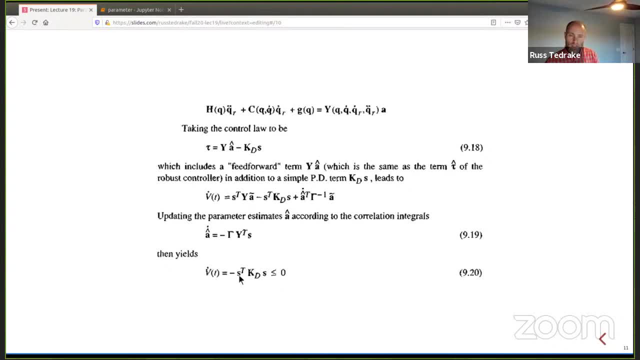 So what this means to me when I look at this is that I have a guarantee that the error metric- my error metric first of all- is a combination of my parameter error and my tracking error, but it only goes downhill when there is tracking error. okay. 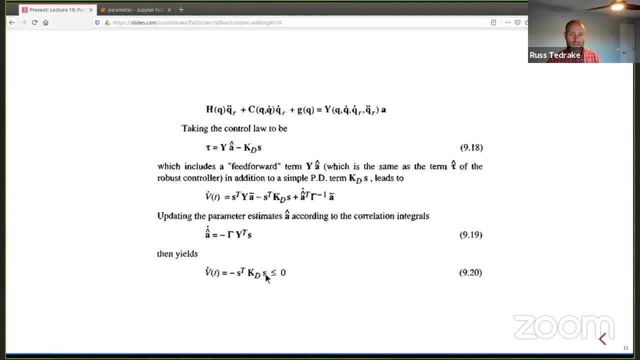 Because S is my tracking error. It's like the error going into my PD gains And I'm only going to try to fight that error. The guarantee I have is that my tracking error will go down, but it never actually tries to estimate the parameters. 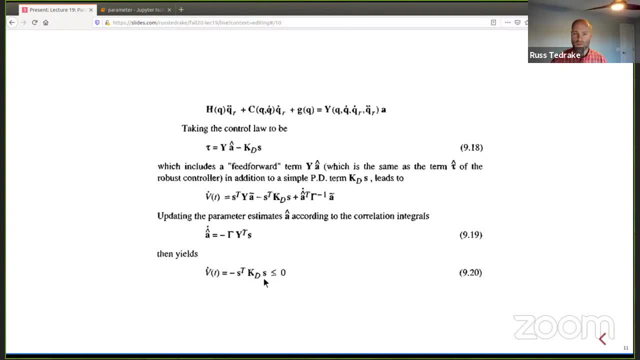 It will leave residual in the parameters as necessary when tracking the controller. Okay, so there's a lot to know in adaptive control. I think the structure of the equations is so rich that it just doesn't let's see. I feel torn because I think for really interesting manipulation tasks. 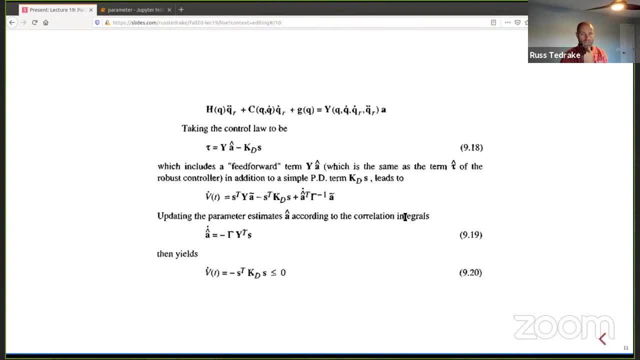 it's not clear that you should try to, should start with physics models and fit the parameters. But for something like tossing bananas, I guess I think you should. I think you probably just can pick that up, think of it as a rigid body, all the objects in that. 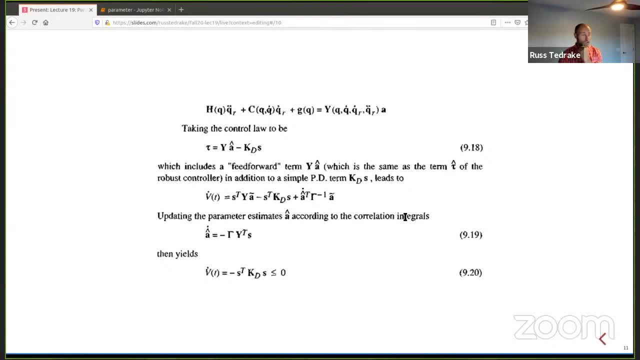 are rigid, You can estimate its center of mass, You can design a better trajectory for your robot to execute that and leave with the proper velocity. And I think that the dominant effect of the residual learning, at least in that example, was more about just being 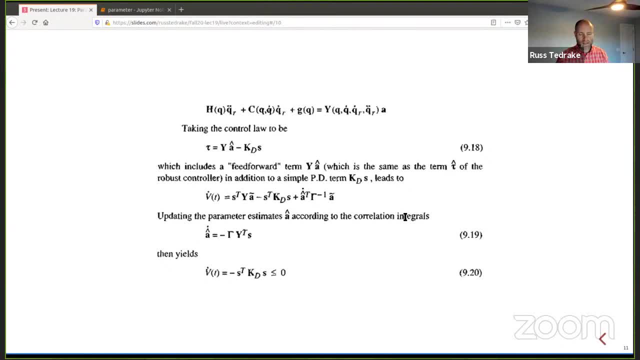 the physics model was too sloppy about where the center of mass was relative to the hand, And we could have done a better job with that. Any other questions about that? So just on a so this one where we don't have to estimate the parameters. 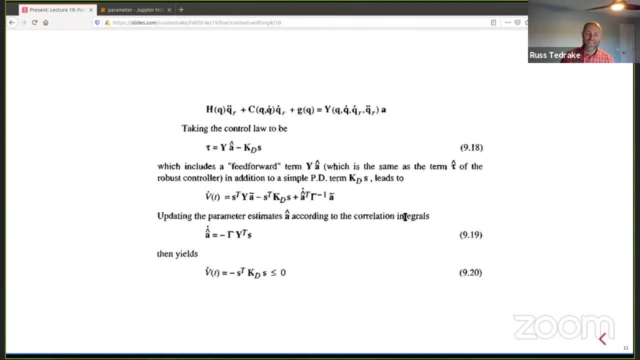 is called indirect right, Wanted to clarify terminology. So good, So they're slightly different. So model reference adaptive control is this one Sort of- I think John-Jacques would call it. the self-tuning controllers would be the other class. 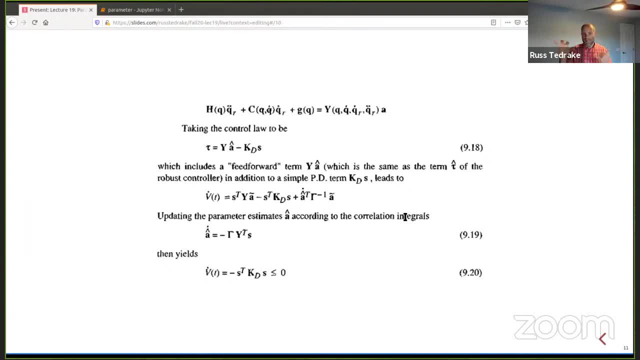 where you're trying to estimate the parameters explicitly And then under self-tuning you would break into either direct adaptive or indirect adaptive, where the direct adaptive would estimate more of the control parameters directly and indirect goes through the plant parameters explicitly. So normally, 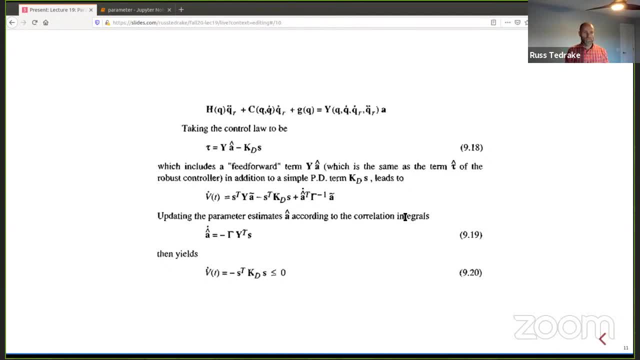 indirect means: estimate the plant parameters and then use it in your controller. That's the shorter answer, And this one is not that. This is design the update for your parameters in order to be able to write a proof that your system's gonna converge. 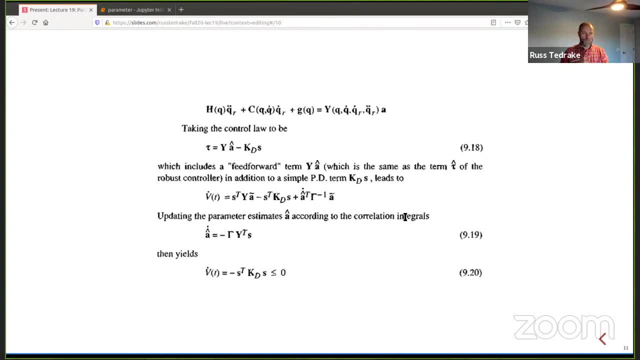 And it's not that your trajectory is gonna converge, right. So these things are typically motivated by giving some algebra that guarantees that my system's gonna converge, And they don't explicitly run through estimating the model parameters. But I thought direct adaptive control doesn't estimate the model parameters either. 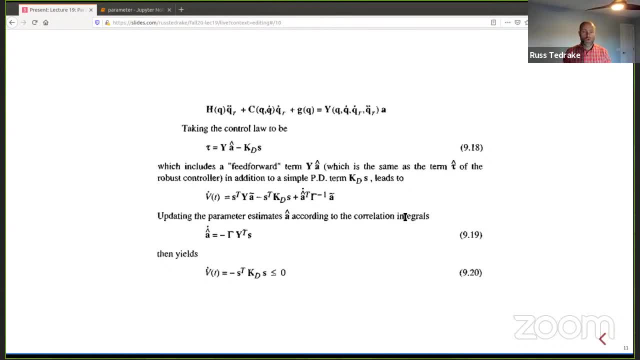 So would it just fall under direct? So yeah, I mean there are ways to write an explicit self-tuning controller parametrized the control parameters instead of by the plant parameters, which I think it's completely fine to think of that as a direct. I think people would distinguish between this and a direct method. 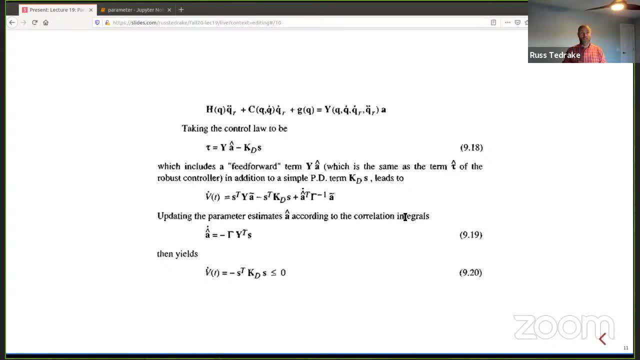 Model reference. adaptive is a slightly different thing, But in broad strokes I would say this is closer to direct than indirect. yes, What do people think? Does it make you think that you should study the robot? Is it the older robot texts? or does it make you think that? 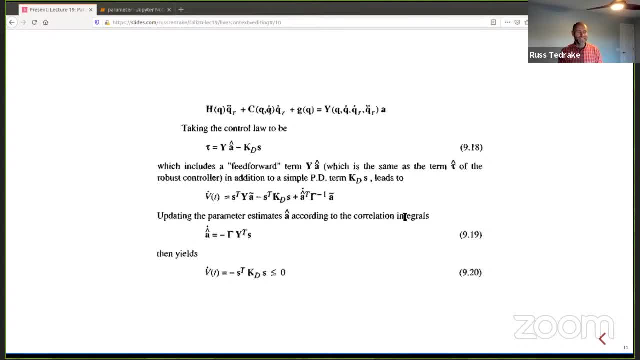 we have reinforcement learning now, so we don't need this stuff. I honestly wonder. I don't know what the right answer is, but I think this should be in your arsenal if you want. Yes, I think reinforcement learning is incredibly general and powerful. 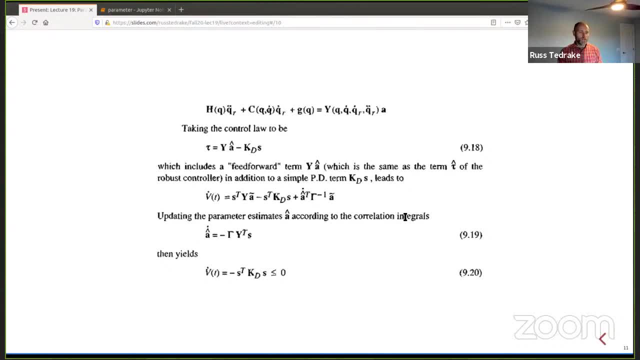 but extremely inefficient, So you should only use it when you don't have more structure, And I think that's a good point. I think that's a good point. I think reinforcement learning is incredibly general and powerful, but extremely inefficient, So you should only use it when you don't have more structure. 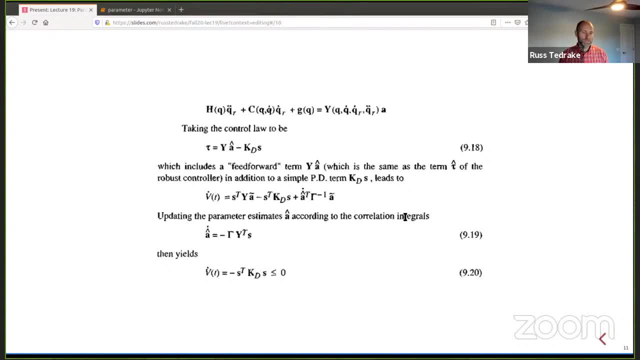 And this is a case where we have lots of structure, basically, Well, it's okay, Oh sorry, Oh no, you can go. Terry, I'm just trying to understand the logic for why you want to do residual learning And 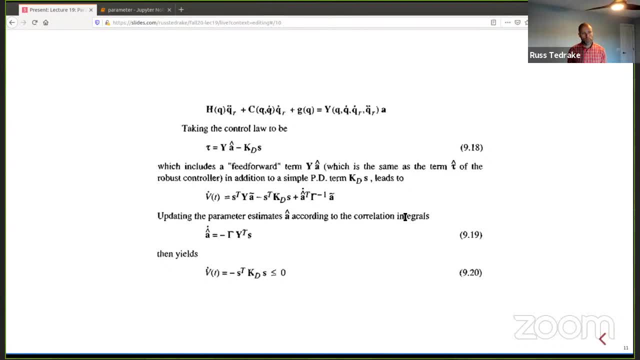 could it be that when you do online gradient descent to find the parameters, the physics model acts as a baseline, a sort of connection? Oh yeah, totally. I think Andy makes that point super well in the paper, Even in the video I think it says that the physics model helps to generalize to different. 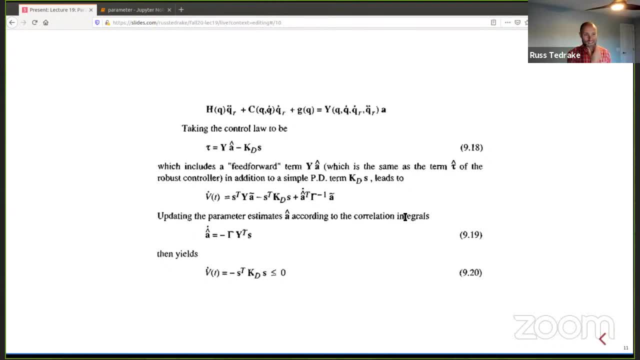 Cartesian things very well And then really just adding something on top of that could capture, for instance, aerodynamic effects and errors. in that, I think the motivation is: use as much physics as you can, hope for the generalization of power of physics and then do a little bit more to capture the slop. And I think there has been a cultural 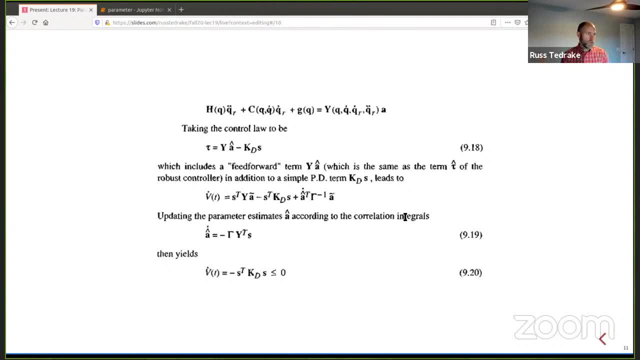 change where we used to think that the equations of motion gave us almost everything. and you really are capturing slop terms And I think now we're willing to say: oh well, that's not going to say that the equations of motion are doing very little and we'll throw a lot of it into the 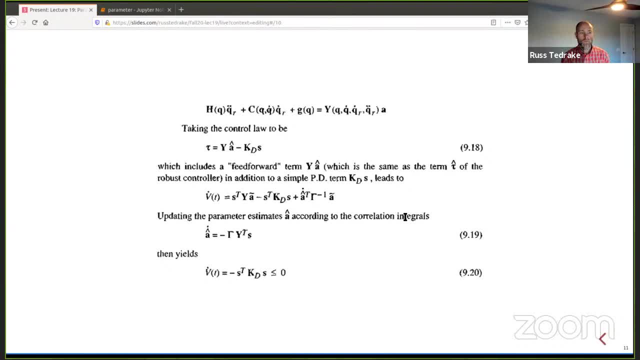 residual. But the only reason I think to use the physics-based models is if you can train it faster or it generalizes better, Because I think the representational power of a deep network would be sufficient without it. Oh, that's what I was wondering.